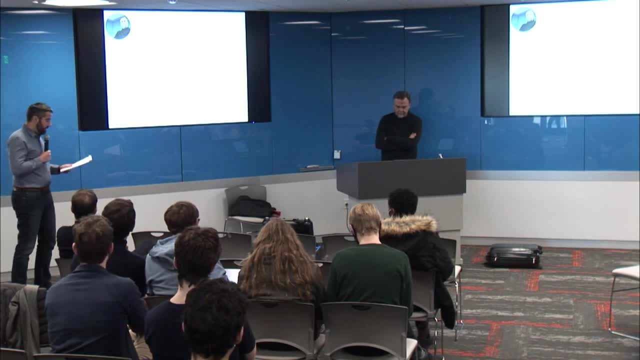 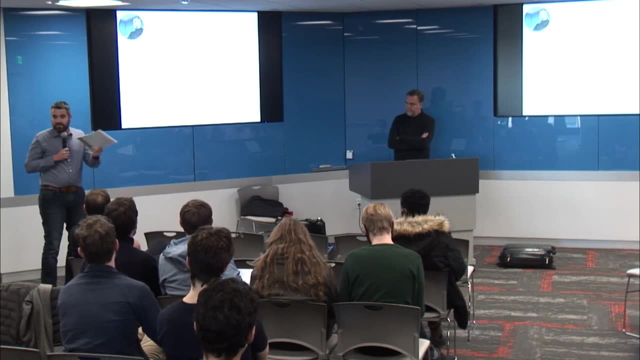 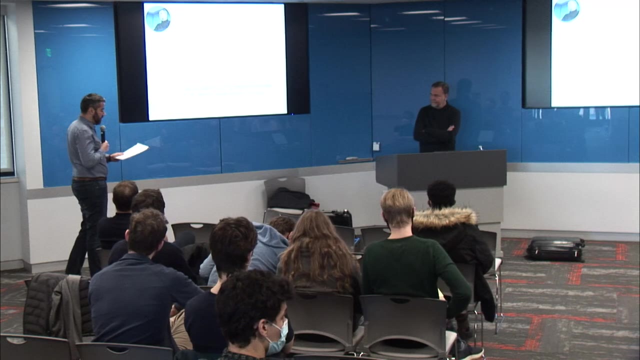 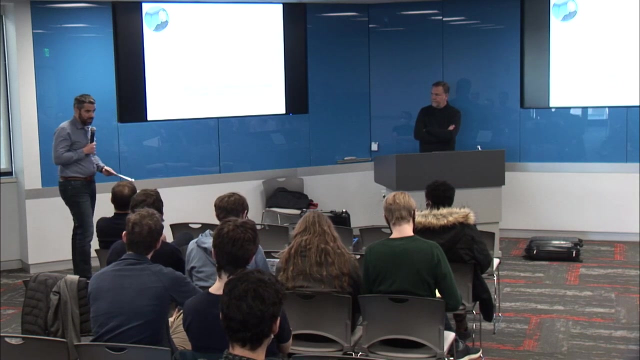 graph-based estimation framework for sensor fusion. It's a library that has been widely distributed, widely used by many people, many of us in this room, to solve complex estimation problems like SLAM or structure from motion. Frank has also worked to transfer some of that technology to industry at Google and before that at Facebook. 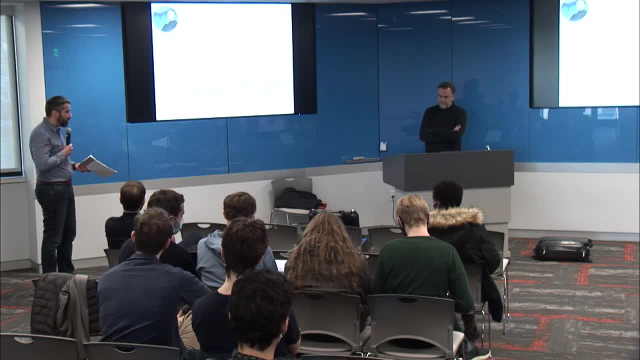 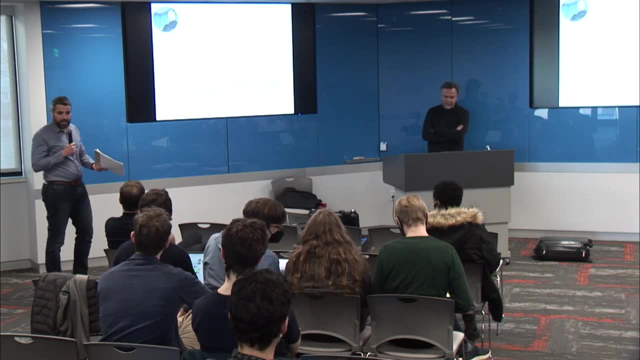 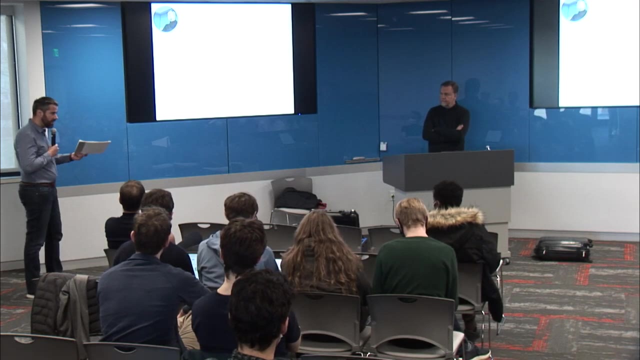 Reality Labs and maybe most influential, I would say. Frank is a chief scientist at Skydio, where it's a company that sort of was founded by. it's a drone company founded by MIT people, MIT students that I heard sometime this year. 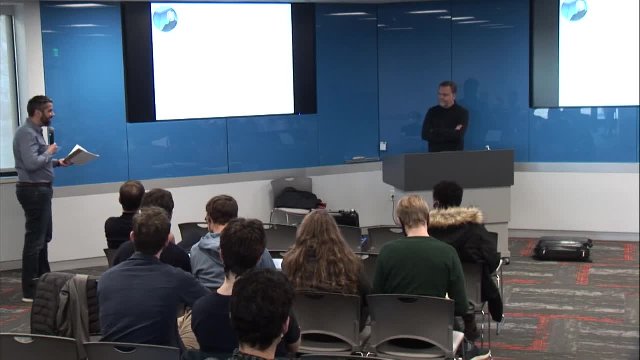 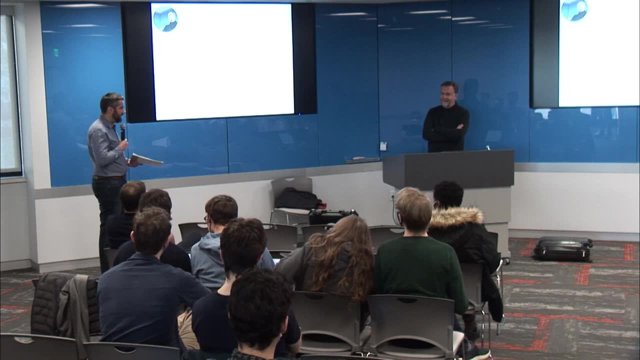 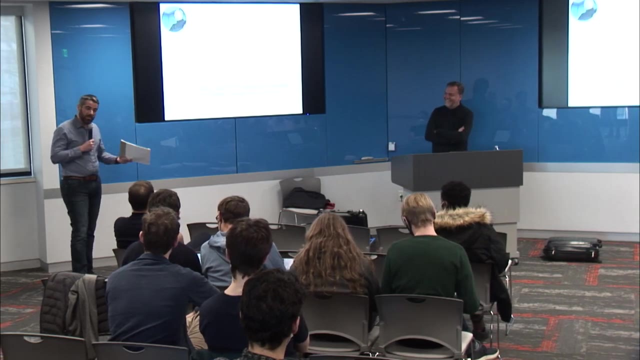 that became a unicorn. So I guess, well done. I don't know if are you going to pay a round for everyone here later. There's free cookies There you go. Anyway, well done, Thank you done really well done, very influential both academically and in industry. So 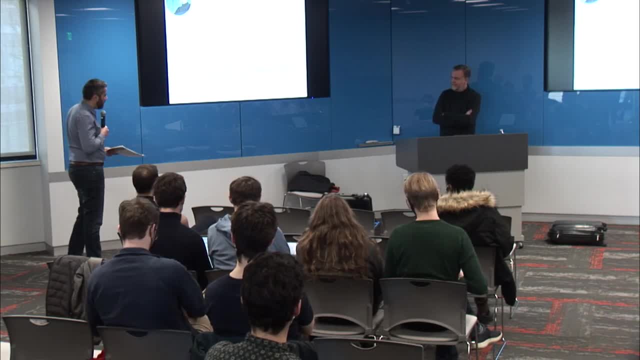 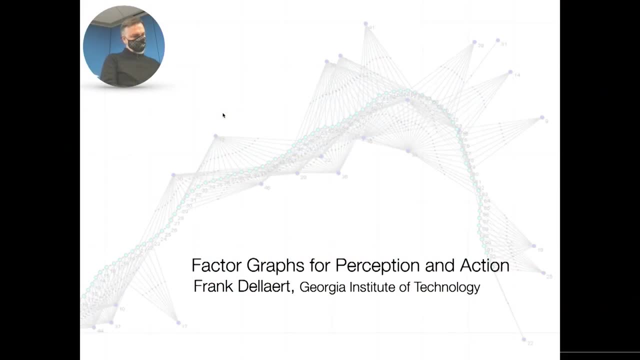 it's an honor to have you here, Frank. thanks for coming. We're all eager to hear more about factor graphs for perception and action. Thank you, Alright. thank you for having me. this is great. Yeah, I've been doing factor graphs. 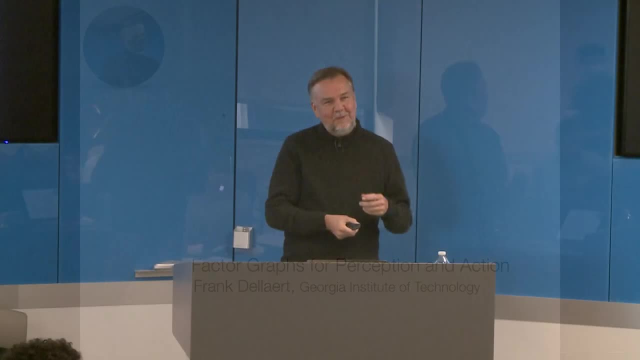 for quite a while, and Luca actually worked with me to make a lot of that possible. In fact, I could probably not have done any of the work at Skydio without Luca, you know, having visited my lab and done a lot of work. so, And of 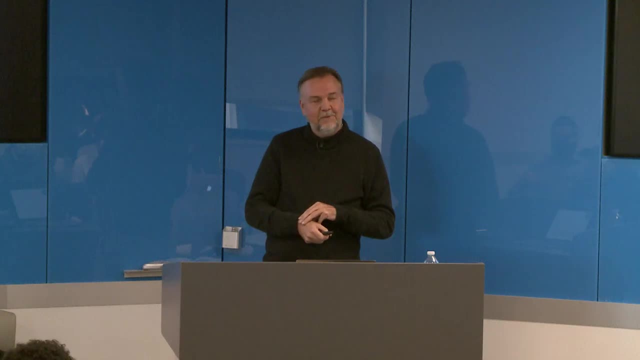 course, Michael Case, who was a postdoc in John's lab for a while now, is at CMU for quite a while already. So there is a deep MIT connection with all this work and I'm very honored and pleased to see that many of you are in. 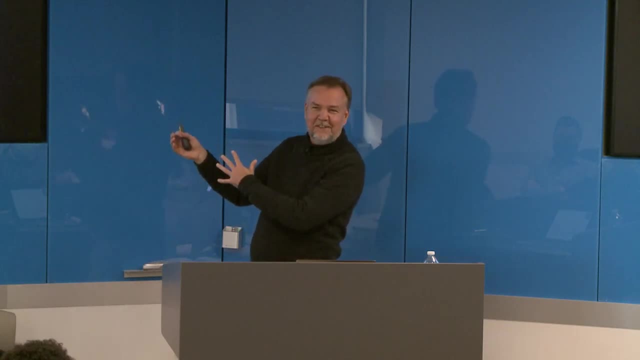 fact using GTSAM, and if you're not yet, I'm going to try and convince you that at least- maybe not GTSAM, but at least factor graphs are worth your attention. So thank you for your time in thinking about it. A lot of that work has been. 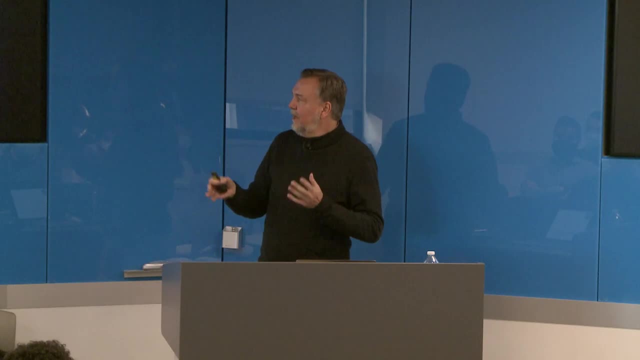 focused on perception and but after I came back from from industry, I really wanted to, I guess, really impact the world by action. So I thought about how can I use factor graphs, how can we use factor graphs to do action? and some of this work already started even before I left, But so let's talk about that. So 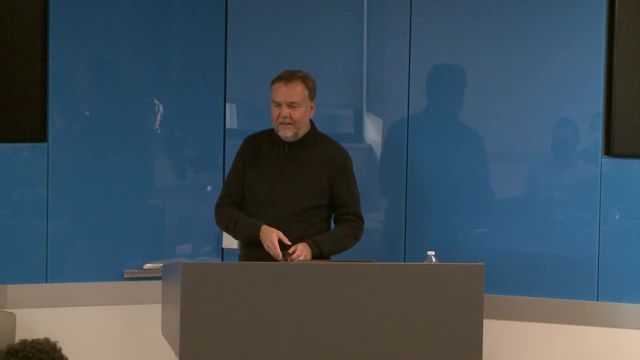 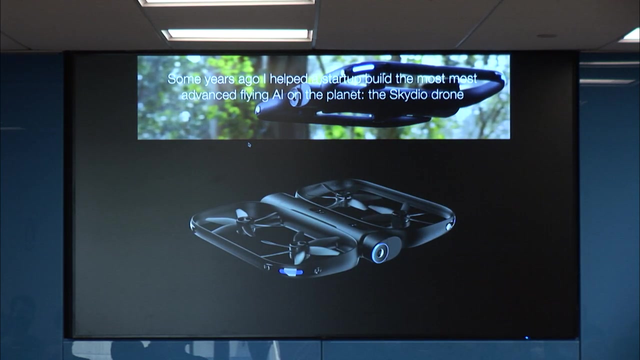 some years ago I did help as a as a chief scientist to to start Skydio. It was very interesting. Adam and Abe, the CEO and the CTO respectively, are actually were students of Nick Roy. Nick Roy was in my lab, my, you know. 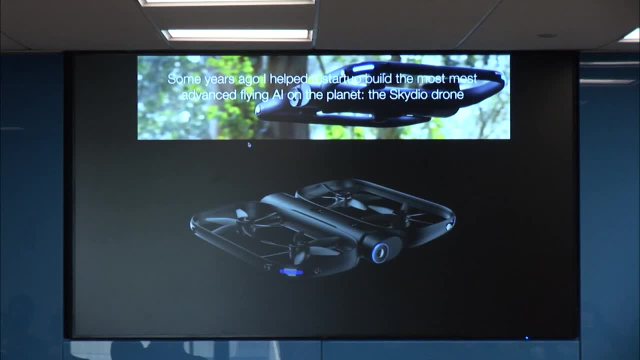 fellow grad student at CMU, So they were my academic nephews, but then I, now I- reported to them. So that was an interesting switch right, And they enlisted the help of their friend Matt to become their CXO. Do you know what CXO means? It's a chief experience officer. So the idea is: 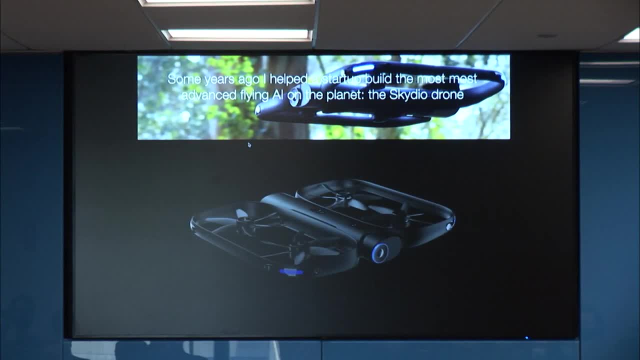 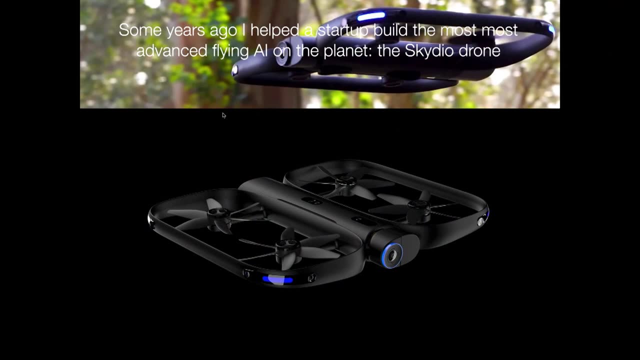 you know, the customer is central. We need to create a cool experience for the user of, in this particular case, this drone, which is the first commercial product from Skydio. It's a drone- and this is the first instantiation- And it's it's. it looks like a regular drone with a pan-tilt camera in front, but 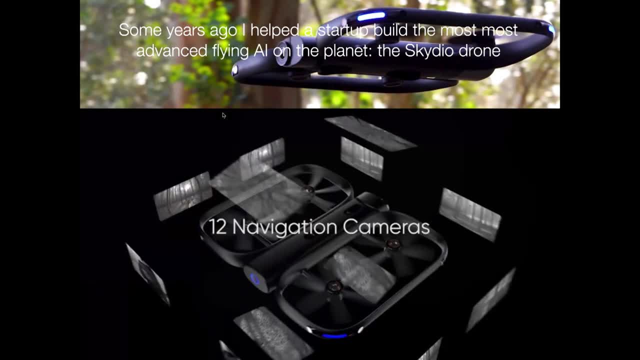 the secret weapon here is that it has this: this drone has 12 navigation cameras arranged in six stereo pairs. okay, And that will enable enable it to to function fully autonomously in in densely, in dense, obstacle environments. So so that's. that's pretty cool. 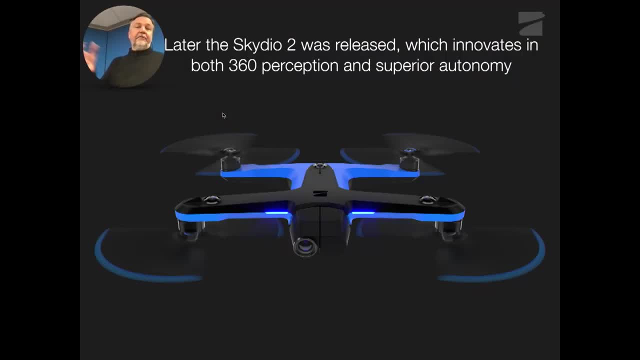 And then later they, they, after I left the company, they, they built a second version of this drone And and look how it has a drone, This is the Skydio 2. And you see, it's quite small but it has a larger battery life than the first one. And 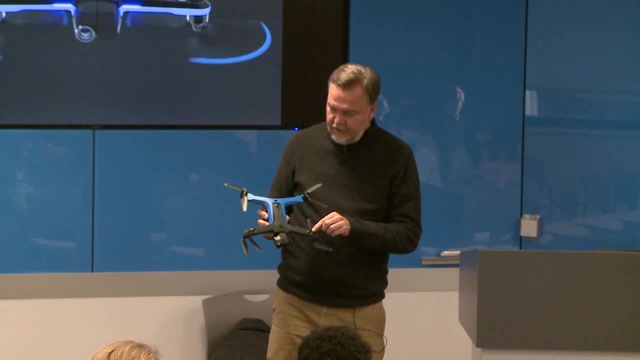 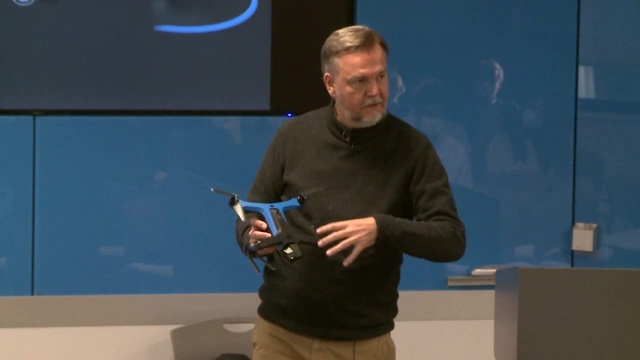 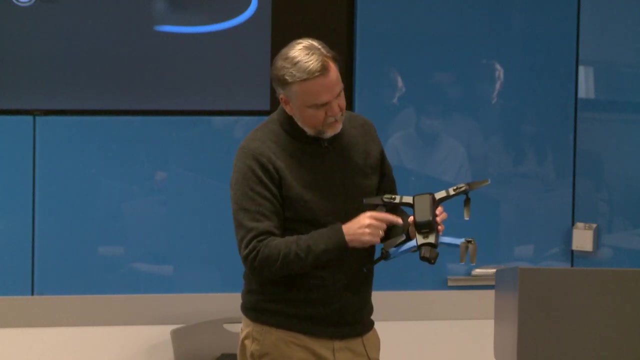 it doesn't have 12 cameras, but it has three very wide field of view cameras here on the top. It has a twin-tri-nuclea stereo rig that gives you vision on the entire top hemisphere, And then they have the same at the bottom, Sort of it's not exactly the. 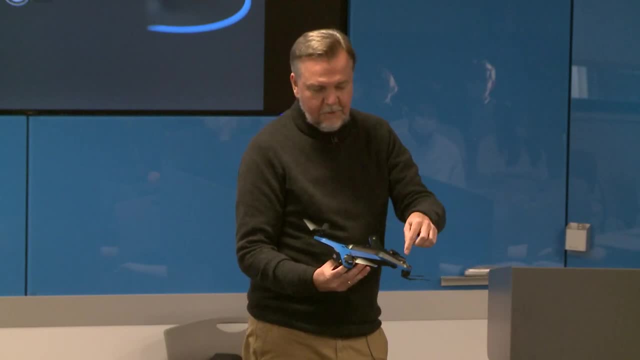 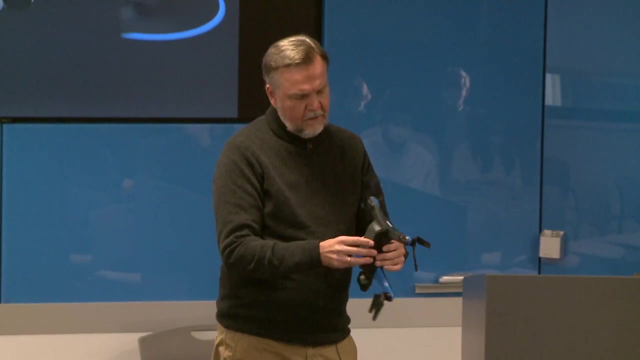 same so so the camera's actually sit on the other arm, all right, So you need to actually stream high-resolution video. All of these cameras are 4K. Grayscale have to be streamed to sort of an in talking to the TX2 or TK2. that's in there and then your 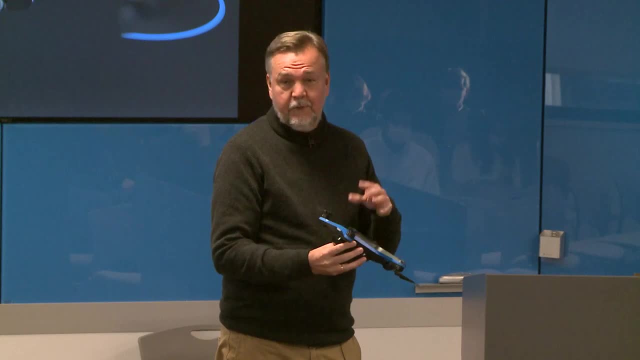 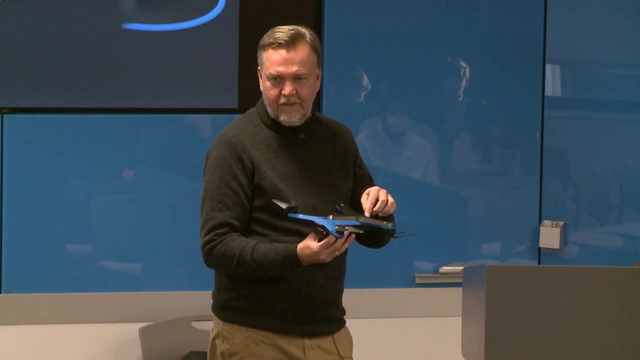 And actually doing that is complex. One of the biggest problems we had, even with the first prototype, is these high bandwidth transmission cables from the cameras to the processors. in the process of fabrication They got pinched, So hardware is really hard If you're thinking of a startup. 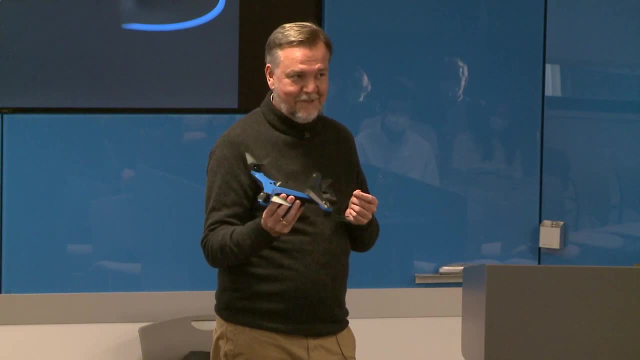 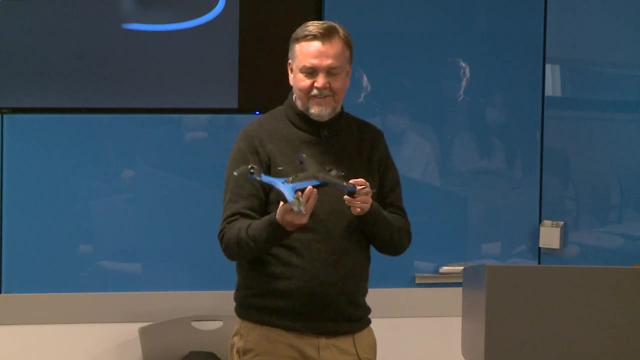 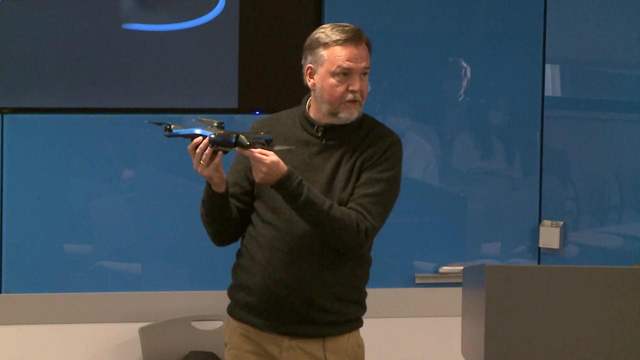 software startups are so much easier than hardware startups. Luckily I was on the software side of this company so I didn't have to deal with most of it. But this then has a pan tilt on the front which is a 4K, 60 frames per second, color camera. 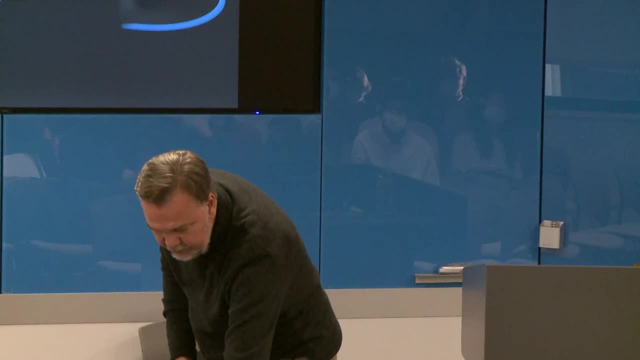 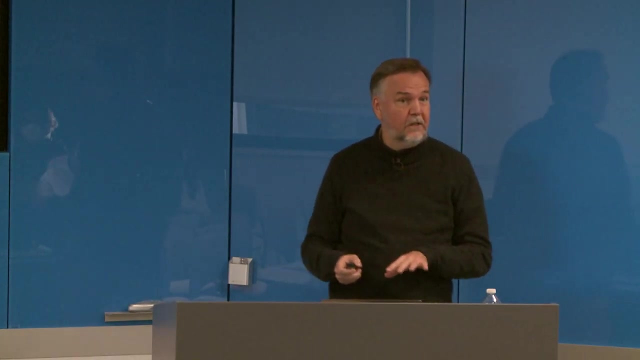 So it's really an awesome piece of technology. Part of it is the hardware that makes it great- It's small, it's omnidirectional- but part of what makes it great is the software that's running on it, And the software is basically what we all do. 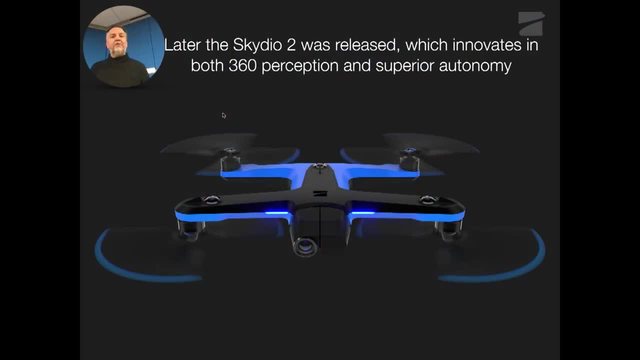 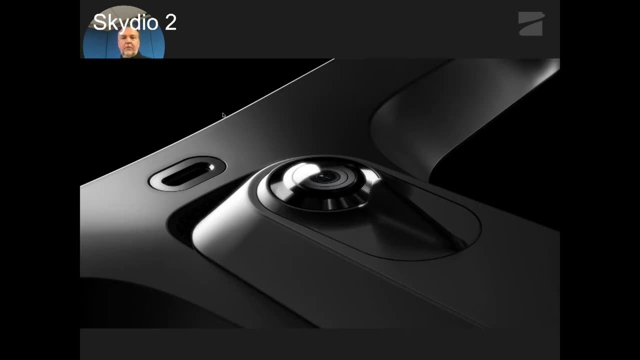 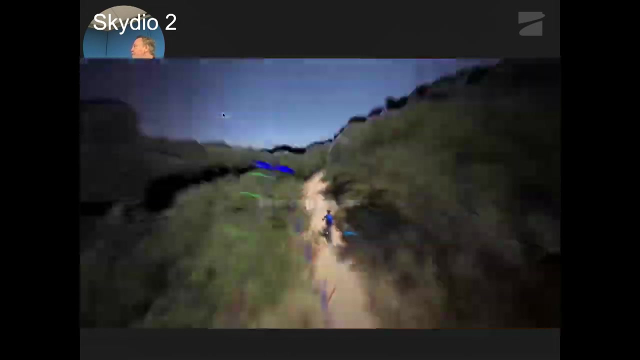 which is which is SLAM and inference and estimation. So let me talk a little bit about that. There is a cool marketing video that they made for the Skydio 2. Most of the footage that you see. so this is the internal representation. 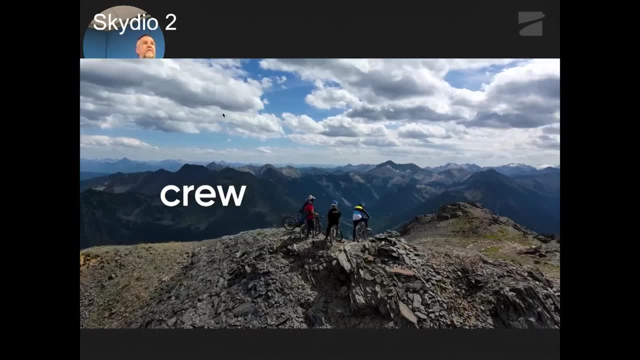 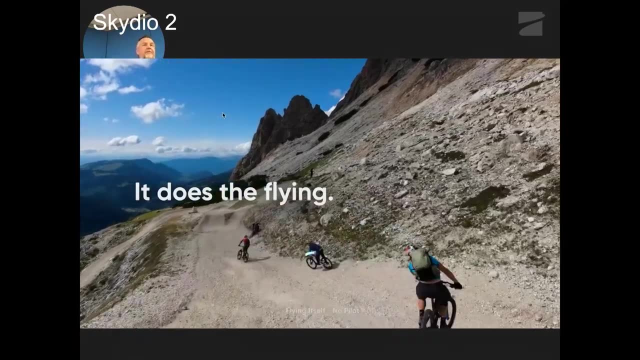 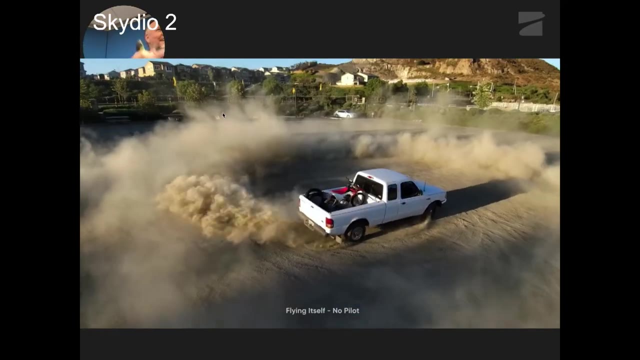 most of the footage you will see is actually shot by the drone itself, And the use case here is following people as they do cool stuff. I know you're all grad students in Cole, Boston, but in California you mountain bike down the mountains. 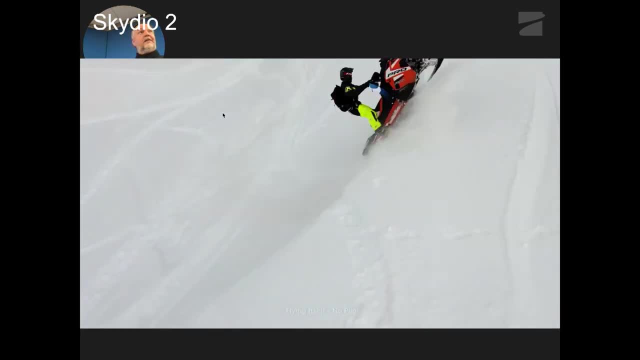 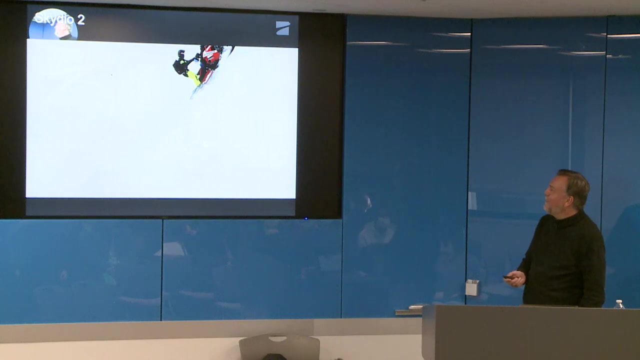 and go windsurfing, And last week I was in California. I went to LA, where my son has a PhD, and to San Diego. It was 80 degrees. We were on the beach, Sorry. So what do you do? 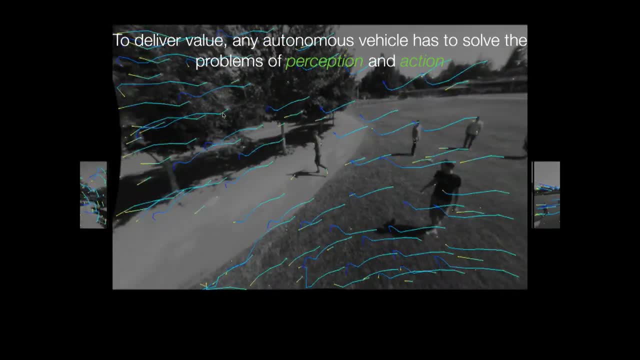 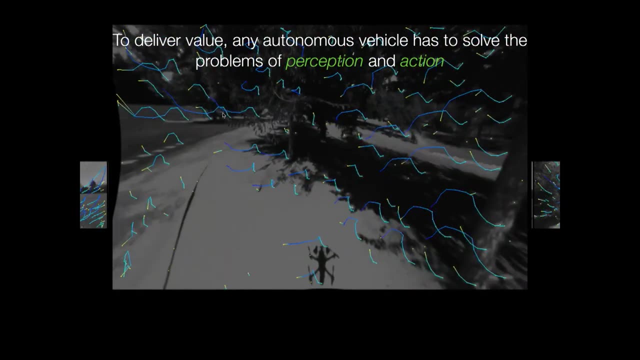 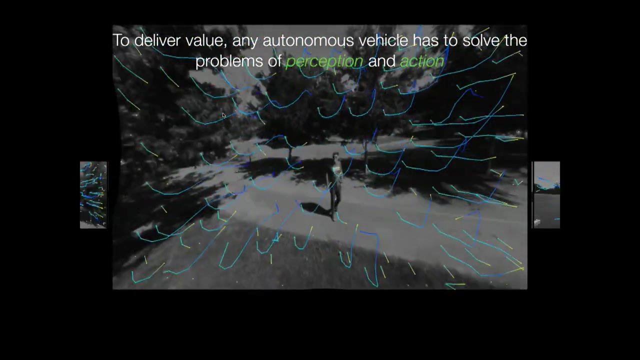 How do you make this thing fly autonomously? The pipeline is actually quite classical, So you extract features. These features you can track through frames And because you're tracking them in 12 cameras or six, which have a 360 field of view. 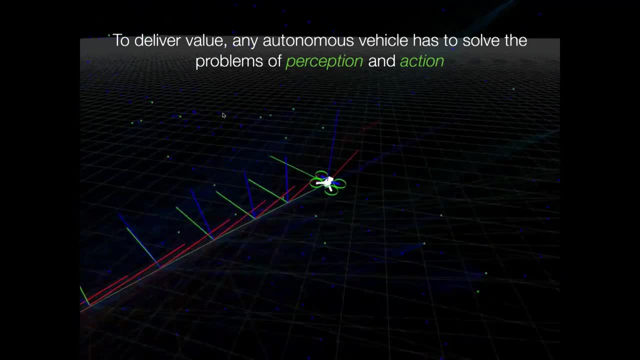 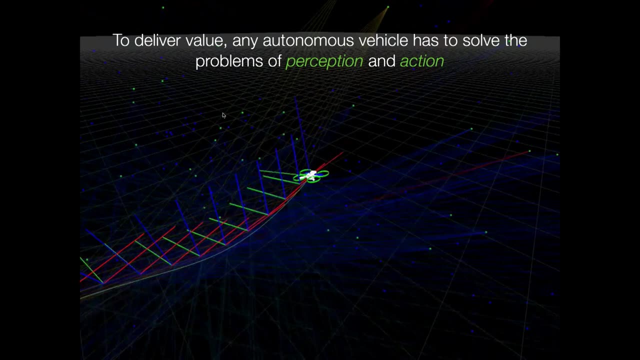 that turns out to be quite important. It's actually hard to do SLAM with a single forward-looking camera. Okay, there is a lot of ambiguities. You can't, you know, disambiguate, You can't do a translation from rotation easily. 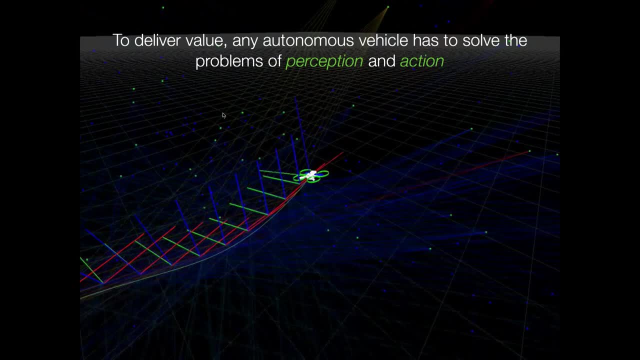 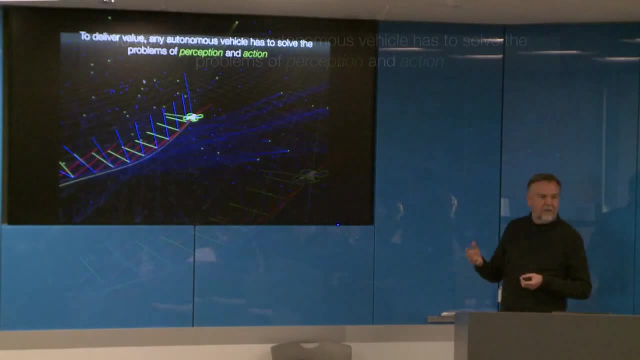 But with 360 field of view it becomes much, much more well-defined. So, and then you can build a sparse SLAM solution, And this is what I helped them build. It went from single camera to multi-camera- A sparse, real-time SLAM solution that provides this ironclad geometry. 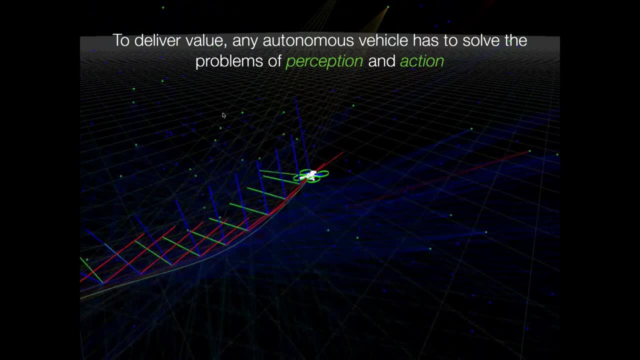 on which you can then do dense stereo, And dense stereo gives you obstacle avoidance and all the nice things Right, And factor graphs and GT-SAM are- were central and are central in solving this. So it solves the SLAM, but it actually also solves the action. 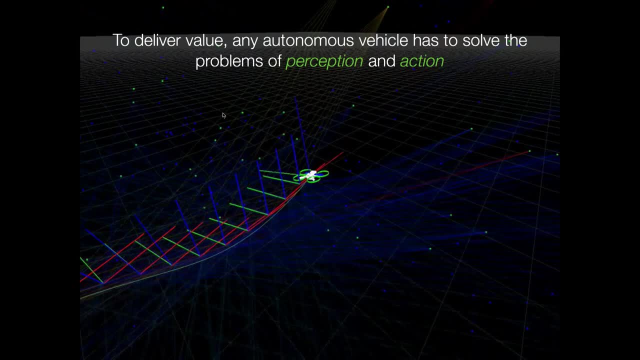 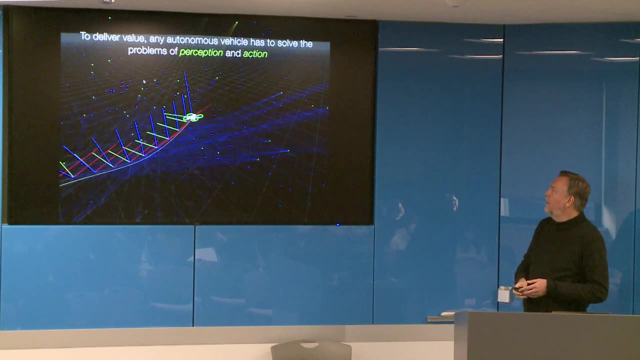 So how do you plan the trajectory? So at Skydio we- I was also involved in sort of the motion planning, And there we use factor graphs for motion planning. So so none of this was sort of possible without the reason why they called me is. 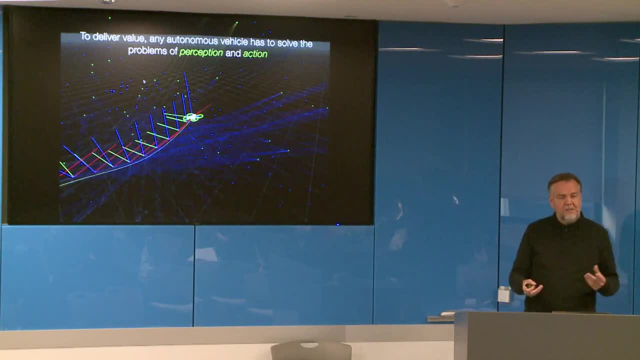 hey, you know we saw that you use GT-SAM, that you create the GT-SAM with your students. Do you want to be an advisor to the company or join? And then I joined for a while And that was that was really, really an amazing time. 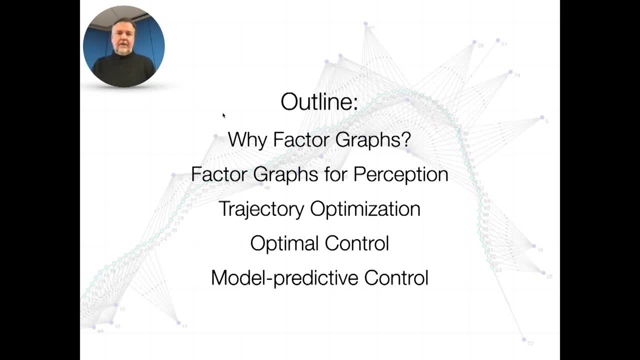 So so let me tell you a little bit about about factor graphs And why you would want to think about them. I will then sort of recap some successes, Many of them by by Michael and and Luca, on using factor graphs for perception and estimation. 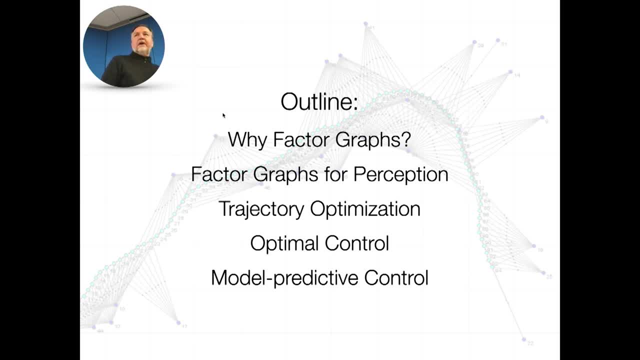 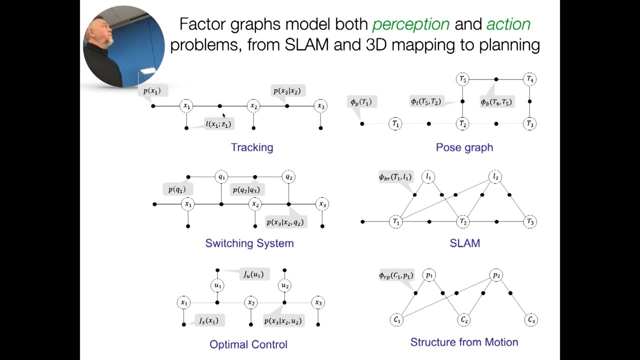 But then the rest of the talk I will spend on factor graphs for action. How? how can we use the same representation to plan and act in the world? Okay, All right. so factor graphs model both perception and action problems in a in a very nice way. 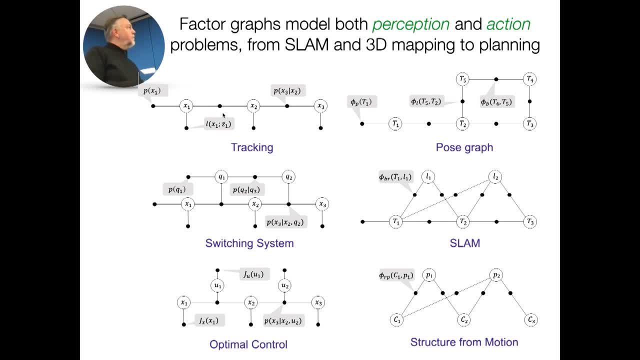 So. so here are a couple of examples. Interestingly, the, the laser pointer doesn't actually do anything on the screen, it seems. Maybe it does on that one. No, There we go. So so in the in the top right I can move my mouse here. 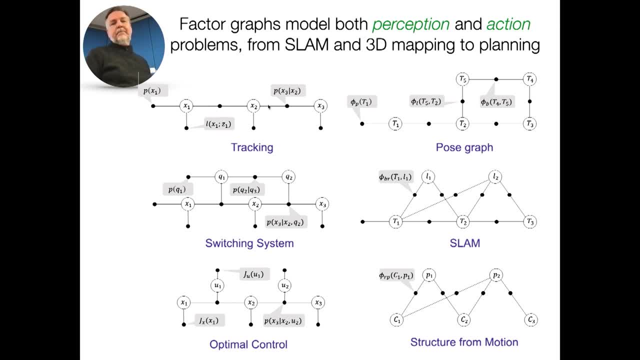 So you'll see that you have a a tracking problem. So here the tracking problem could be: you're tracking a person from the, from the camera. These are not abstract things. I'm talking about real things now. Okay. 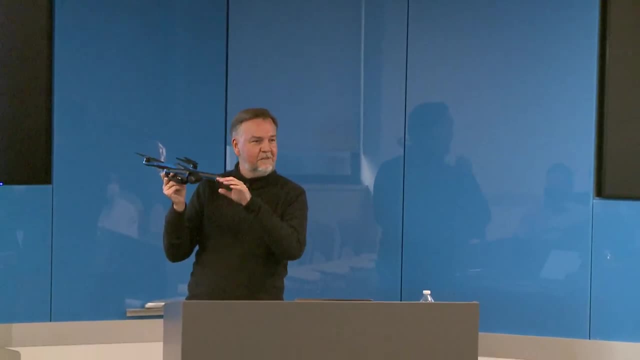 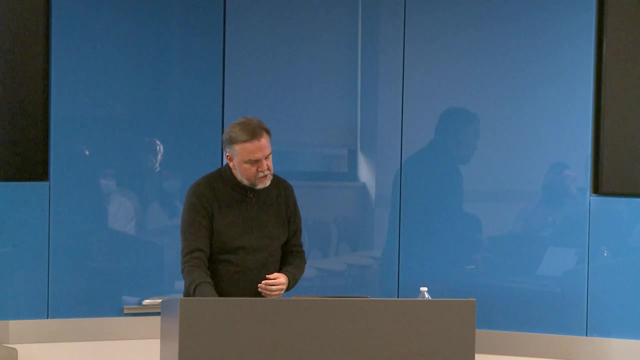 So you have a, a camera. The camera, by definition, is pointed at your customer And you want to try and track that person over time from from observations. Okay, So so what you want to know is the unknown variable is: is what is the location of the? 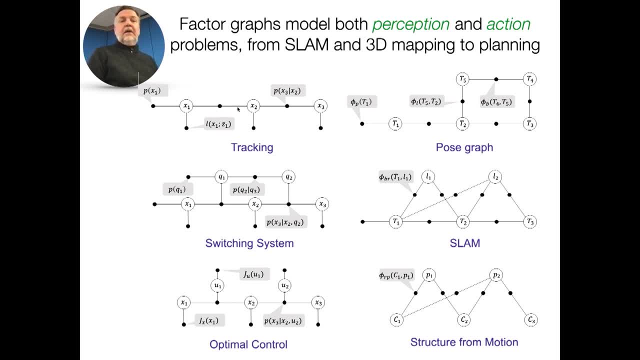 person at time one, at time two, at time three, You also have a motion model of the person. So there's, there's a factor which, which is a probabilistic relationship between between X1 and X2.. It says: 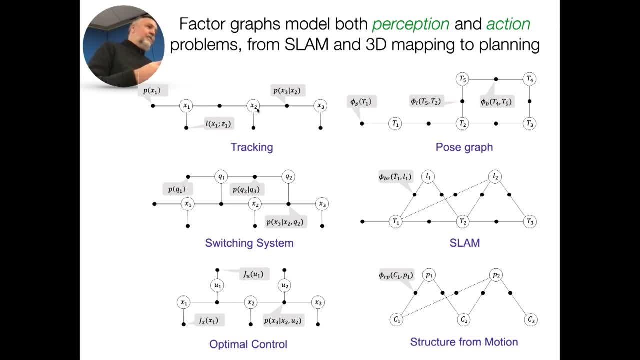 So it was at time one, that was, I was here, Then at time two- I'm probably close. Okay, So that's a probability distribution on the joint space of X1 and X2.. You also maybe have a prior as to where the person started out. 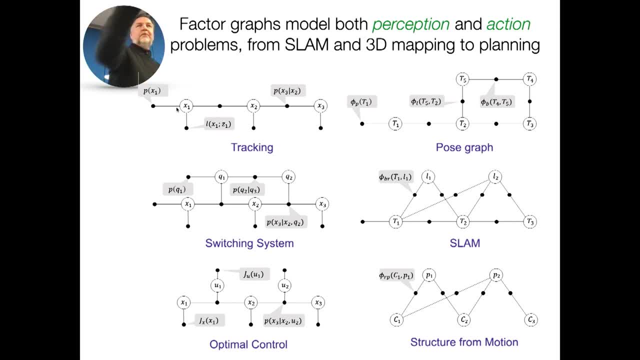 Okay, Maybe the person started out at the origin and then you, you track the person And then you have these unary factors that encodes the relationship between the measurement, which is which is given. So there is no unknown variable for the measurement, because it's not unknown. 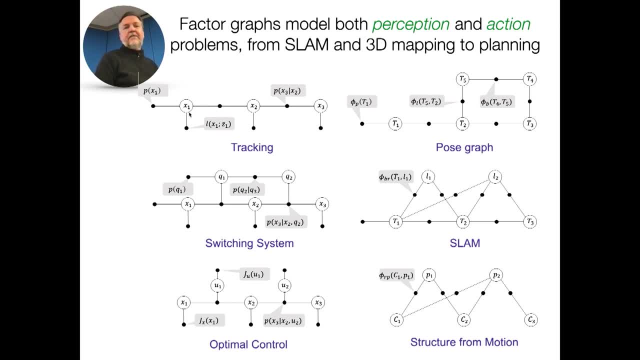 It's known. So you have a just a factor, that is, a probability distribution on X1 derived from the measurements, which could be, could be anything Right And in, in, in. in the Skydio case it was you know, detect the person, relocalize it. 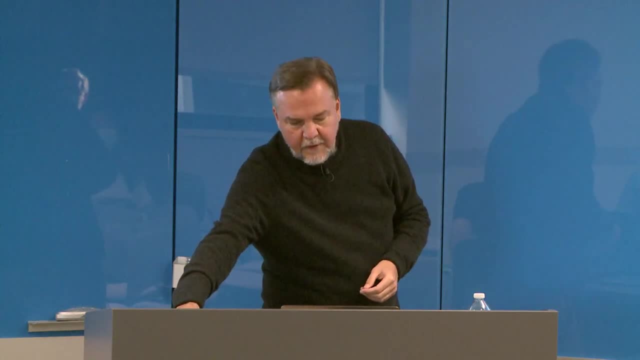 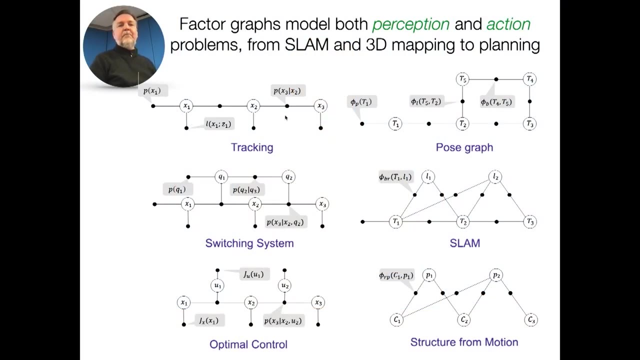 and then you have a 2D observation image and you try to track the person in 3D. So in this case the variables here are three-dimensional, The measurements are two-dimensional And you have a motion model, Say constant velocity or or something. 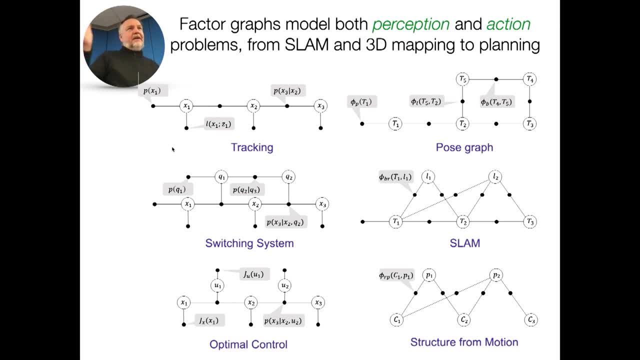 But people are arbitrary and and and difficult, And, and so you know they have their own minds, you know, So can we? can we actually estimate what's in their minds? Okay, So now, now we're going into hybrid inference. 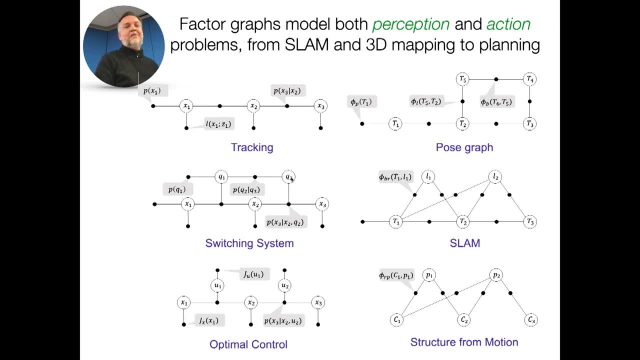 Okay, So we can add a sequence of discrete variables at the top with with its own Markov chain. This is now a discrete Markov chain. Okay, That influences what the person does, So maybe the person is. okay, I'm running along. 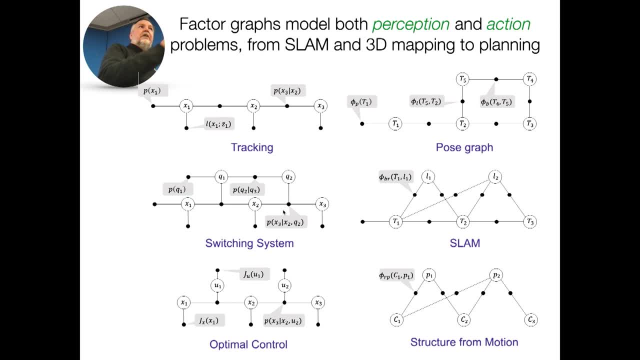 So the the discrete states is is running along, running along, going straight. But then you take a. you know you're going to do a left turn, so that you know the person is not thinking about going left. 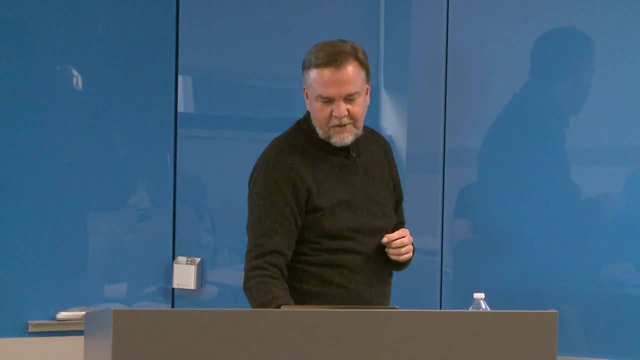 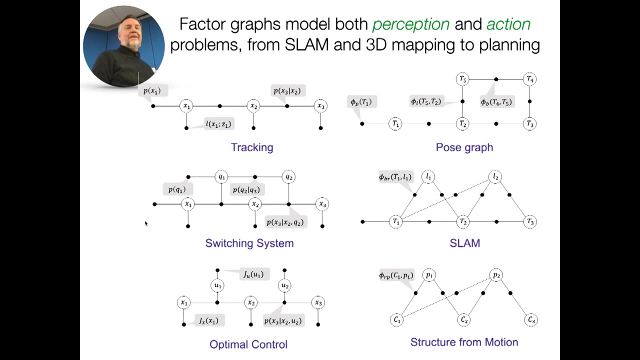 So that's a whole different motion model. So you see that the, the discrete states, influences the motion model, And so this is estimation in a switching system. Right, You can also do optimal control with factorization, And so this is the the second half of the part of of the talk. 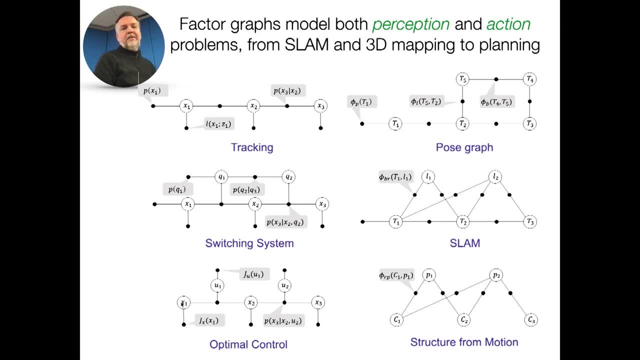 So, so now the, the states are: what is your trajectory that you want to effectuate in the future, And how do you effectuate? how do you create a trajectory? Well, you do it by a sequence of controls, And the controls tell you what the you know, allow you to influence the, the dynamical, 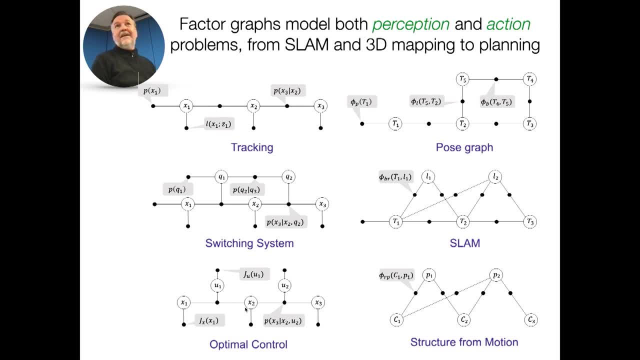 system between successive states in time, And so the optimal control problem is Find the trajectory and the controls together, That's that's called collocated optimal control, in a way Right So to satisfy an objective. And how do you specify objectives? 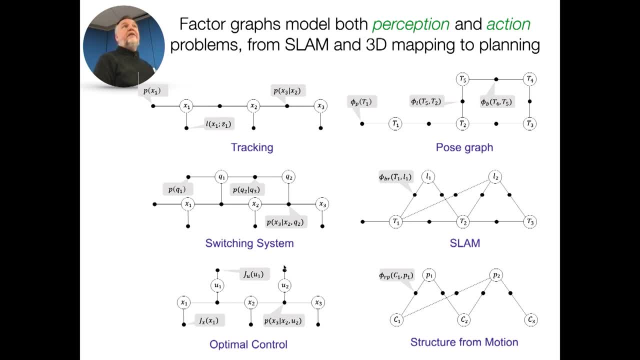 Well, you specify objectives by adding factors that are now costs that you want to, costs that you want to minimize or rewards that you want to maximize. And then there is some more complicated graphs here, But you know, these are SLAM pose graphs for SLAM. 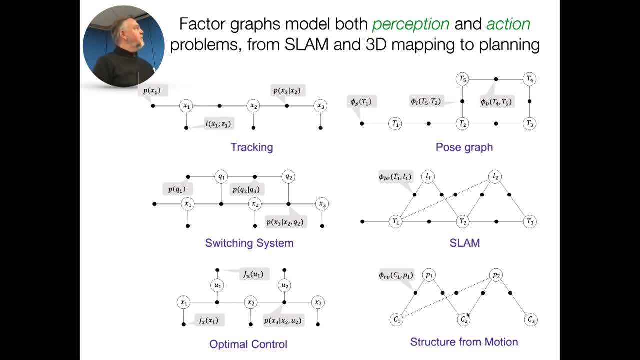 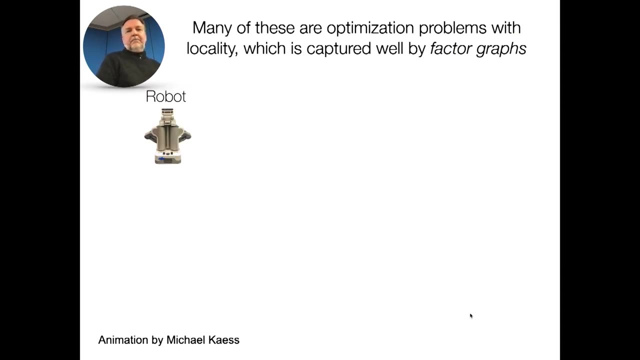 SLAM with landmarks and a structure for motion, which is a computer vision SLAM right version. So I'll talk about them in a little bit more detail. So many of these are just optimization problems. You know, typically you find one solution which is the maximum probable solution, or 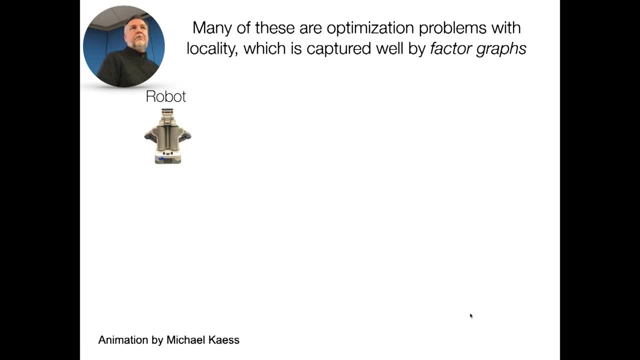 one of the modes of your probability distribution And you could get in the wrong order. Right, You could get in the wrong mode. But- and that's exactly the sort of the cutting edge of research where John and his students are doing a lot of thinking about multimodal problems and Michael at CMU is doing that- 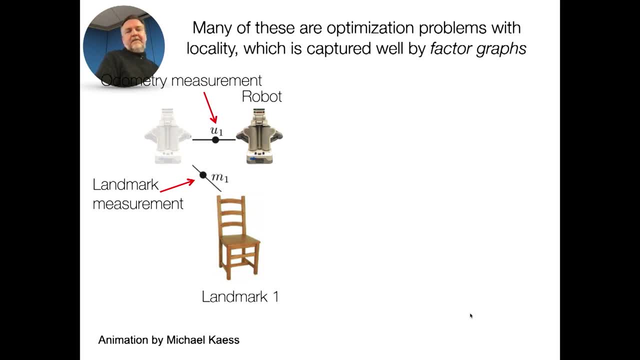 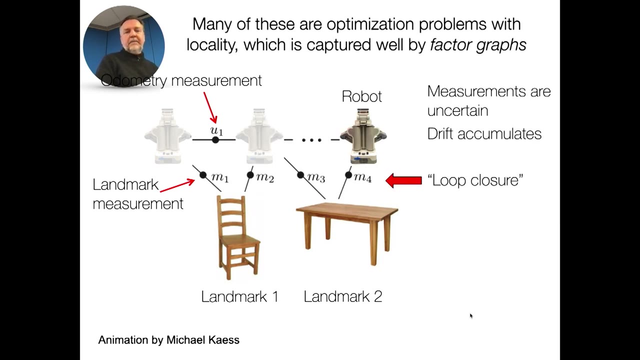 as well. But you build this factor graph. You can build it on the fly as your robot is moving and it finds landmarks, and you add factors for measurements, variables for landmarks, and then you have loop closures, et cetera. This is a slide by Michael. 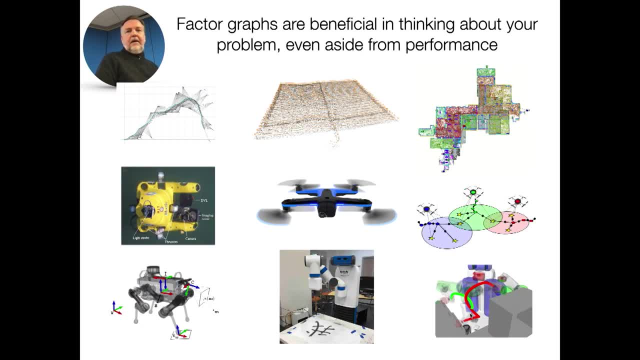 And so I'm going to argue. maybe I'll try to give you evidence, But part of the evidence is just my experience. I have experienced at Georgia Tech and all these companies, that factor graphs are just an amazing thing to write on blackboards Or whiteboards. 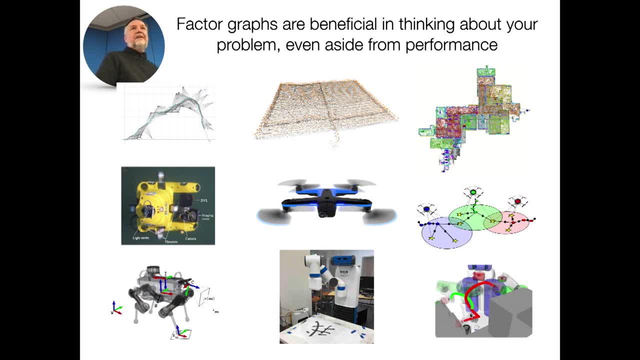 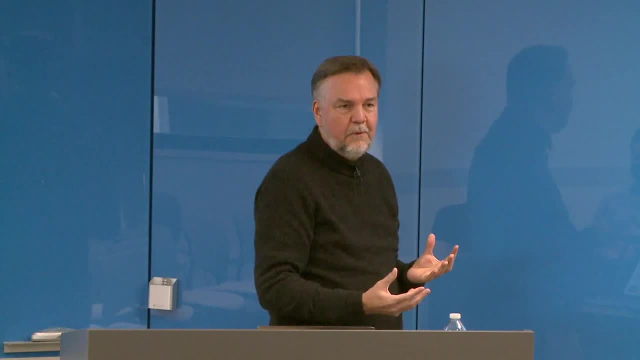 Okay, It ties together all these problems. It allows you to sketch out: okay, this is our problem, These are the constraints, These are the things that are connected to this. This gives you the structure of the problem, And so it allows you to talk about it. ties together different engineering teams. 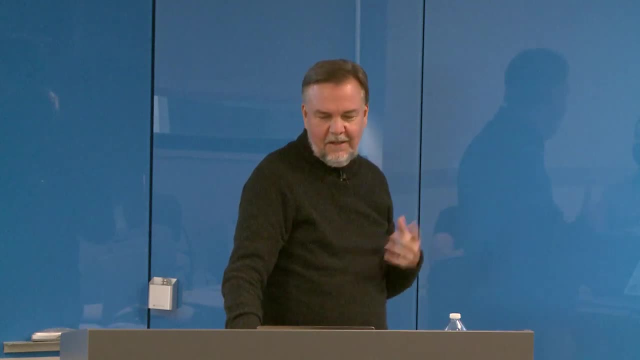 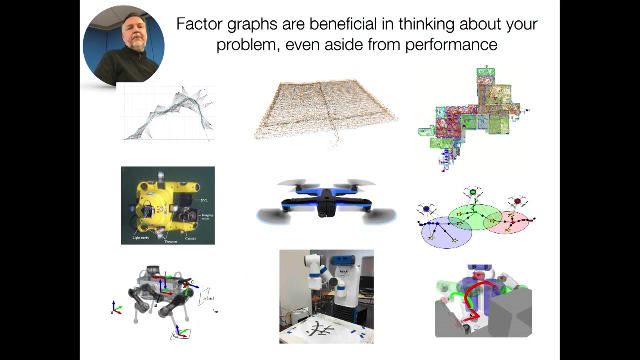 You know so the action team and the perception team, And so it gives you a common language to talk about all these things. So, just aside from, even from aside from, performance factor graphs are worth your time, All right, and so I'll give some examples for for perception. 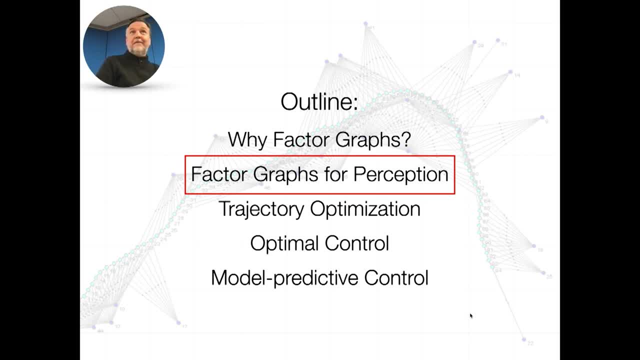 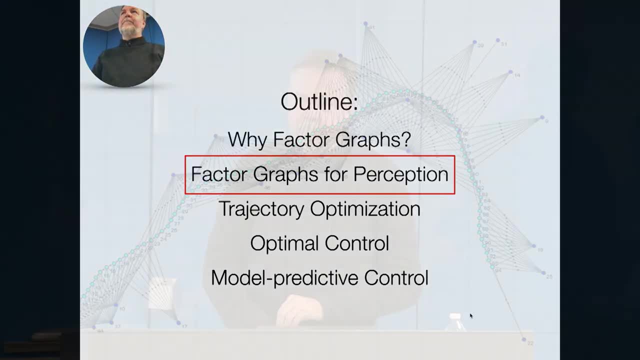 And, by the way, I can make this quite interactive. So if you have any questions, there is a question there. I'm sorry. Is there a difference between just a general graphical model from statistics and a factor graph? Is it No? 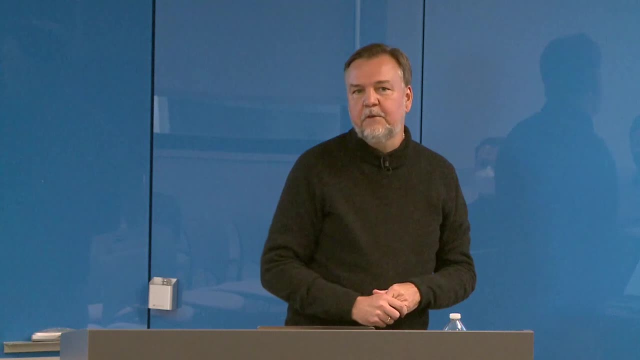 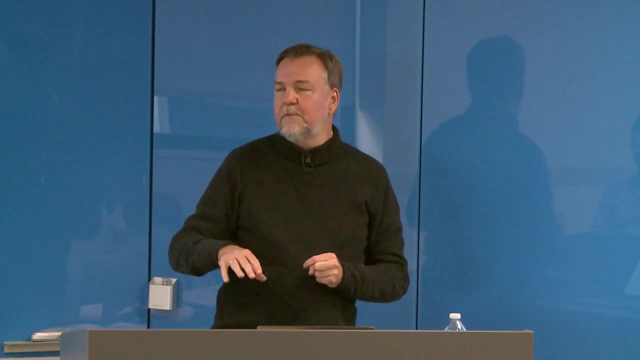 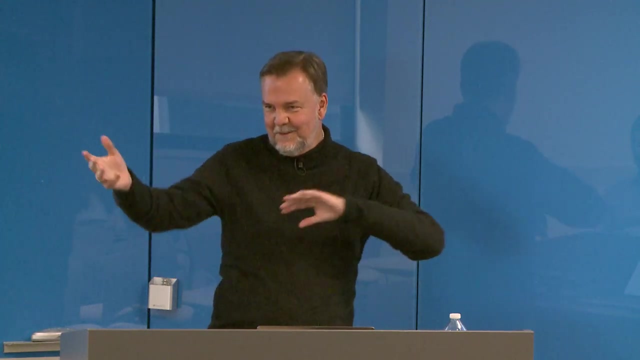 A factor graph is a form of a graphical model, So the most commonly known graphical models are base nets, Which can be trivially converted into factor graphs. So so, and typically you always want to do. In fact, Kevin Murphy, who wrote the book on you, know probabilistic estimation and 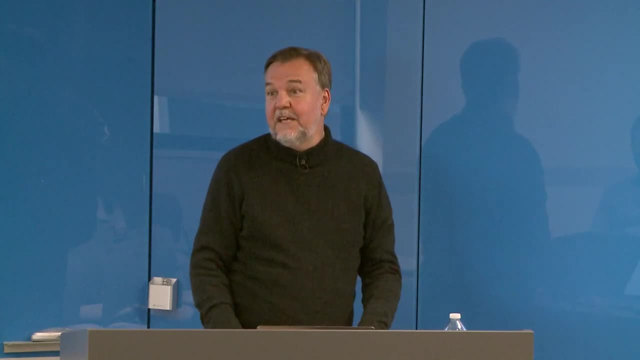 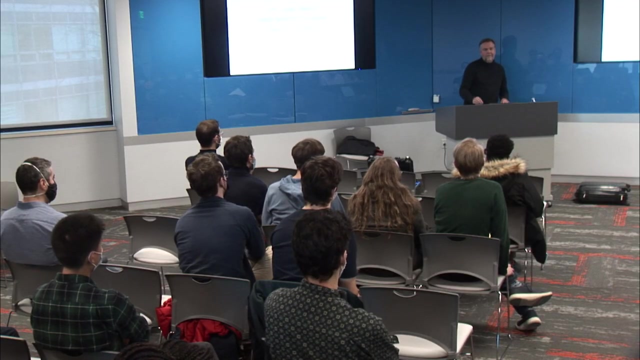 HMMs and all these things. he has a base net inference library And the first thing he does under the hood is convert it to a factor graph, then do inference Right. The other well-known graphical model is, is, is is Markov networks. 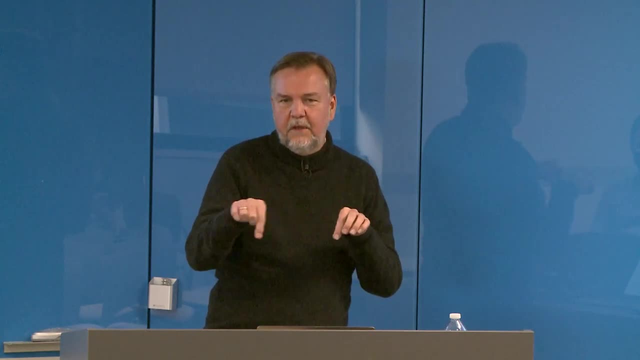 Right Where you have not. You don't have, You just have undirected edges, that sort of encode, the Markov blankets. But I will argue that anytime you have a Markov network it's better to to talk about the factor graph. 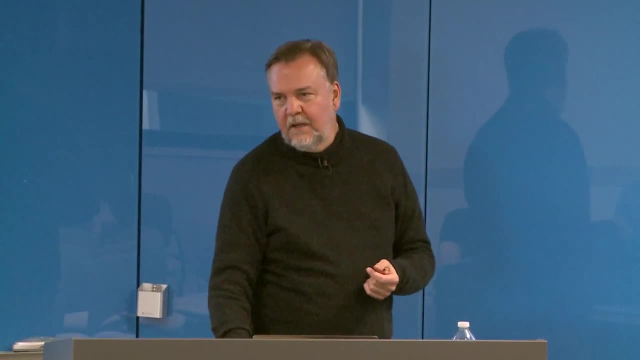 Which can bring finer structure out. So it's one of the array of graphical models from statistics you can use. That's a great question, Would you say. the key benefit is making explicit conditional independence relationships to exclude, To exploit the sort of problem structure, things like sparsity and in terms of factor. 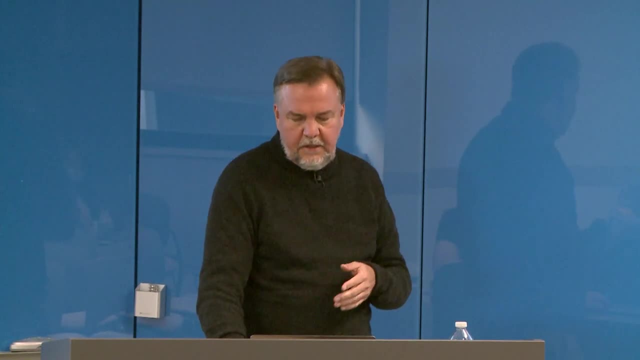 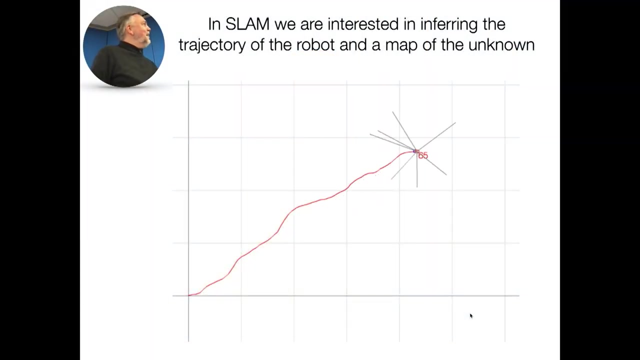 graphs versus more general graphical models? Yeah, absolutely. Let me give you an example here. So the example is the one that I've been showing since RSS 2005 at MIT Okay, Which I think was the first RSS, And, and back then my, my daughter was like five and now she's 22.. 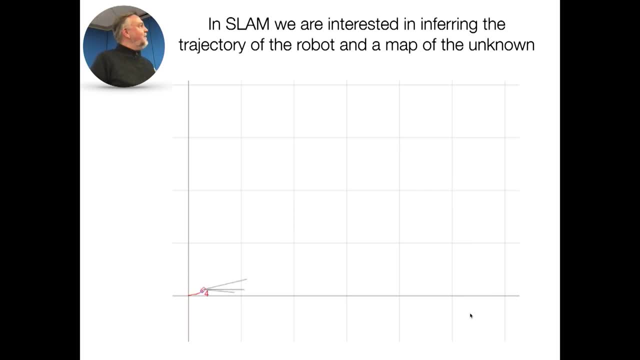 So The This is a little robot And and it's, It goes around and it, it, it samples the environment In, in this case it it takes bearing range measurements to trees. This is actually a truck driving in a park in in Sydney. 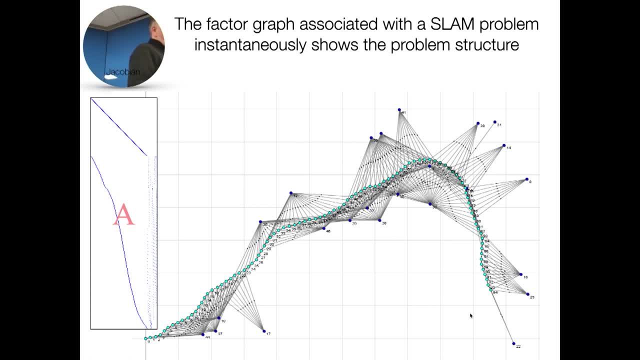 And this is then the factor graph, And it shows very well that that you know this. this landmark here is only connected to a subset of the of the truck positions, So it was only visible for a small amount of time. 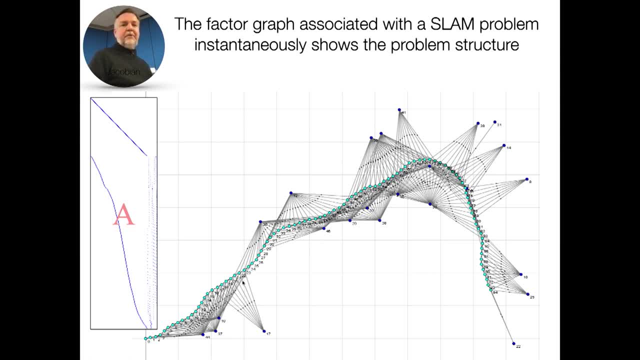 And so that induces sparsity. This, this thing, is not seen from the very first position. So the sparsity here is encoded in that bipartite graph. Okay, It's bipartite, because these little factors tell you the the nature of the probabilistic. 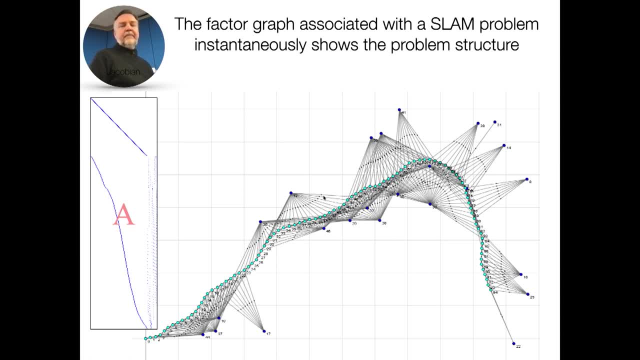 constraint between them Right And in fact, the sparsity and and and I said this in a in a meeting with with Leslie today. So so there is a deep connection between factor graphs and and and sparse linear algebra. 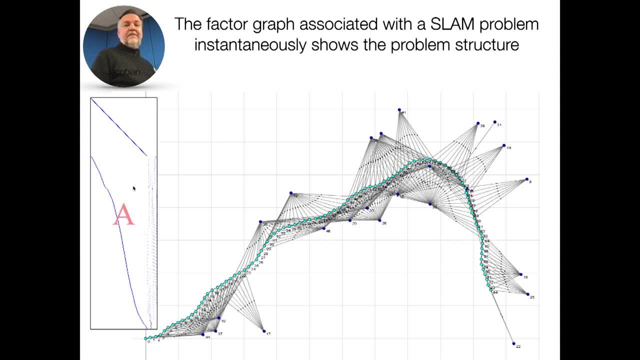 This graph is literally the connect, the, the connectivity graph of this square matrix, of this non-square matrix, Right. So for rectangular matrices, for for symmetric matrices, you can think about the sparsity as an undirected graph, But for rectangular matrices you have rows and you have columns. 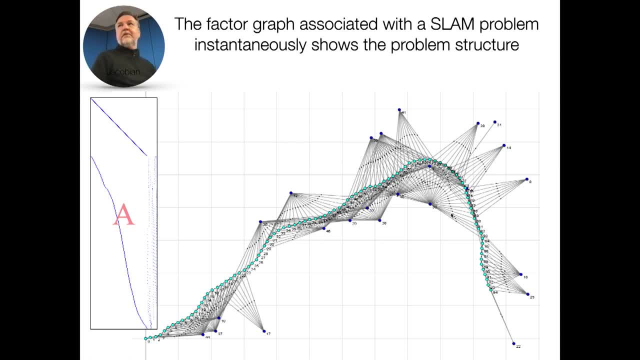 Well, the columns here are actually just the variables in this factor graph And the rows are the factors. So you can see that you know, for example, if you take, if you take, if you take the, the, the, the row of this sparse matrix, aligned with the, the bar in A, it has some connection. 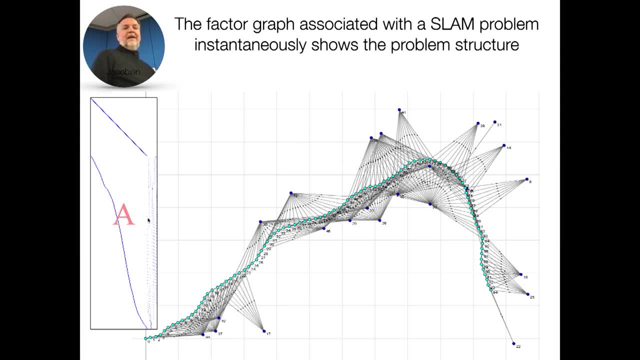 to some poles and it has some connection to some landmarks, Right, But? but looking at this graph tells me a lot. Looking at this matrix tells me nothing, Right? So so the factor graph is really the embodiment of the sparsity of of this linear algebra. 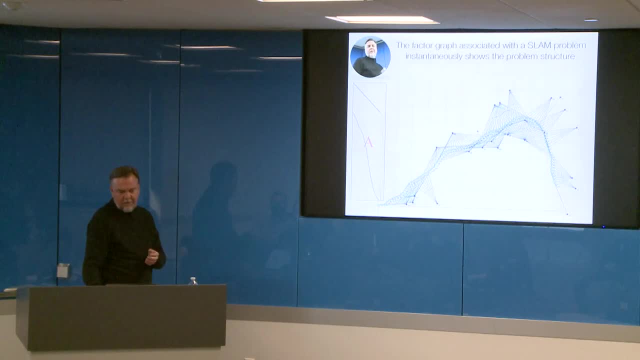 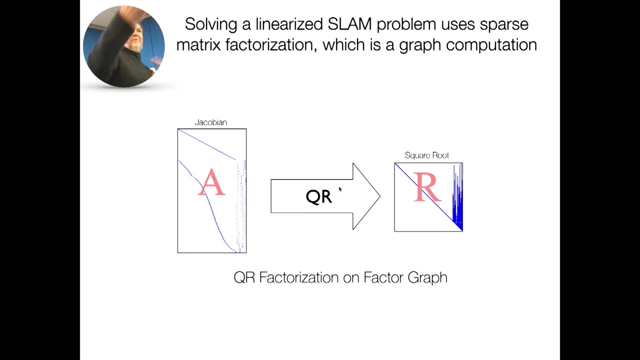 problem here. Why is it a linear algebra problem? Well, because the if you solve large-scale, least squares in a linear algebra problem, which is basically what you do in SLAM or structural motion or tracking. in the inner loop, you know you might have an outer non-linear loop. it linearizes and then creates a linear. 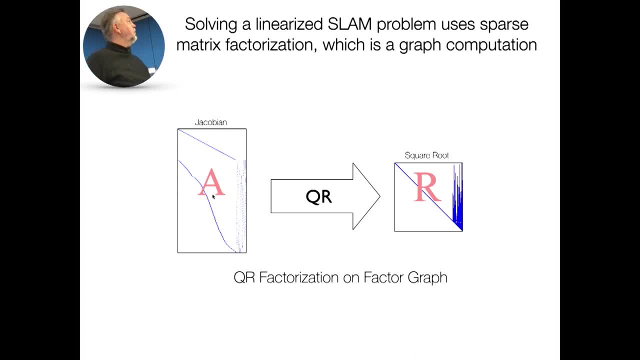 problem And then you solve that linear problem by by creating this sparse matrix. if you want to do that, We don't do that in GT-SAM. We just have the graph And then we do bucket elimination, Leslie, which is a linear problem. 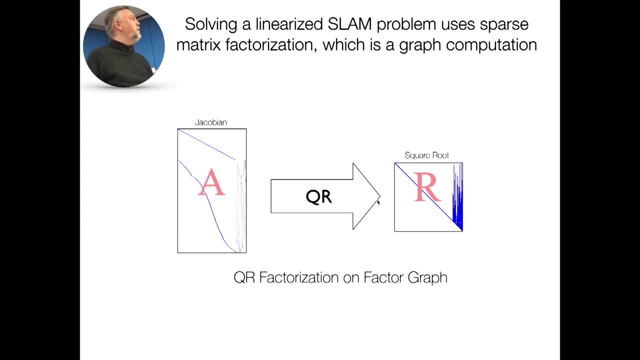 Leslie, which is also known in linear algebra as QR factorization, And then you get a factorized matrix which is basically the solution to the linear system. You now have a new estimate and then you linearize again, Okay, So, so that's interesting, because- but who knows here when I talk about bucket elimination? 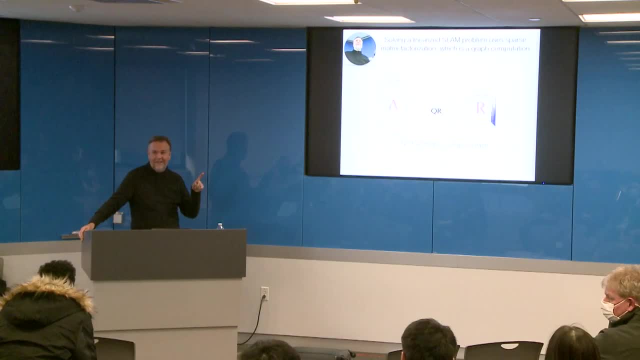 what I'm talking about. Raise your hand if you've ever heard the term bucket elimination. Okay, So, only four or five people. So I? I hear that Rena Dichter visited here, right, So so she she is a professor in UC Irvine. 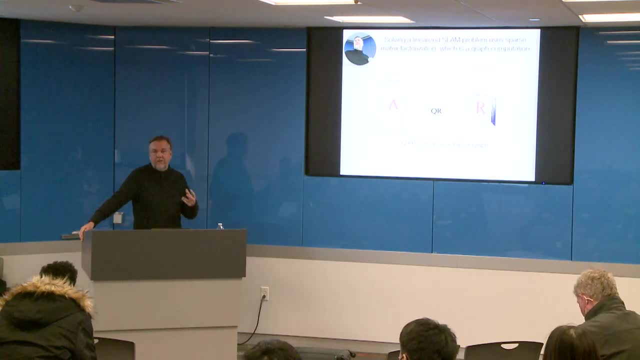 She's very well known for constraint satisfaction. She's like the queen of constraint satisfaction solvers And she literally wrote the book on it. But before that she worked with Judea Pearl on inference in Bayes, nets and sort of graphical models. 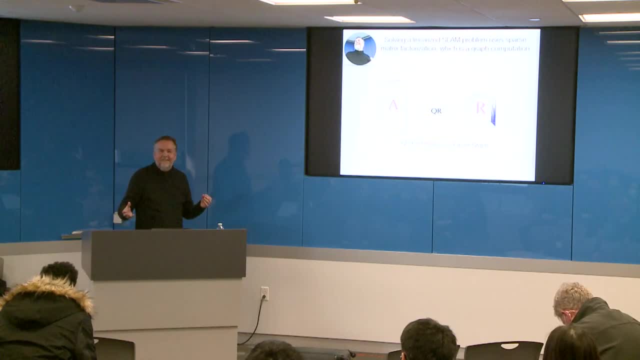 If, if you say graphical models in machine learning, where did they come from? They come from Rena Dichter. They came from Rena Dichter and Judea Pearl. Okay, And how you do inference in these Bayes networks is you can do that with bucket elimination. 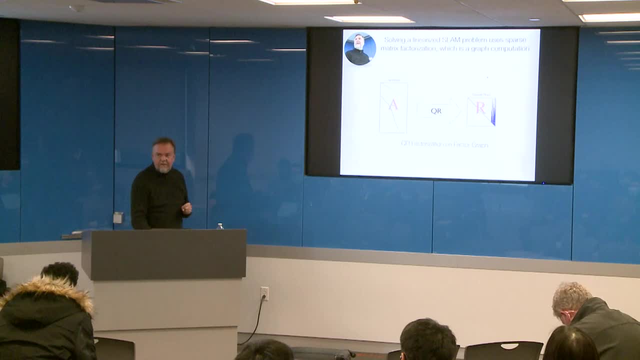 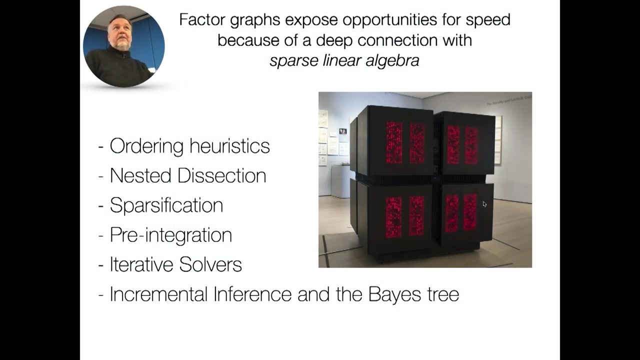 Back then. it's probably not as apparent to Rena that that bucket elimination is QR factorization in linear algebra, But so these things are all deeply connected. Yeah, In fact that's. that's that's the key advantage from the performance side. 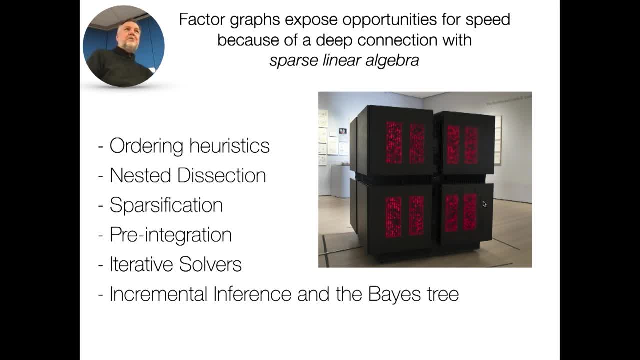 So there's a there's a human anthropomorphism, There's a human anthropological advantage of just talking about factorization on the, on the blackboard, But there is also a raw performance benefit, which is that if you expose that sparsity, 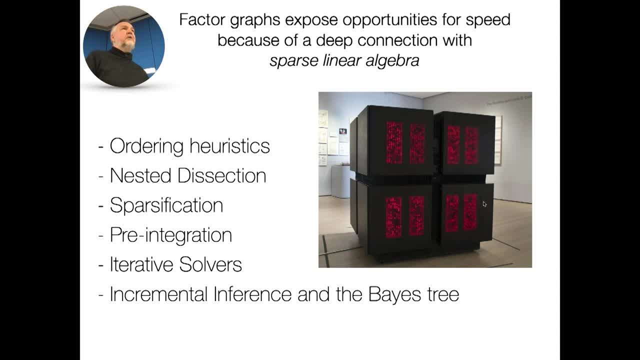 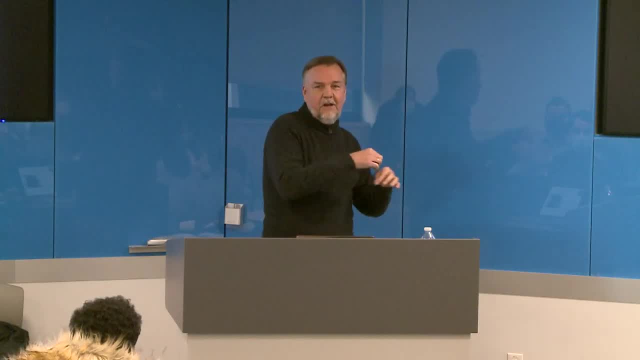 then you can use all the tricks from linear algebra, And, and, and. people that do linear algebra have come up with a lot of tricks. Okay, Heuristics on how to order the, the, the bucket elimination: How do you, how do you eliminate variables? in what order? 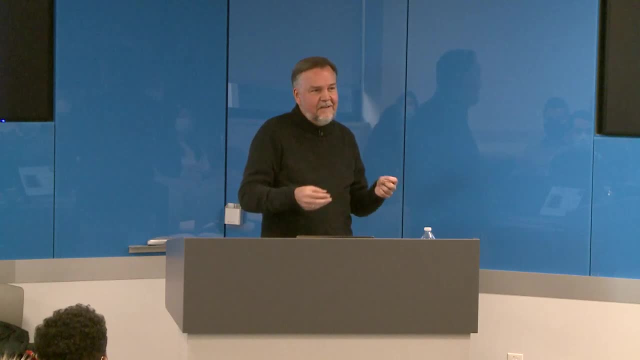 Okay, You know split up graphs. you know recursively That that is the famous finite element. you know separator theorem, et cetera. Is bucket elimination related to marginalization? or If you eliminate a variable, you have effectively marginalized it out? 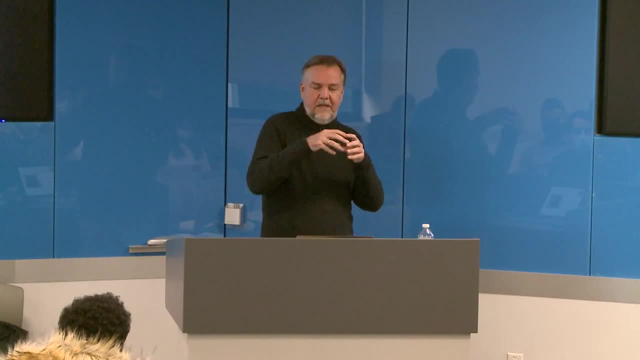 That's right. That's right. But what? what happens is you, you, you marginalize it out, but you also keep around the function that once, once you solve the problem. In fact, I, I probably don't have a problem with that. 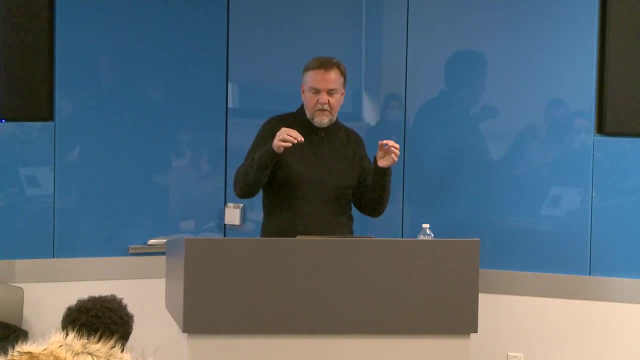 I- I probably don't have a slide on that, because this is not that talk, But you keep a function that if you then solve the entire problem, you can recompute what the optimal solution is for that variable. We'll see some examples later. 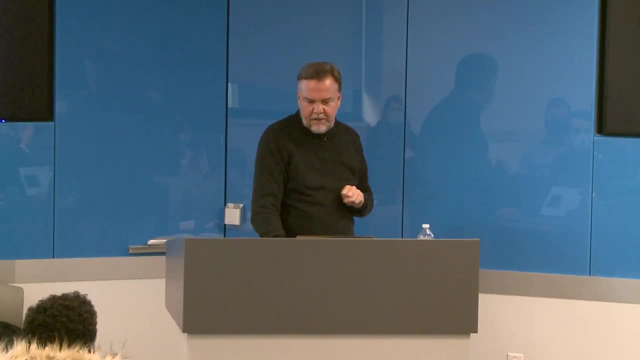 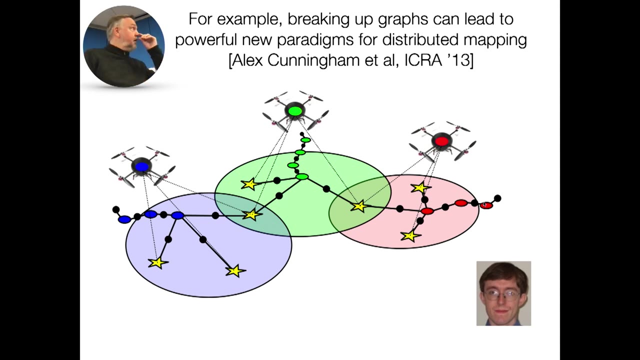 Anyway. so there's raw speed opportunities as well because of this connection with linear algebra And then- and we did a lot of that in, in, in, in in my group, So so so this is Alex, He who works at TRI now. 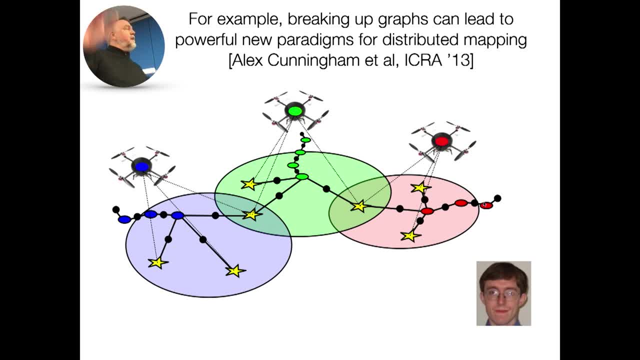 He was thinking about. okay, if you fly multiple drones, say, we build this massive factor graph, but could we cut it up in little pieces and solve pieces on the drones themselves and then just send some information back and forth to still solve the exact same problem? 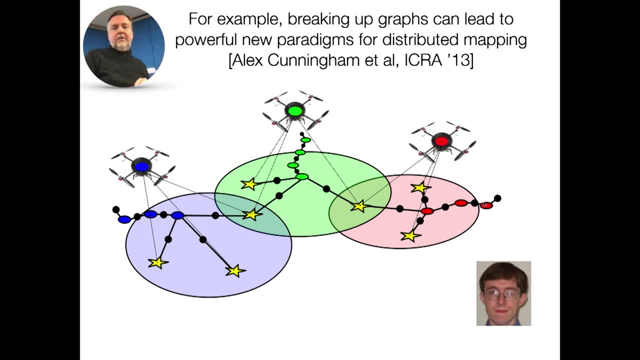 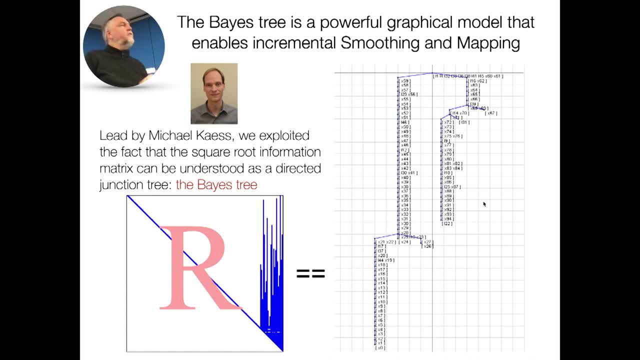 Okay, So that was a ICRA 13 paper With Michael. some of the most influential work we did is is: is think about: well, in linear algebra we did a lot of that. What was the? did the happines? 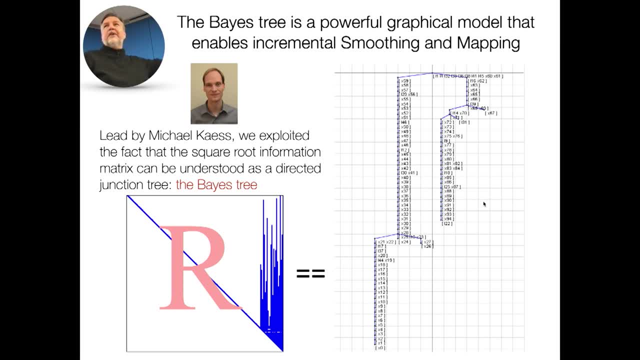 What are the things that you get? Well, what is the? is the is the upper triangular matrix, Because if a, if a, you do a wave in a need. well, it makes for a number of things. So you have this, this security matrix, or this, this unit of space. 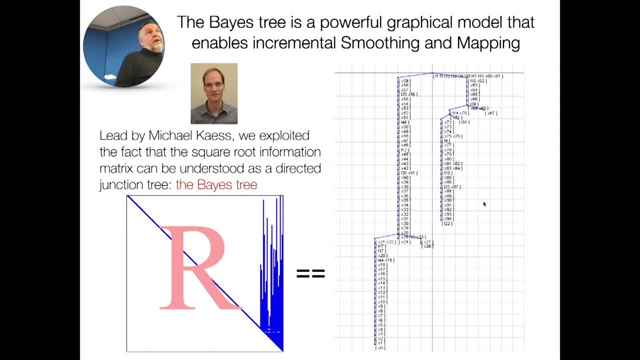 It's a going to be a rule of thumb, It's going to be a log of space And it's going to be a source of time. It's going to be a time for the data And if you get the point, you get the, you get the, you get the ccf of this data. 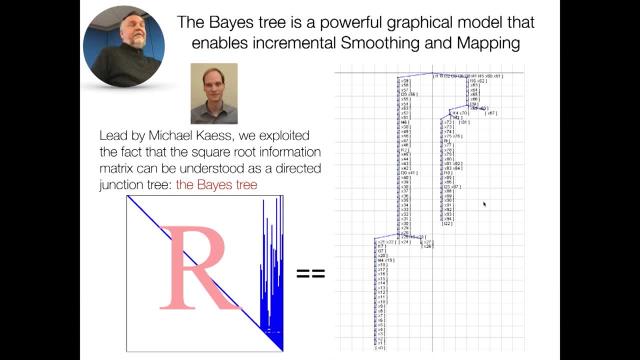 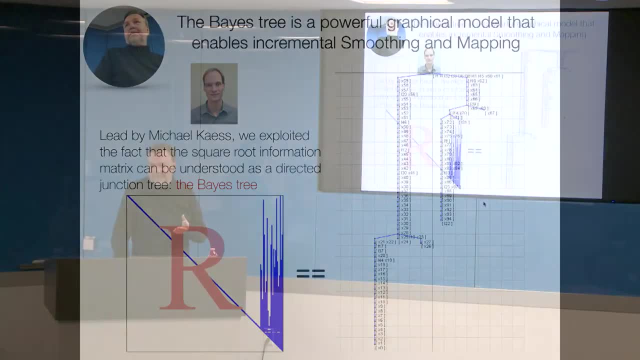 What do you get? Well, in linear algebra, the only thing you get from QR factorization is this ugly-looking upper triangular matrix which doesn't mean anything to anybody. All right, which is another graphical model from statistics and machine learning, which is the junction tree. 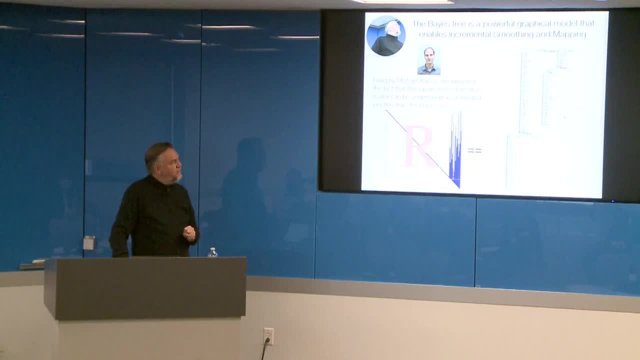 So it turns out, after you do inference on this factor graph, you get a triangulated base net which is exactly that R matrix. And not only is it a base net that is triangulated, but it has, if you look at the cliques of that base net. 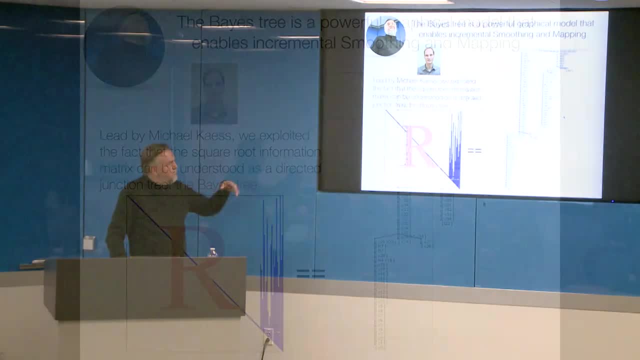 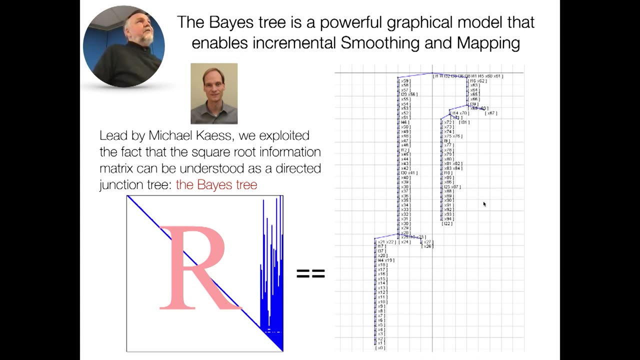 you get a tree structure which we call the base tree because we think of it as directed, but the undirected equivalent is basically the junction tree from machine learning. So again, a deep connection between all these concepts from graph theory, statistics, machine learning. 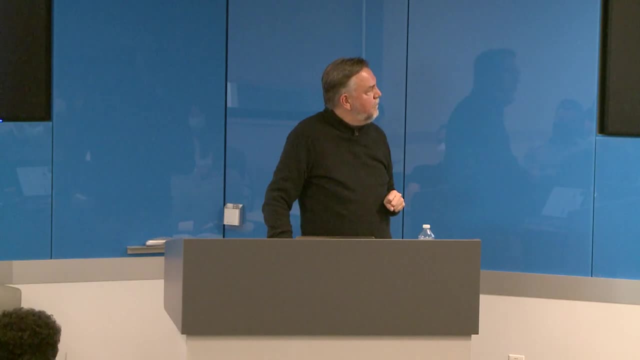 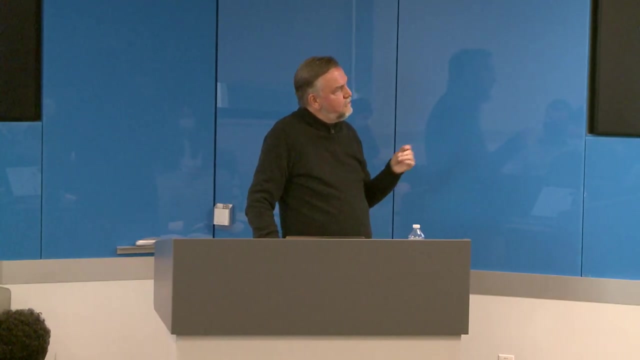 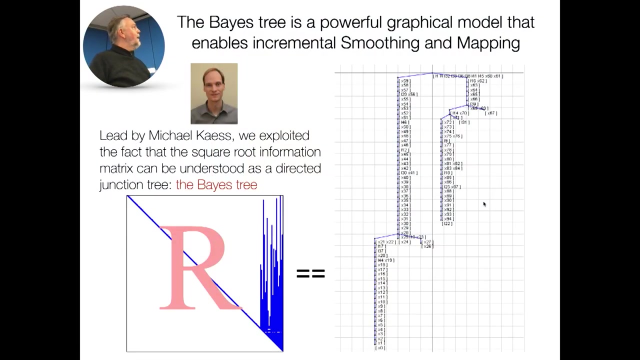 and linear algebra. And people do notice in linear algebra that there is a- they call it the clique tree- Okay, and it's used to create sort of large parallel solvers for multi-processor clusters And with this base tree we can enable 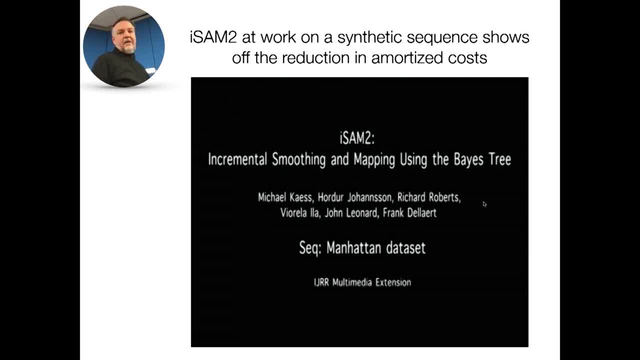 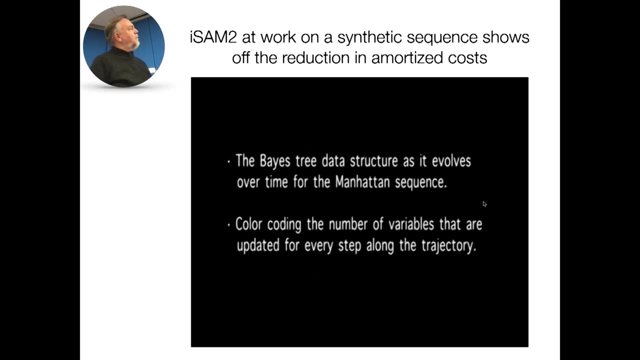 and this is an old movie. This is when Michael was a postdoc here that we did this work. So John is a co-author on this paper And that's our incremental SAM paper, where you will see that the base tree is created. 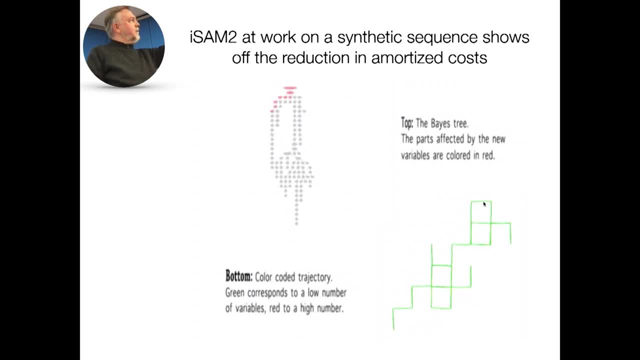 So every, Every green. So it's a robot exploring a Manhattan world. And then, if you inference on the SLAM problem, you get an upper triangular matrix, but nobody cares about that one. But the tree itself is laid out from the present to the past. 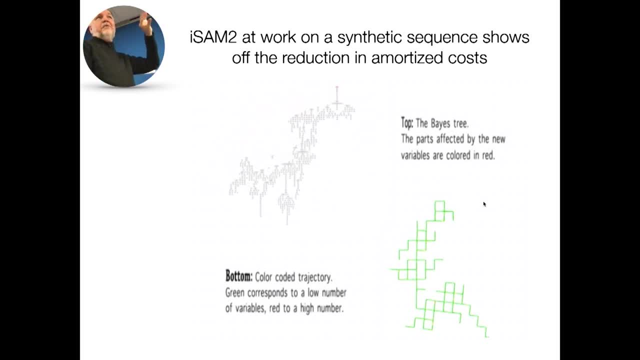 And because we lay it out that way, the tree is almost constant. Only the very top of the tree changes, And that is the key insight in making incremental mapping very fast, because, except if you have a loop closure, the computation is almost constant. basically, 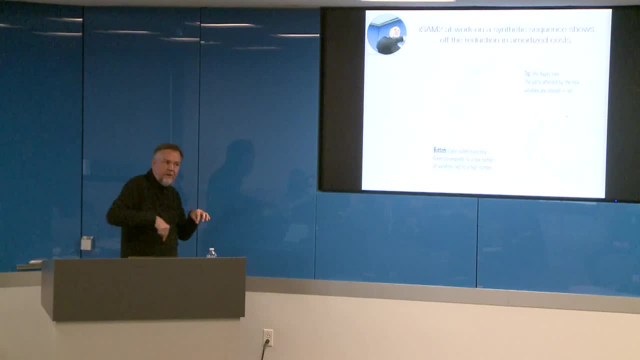 And if you have a loop closure, it depends on the size of the loop closure how many variables are involved as to what size of the base tree you have to recompute Right. And, by the way, again making a connection with Rena Dexter, 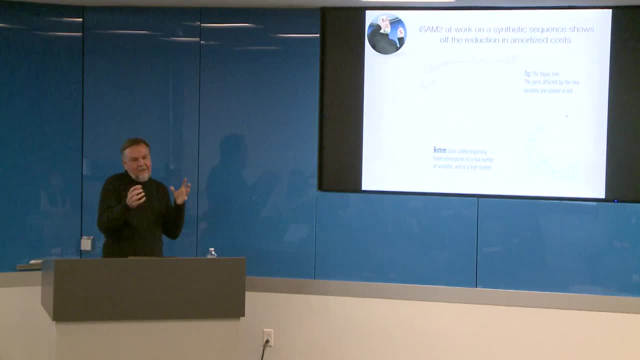 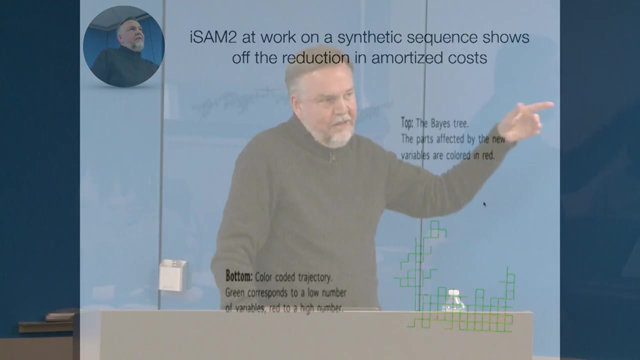 I guess I'm talking more about Rena Dexter here than about that. you know she's a hero of mine. She's really really great. She taught about all these computational aspects already, So she has mini buckets, which is really heuristic inside. 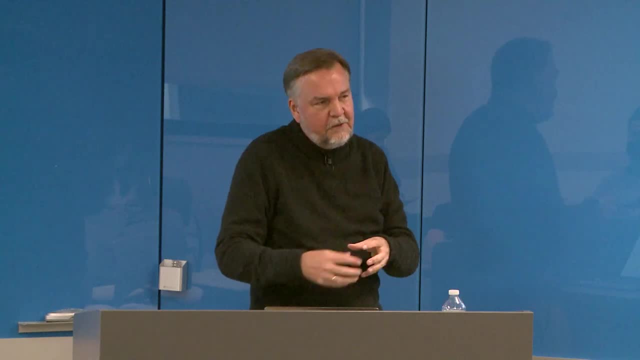 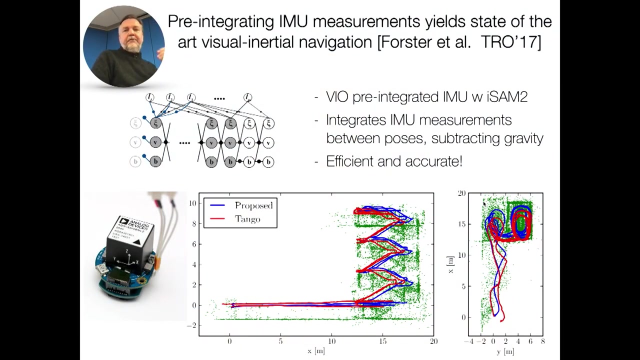 a clique tree to limit the size of the cliques that you're looking at. So a lot of this work is also present in papers in classical AI and constraint. satisfaction With Luca and Christian Forster. so Christian is a student that joined us for one semester. 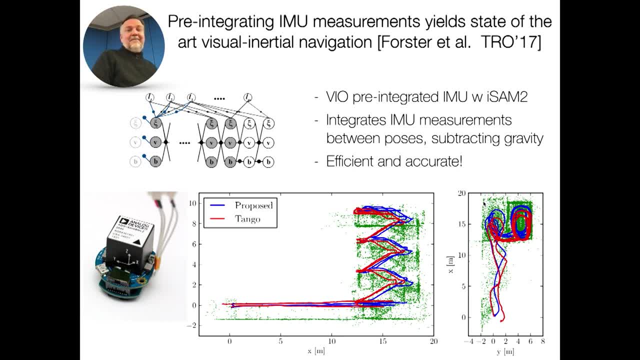 only in Wright And he's from Davide Scaramuzza's group back then at the University of Zurich. Davide is now at ETH. We took his really cool visual odometry pipeline and put it together with ISAM And the. I am you factor. 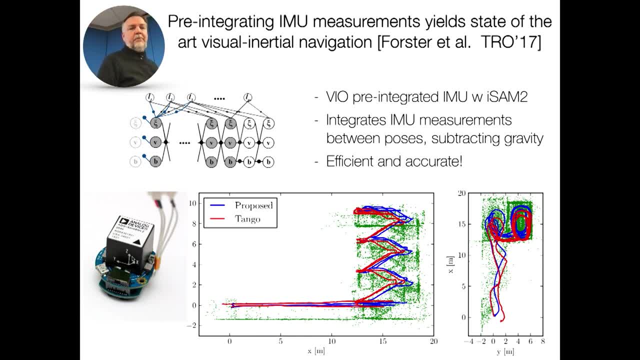 So this little gadget many of you will be familiar with. It's an inertial measurement unit. It comprises of a gyroscope and an accelerometer And it's a really annoying sensor. It's really great. if you just want to know how is my phone oriented? 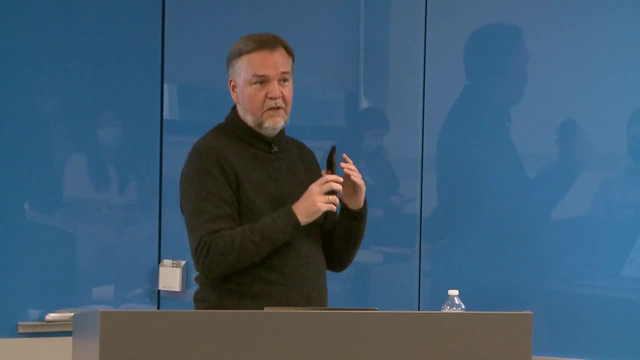 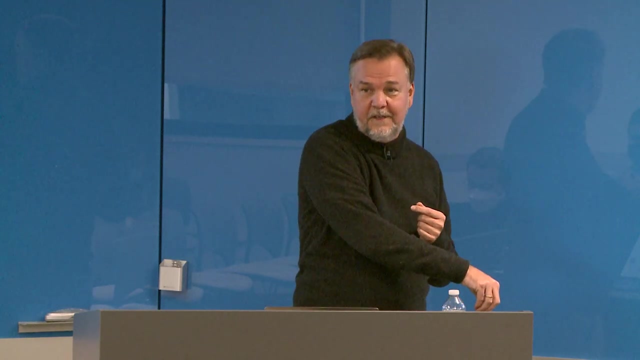 Which is exactly what the accelerometer does in your phone. The only thing that Apple uses the accelerometer for is points to gravity. OK, But what more nefarious uses of accelerometers can put an ICBM and launch it in the US and have it hit a target in Russia with 50 meters accuracy. 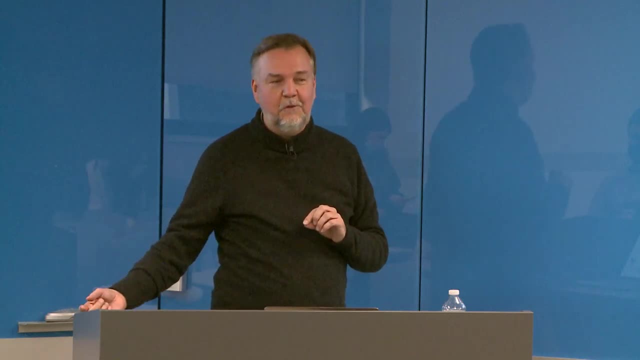 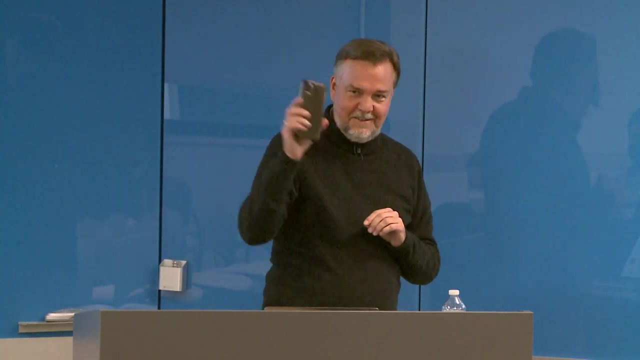 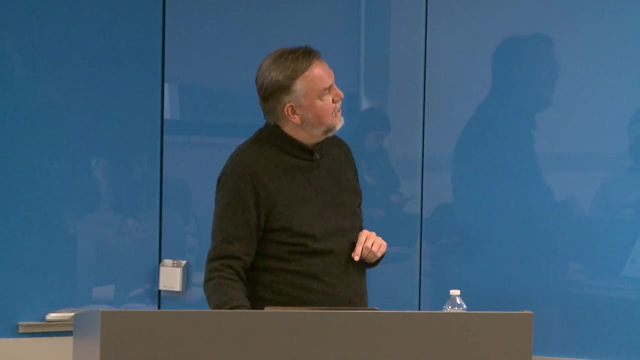 without any GPS correction. So that is what you could do if you had an amazingly good and very expensive I am you. Unfortunately that's not the I am you that's in these phones Or in the drone, So dealing with the noise is very, very hard. 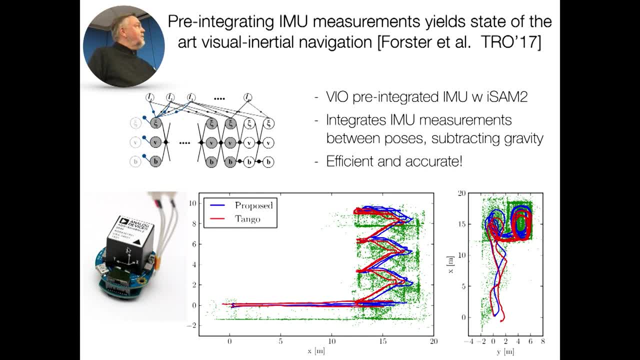 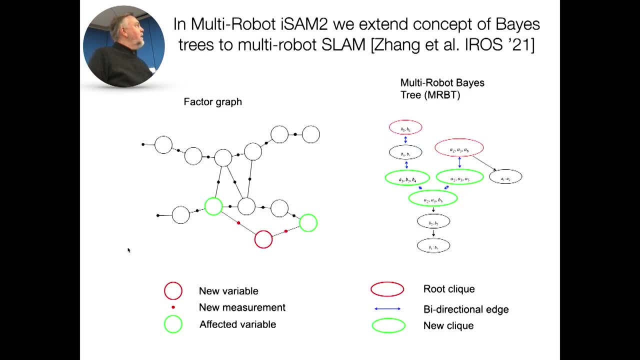 But we have a special factor in GDSAM that deals with this, So you don't have to solve it, And a lot of this is actually Luca's work. Most recently, we also started looking at new students, So this is a new student, Yatong Zhang. 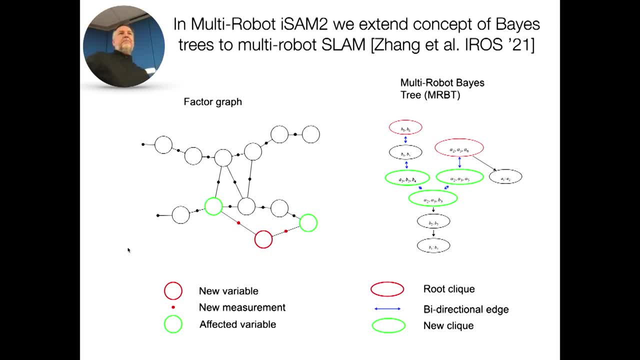 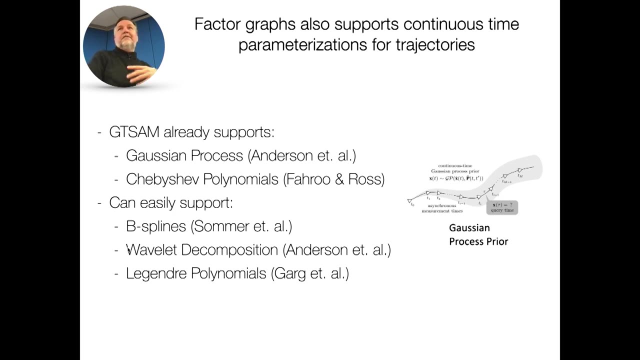 who looked at multi-robot SLAM. So we expanded the notion of a base Three, two, one with multiple routes. So that's work done with Facebook Reality Labs. And then, finally, I also want to say, in response to a discussion I had with Ross, 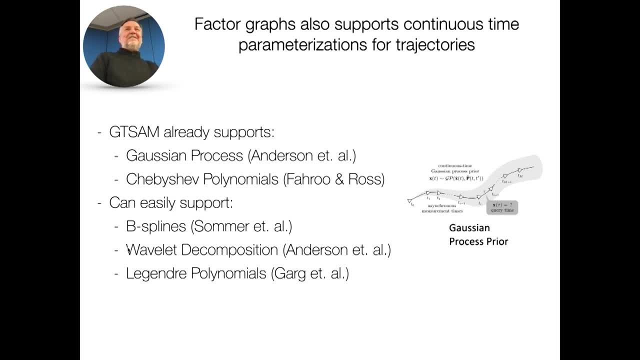 these slides were made before this, But you could get frustrated with this notion of: hey, do we really have to discretize time, finally, and then think about the state. I mean, what's the state of the robot at every one of these times? 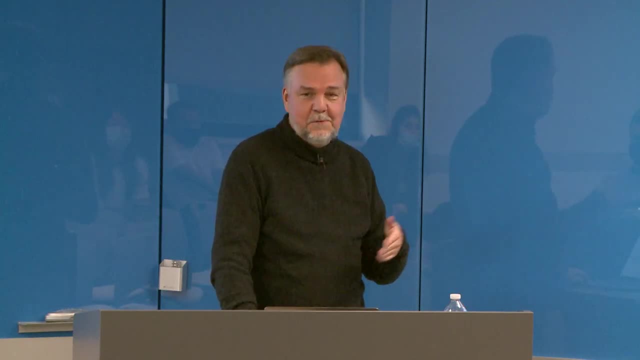 So one way is to think about time asynchronously, which people do in simulation. So there's this guy, Ethan Grinspen, at NYU or Columbia. He thinks about simulation in a very cool way, But you can also do something else. 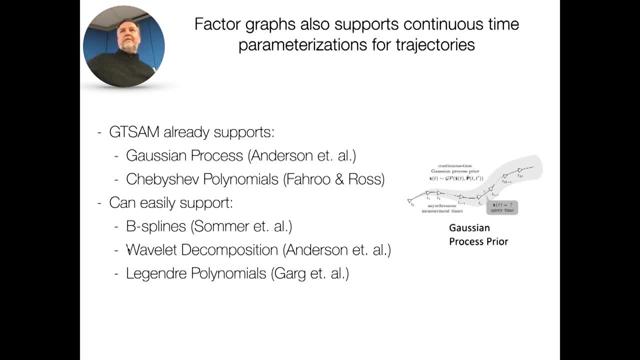 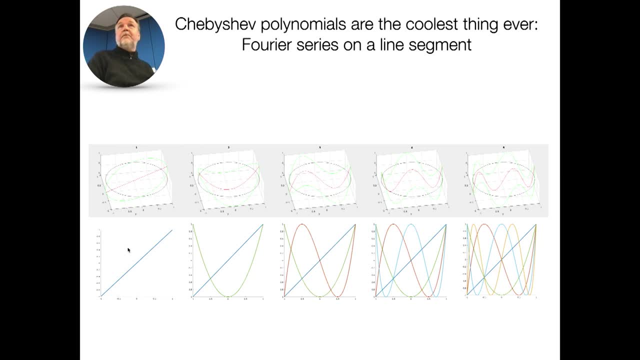 which is have continuous time parameterizations for trajectories. So, for example, B-splines or wavelets or polynomials, And my favorite polynomial I already talked about at MIT at one point- is the Chebyshev polynomial. In fact, I also consulted for a company in China. 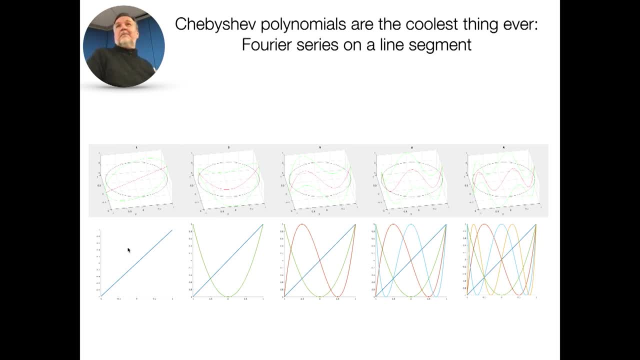 an autonomous driving company started by one of my former students, Nick Kai, And every person in the company had a nickname, which was a mathematician. OK, Now, they couldn't pronounce these names, So it was really funny to visit them and try to parse what mathematician they actually. 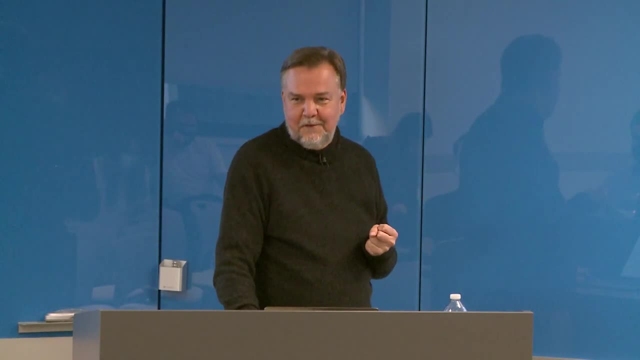 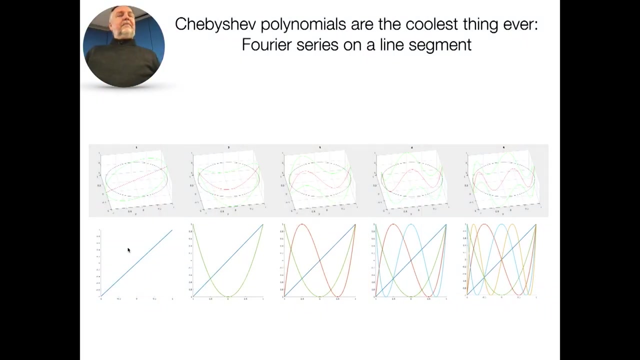 referred to, But my nickname was Chebyshev And Chebyshev is a polynomial basis, which is really cool. You all know a Fourier series on a circle, So you can basically approximate any function on a circle infinitely closely by adding more cosines and sine. 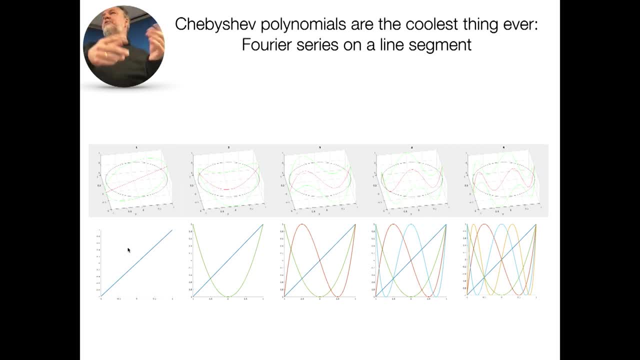 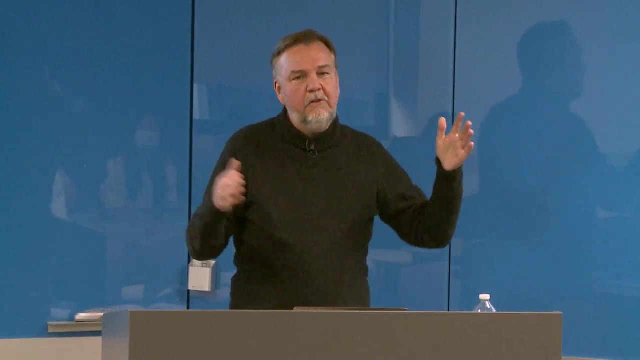 But in robotics we typically have trajectories with a defined start and a defined endpoint, So it's not periodic. So how do we have a? what is a basis, the best basis for trajectories? Well, it turns out you can just take all the cosines. 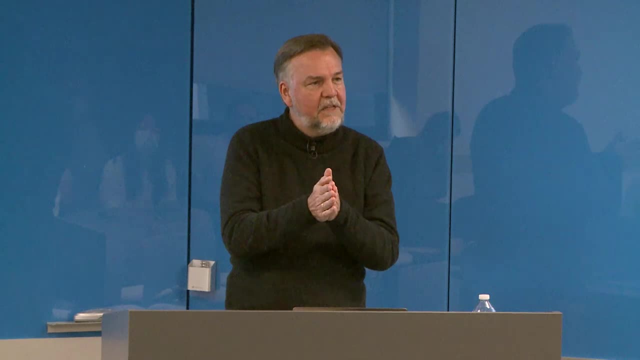 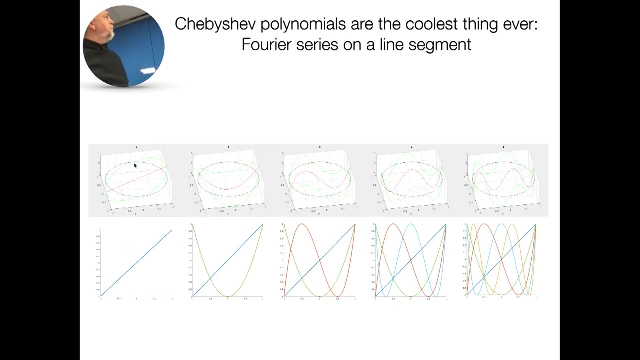 of the Fourier series and collapse them onto the midline of the circle And magically it's crazy, but magically these things are a set of polygons. So you project a cosine of period, one, one period, onto the midline and you get a linear line. 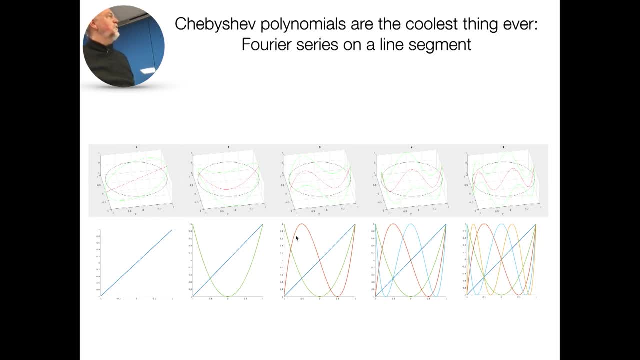 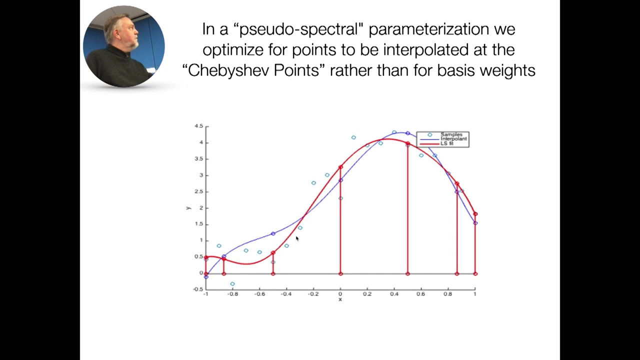 You double the frequency and you get a quadratic. You triple the frequency, you get a cubic, et cetera. So those are the Chebyshev polynomials. So in GDSAM we've implemented those And you can parameterize them in two different ways: spectral. 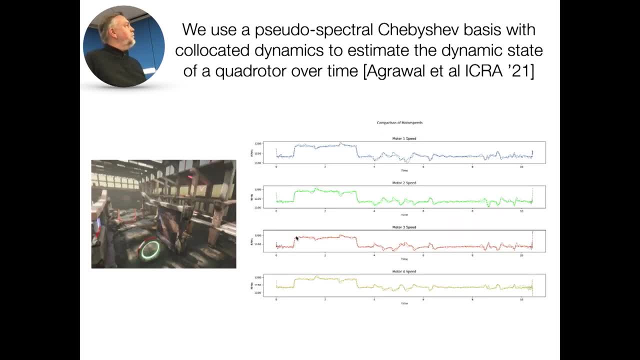 or pseudo-spectral, But we use them then to do state estimation on drones. This is with Varun Agrawal, where you can parameterize everything with Chebyshev polynomials over your entire experiments, Like not only the state. OK, and we 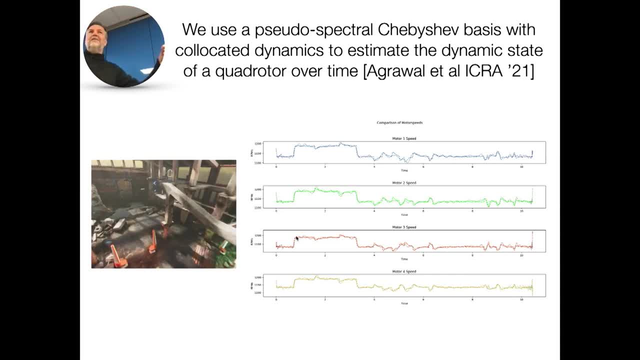 do this in tangent space of SE3. That means we have a polynomial in the tangent space so we can deal with Lie groups like SE3.. But also, these are the four trajectories of the motors So we can after the fact try to estimate. 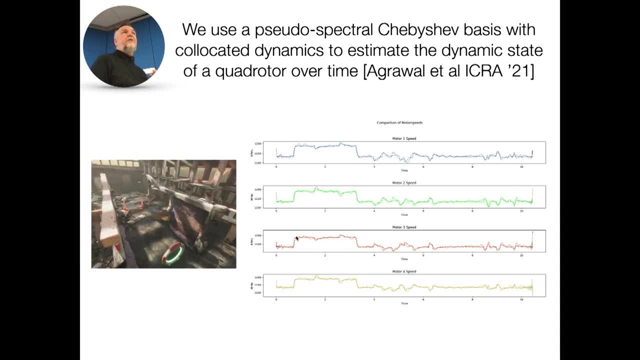 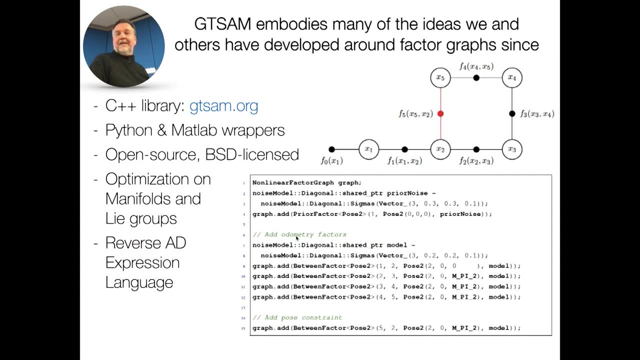 what the motors did, And that's interesting. Now we're bringing force. All of this is built into GDSAM. GDSAM is a C++ library that we've been working on for more than 10 years. Interestingly, it started out as a library. 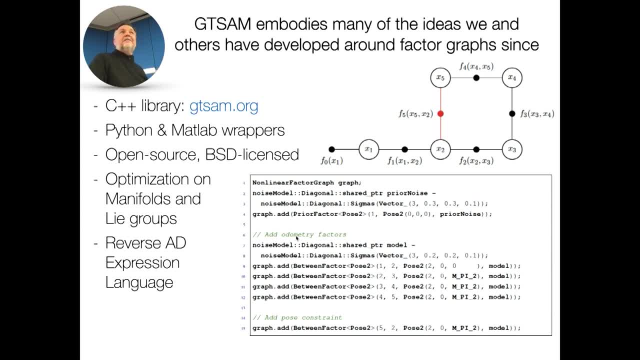 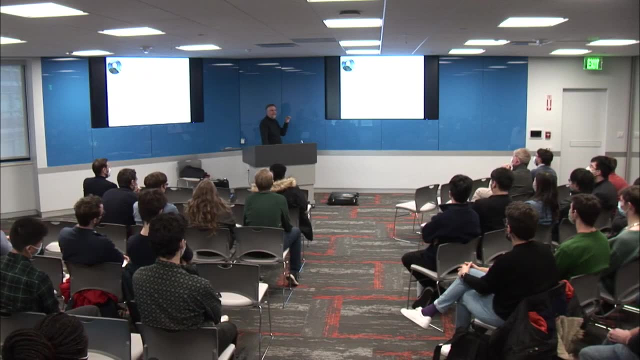 a library in ML, Raise your hand. if you know what ML is, It's always the same two people in the back that are raising their hands, So it's like camel, yeah, or machine. So camel is an instantiation of the language ML. 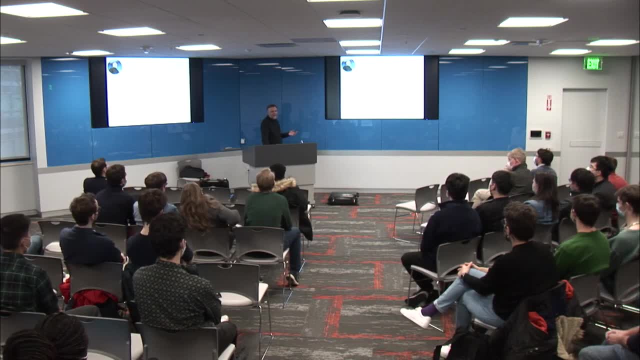 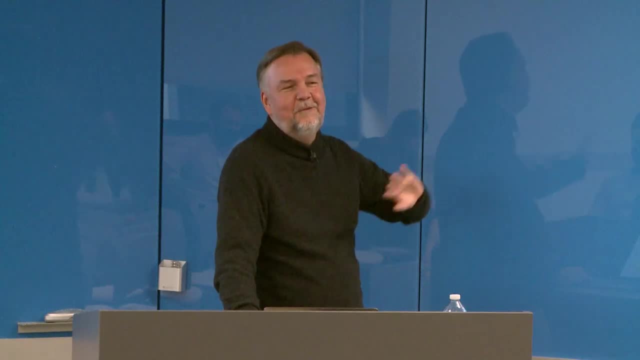 which is a functional language, And the first seven years of my professorship at Georgia Tech I did everything in ML, to the frustration of my students. So at one point we switched because I couldn't hire a student. But ML is a really cool language. 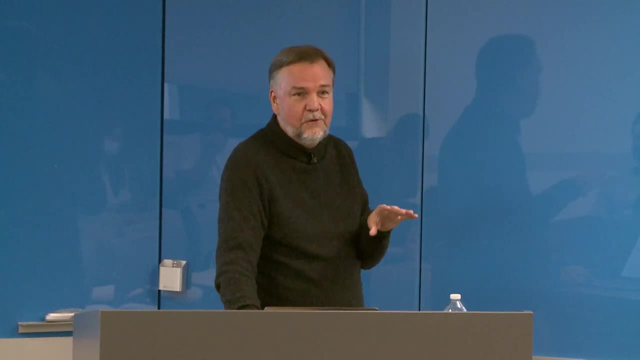 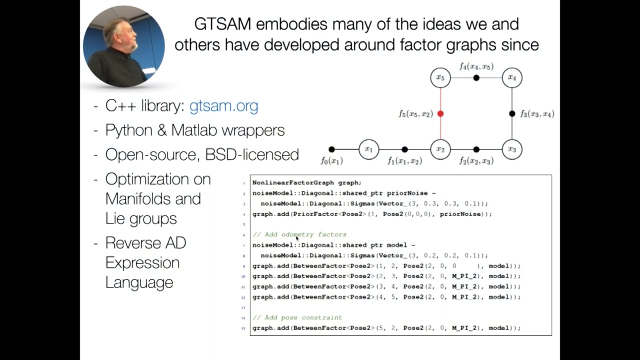 And so, by the way, Swift, and so there are really cool languages that are never used. I guess you guys like Julia, So I really should get into Julia, maybe Or not. John is like: no, not Julia, But this one is C++ based, but we do have wrappers in MATLAB. 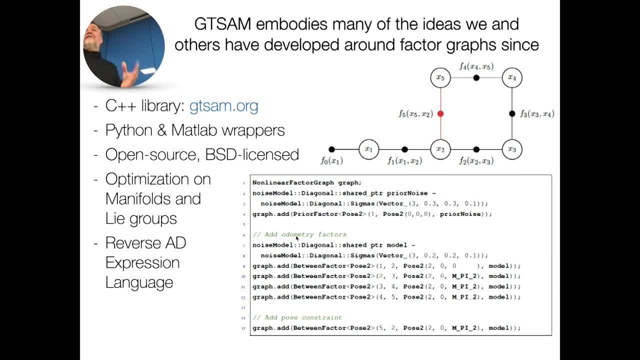 In MATLAB and Python. So you can just literally open a Colab, do bang pip, install gtsam and do import gtsam and you're up and running. It's open source, so you can use it to start your startup. 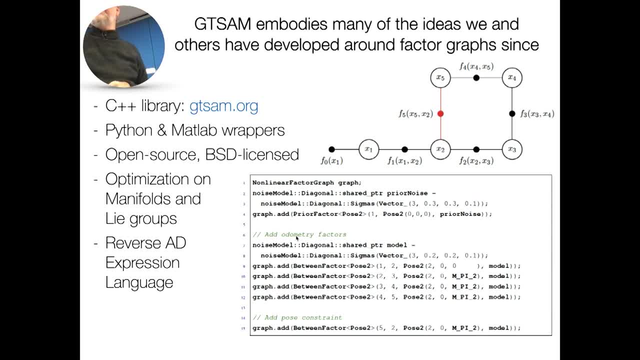 and become a unicorn startup without even mentioning that you use gtsam. It does optimization on manifolds and league groups And it has reverse automatic differentiation built in So you can build computation graphs and then you don't even have to compute the Jacobians numerically. 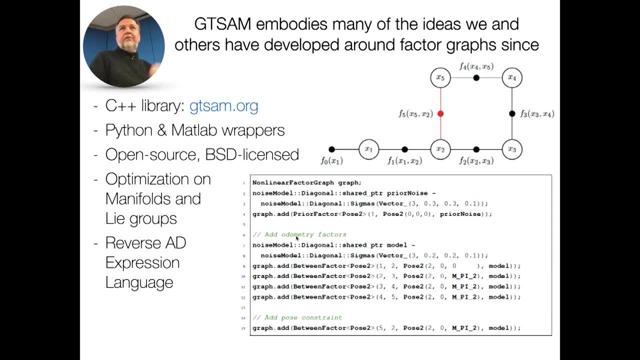 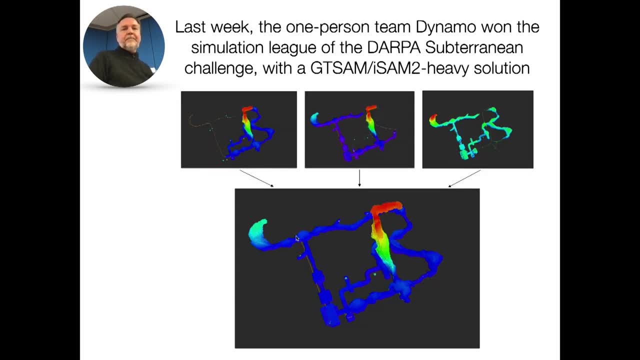 or manually, So free for you to use. And it uses factor graphs, of course, as the main computational substrate. And, by the way, this is a slide I wanted to change. I gave this talk one week after the DAPRA, subterranean. 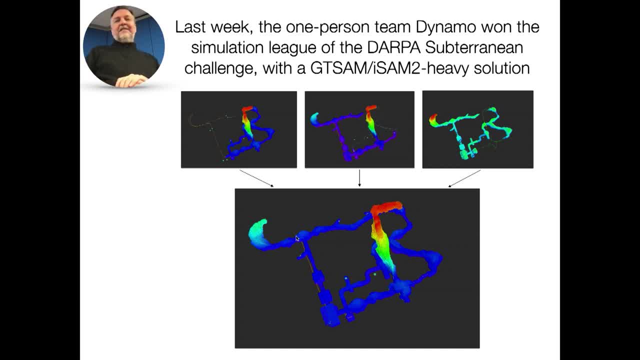 Challenge. It turns out that the simulation league was won by one guy, Hilario, from Barcelona, who had a simulation of five quadrotors And he used gtsam in at least two different ways. He used isam and a gtsam for post graph optimization. 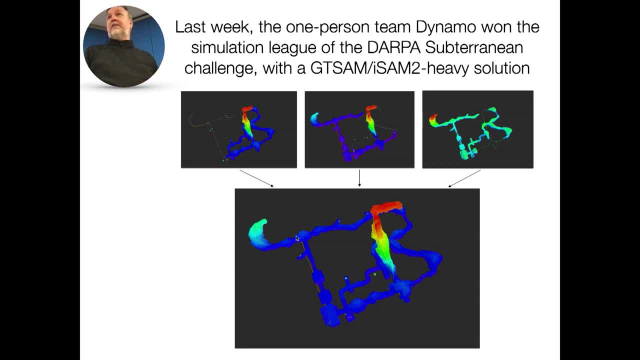 Won the simulation league and with that also $750,000.. One guy, All right, Which he's done, He's done To his credit. he's pumping that $750,000 in his new startup in Barcelona. But very cool right. 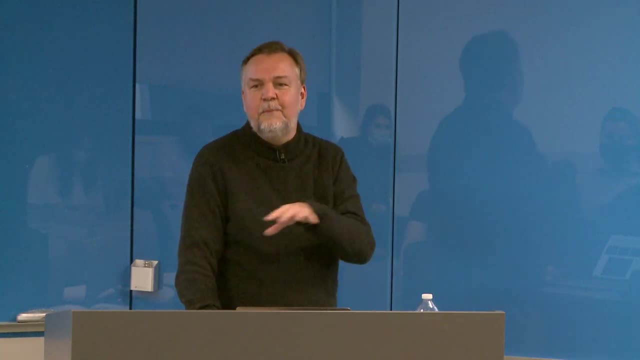 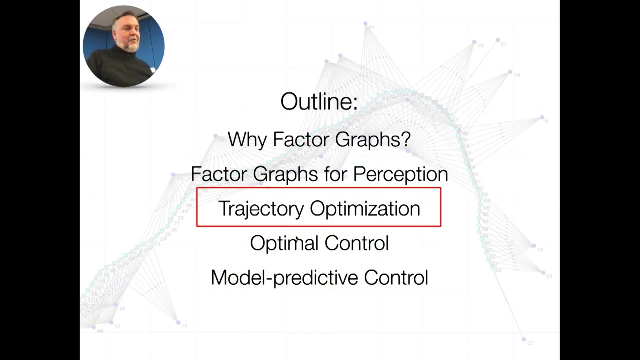 So you can use gtsam as a secret weapon to make lots of money is basically what I'm telling you. OK, All right, So I spent most of the time to talk about it, So I'll quickly go over things that we. 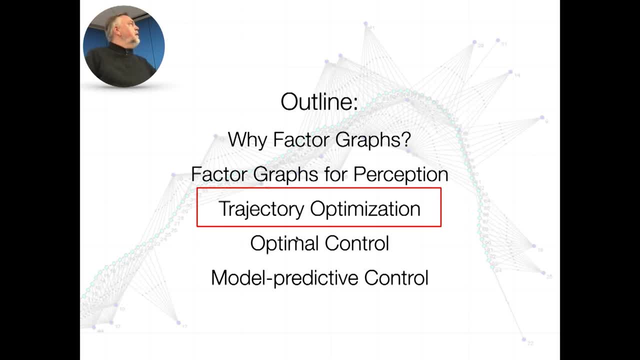 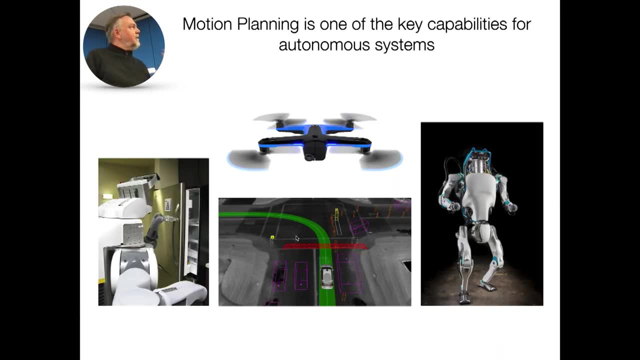 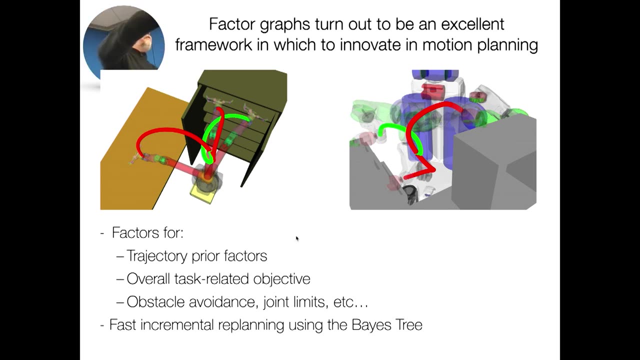 did for trajectory optimization. That's sort of the easiest transition. So with Byron Boots, Who is now at UW, We tackled motion planning. So motion planning is complex. You have to make lots of discrete decisions and sort of go left or go right. 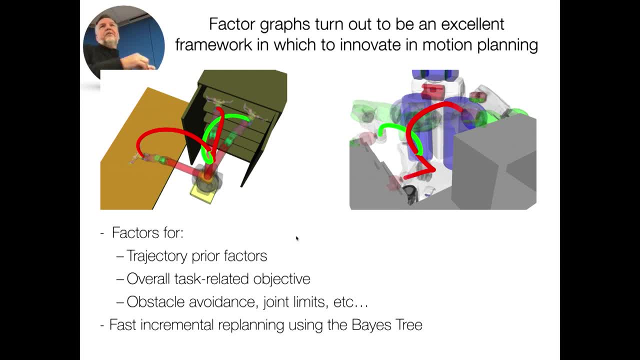 But once you know where you want to go, you can think of this as trajectory optimization. Right, So you might have a sampling-based planner that tells you, OK, this is roughly how you should go, And then you solve for the joint angles of your arm over time. 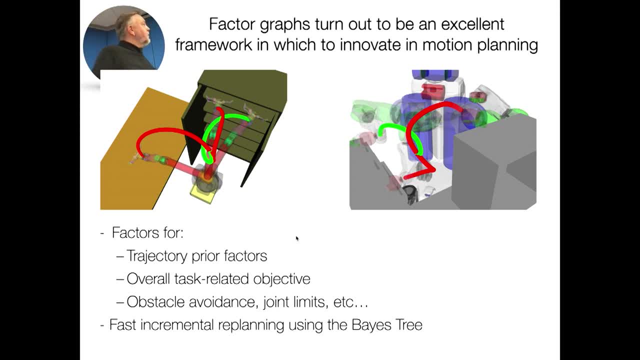 Maybe with Chebyshev. Chebyshev polynomial say right, But it's relatively easy to then put this trajectory optimization problem as a factor graph. You just add factors for your priors on the trajectory. You want some smoothness. 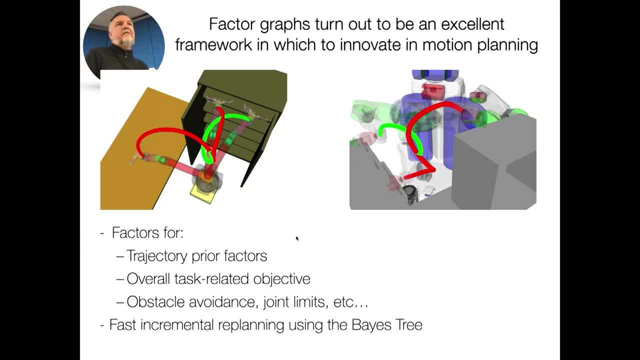 You want task objectives, like don't collide with things, So you can use sine distance functions around obstacles. You can add factors for joint limits, et cetera, And then you can use all the tricks from SLAM and Michael Case's ISAM. 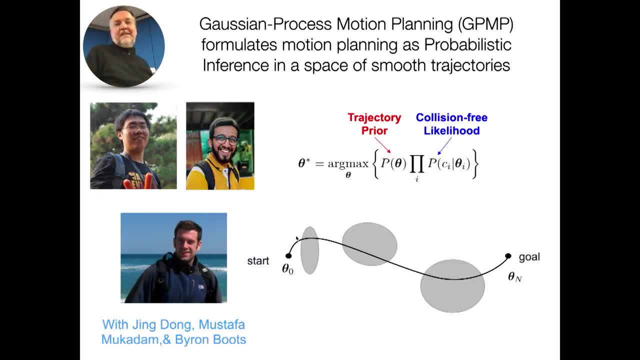 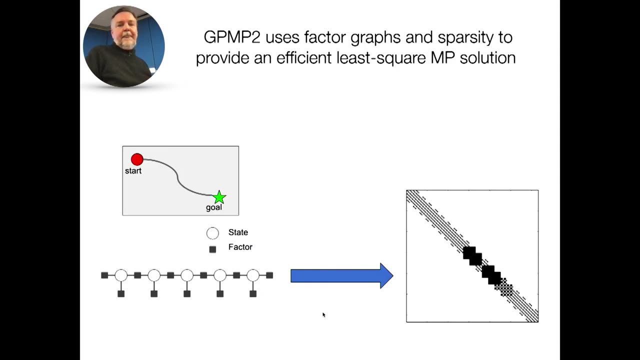 To do this really fast, Right? So that's exactly what we did. This is Jing Dong and and then Byron. So the prior that we used in this set of papers was a Gaussian process Prior. that's a smooth set of trajectories. 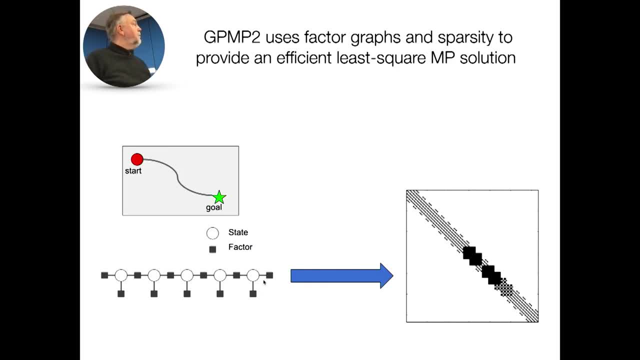 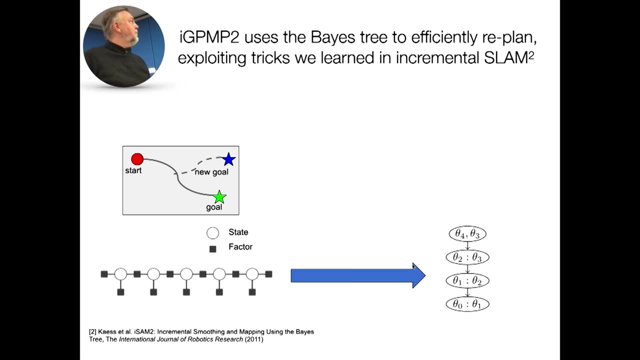 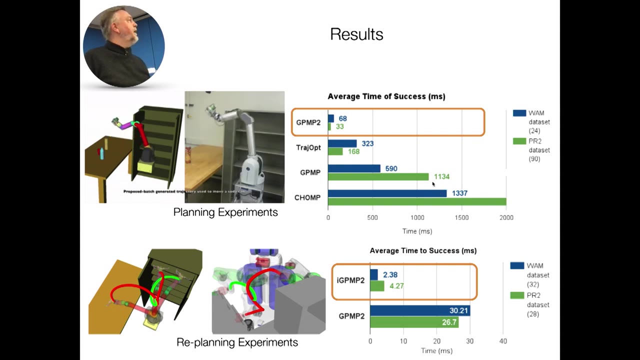 We literally encode it as a factor graph and then solve it, And then also solve it incrementally And we showed that the traditional trajectory optimization motion planners are Chomp and TrajOpt And just by using all the techniques that we discovered by reading papers in linear algebra. 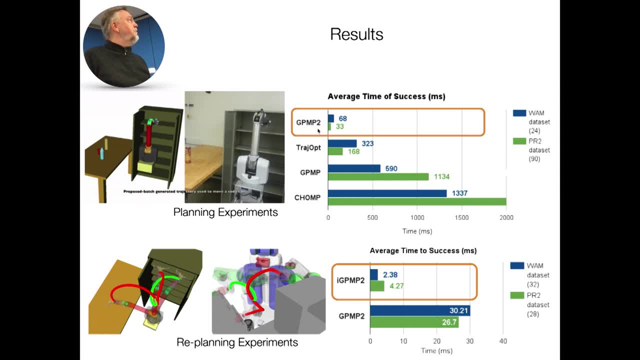 et cetera. we built GPMP2, which immediately beat the state of the art by a factor of 10. And then this is for a single plan, from a single start to a single goal. But if you in the middle sort of start changing that, you can. 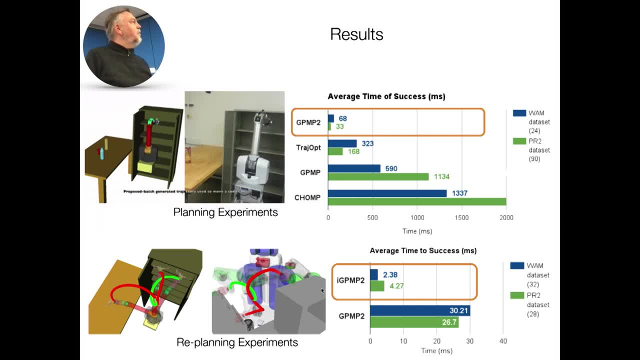 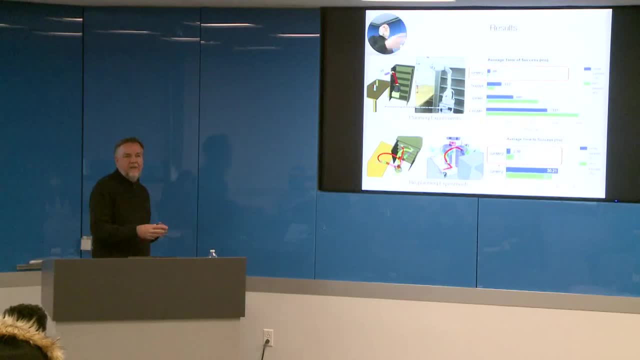 start changing your minds. We can do incremental planning another order of magnitude faster. So if you did most of the work already and if you change just your goal, then actually it's fast to change your mind. Yeah, this is actually pretty sparse. 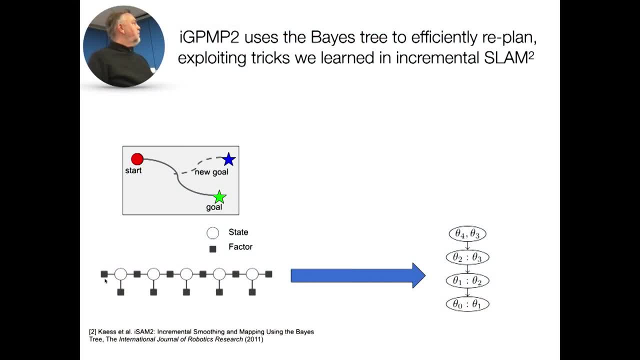 So this is really like a Markov chain, with smoothness on the trajectory and unary factors that that do that do obstacle avoidance. So this is- this is not necessarily the most difficult motion planning problem- The obstacle avoidance constraints are they applied at all times? for instance, 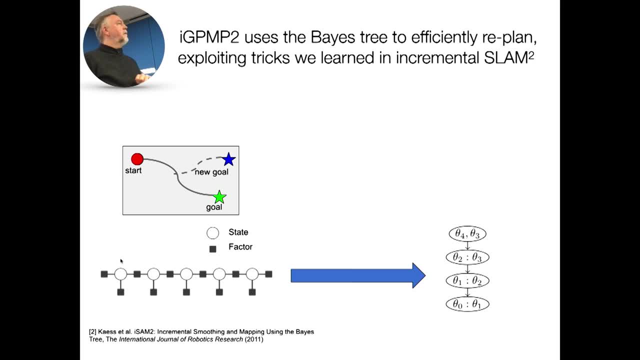 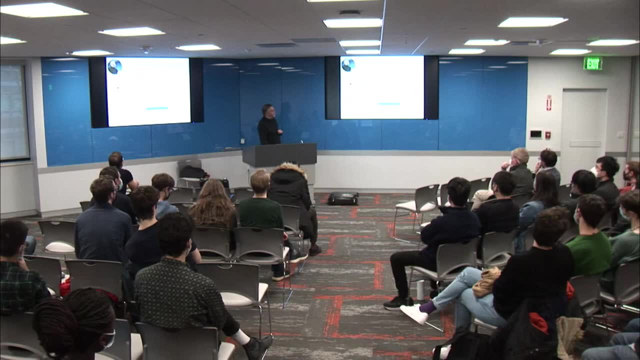 Or I mean, of course there's the dynamic sparsity in that sense, but do you apply the same constraints at all times? Or do you like, in your post-graph optimization, talk about you see only a landscape from a few time? 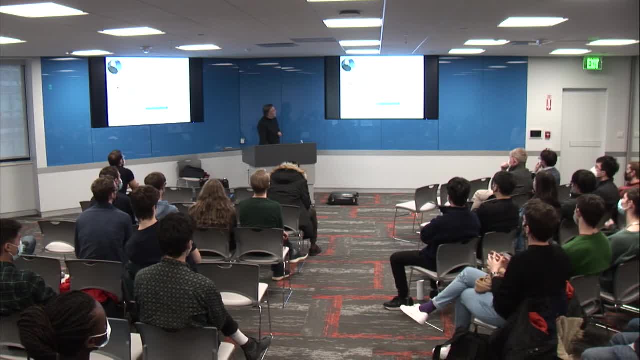 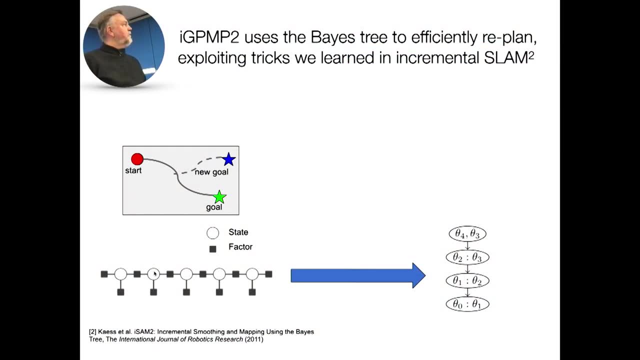 samples. Can you exploit that in the trajectory optimization case too? Yeah, so the factor graph here is actually quite simple, right? So it's really. we're just trying to solve for the joint angles at time, one time, two time three. 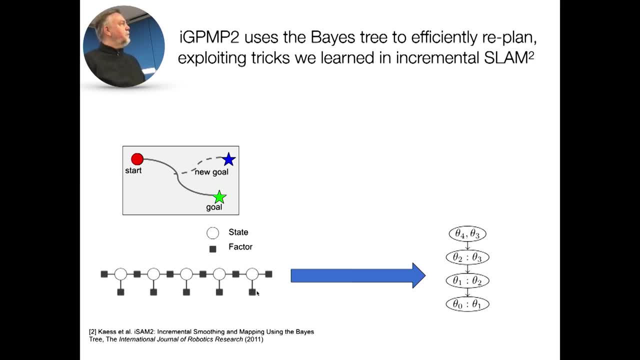 time four time five, And at any one of these times this unary factor says: I don't want to be inside an obstacle. And so it's sparse, because it's really connected to one time step only. right, But we'll come back to more complex constraints. actually, 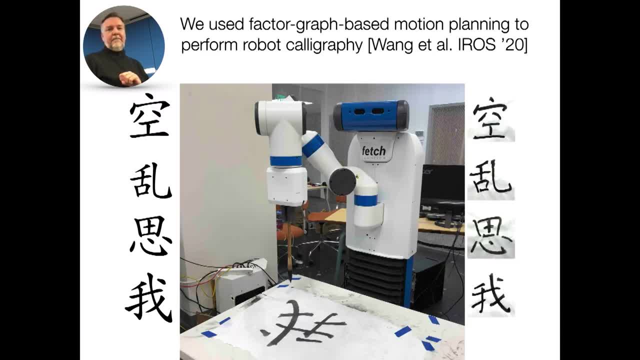 in like a couple of slides. I've also gotten interested in using robots for art, And so one of the first things we did is calligraphy. So we can this robot, the fetch robot. we did Chebyshev optimization for open loop control. 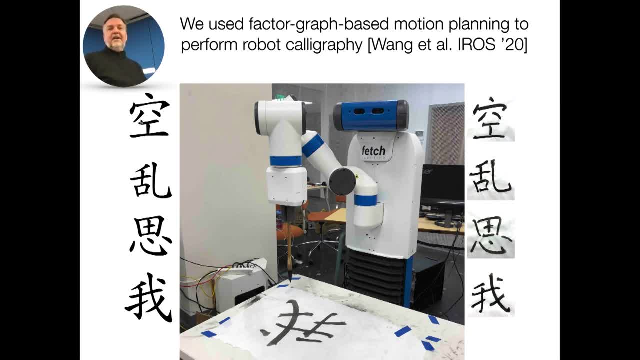 So any Unicode character you can give the fetch and it will try to paint it by solving an optimization problem with GTSAM Chebyshev polynomial for each stroke with a differentiable image formation model inside. It's still quite, it's still open loop. 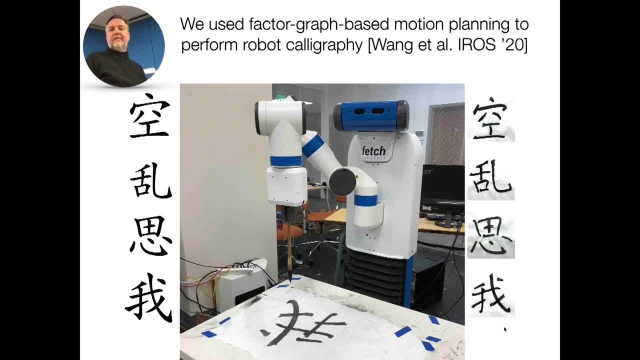 So my Taiwanese friend said that this calligraphy is at the level of an eight-year-old. But we're making progress. We bought a panda robot, So things are going to go smooth now because we can sort of bolt it to the table, whereas the fetch is on little rubber wheels. 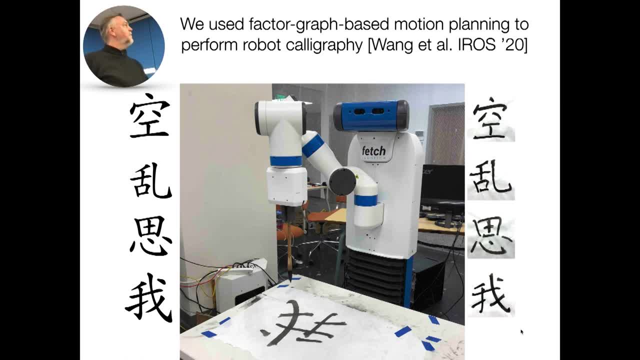 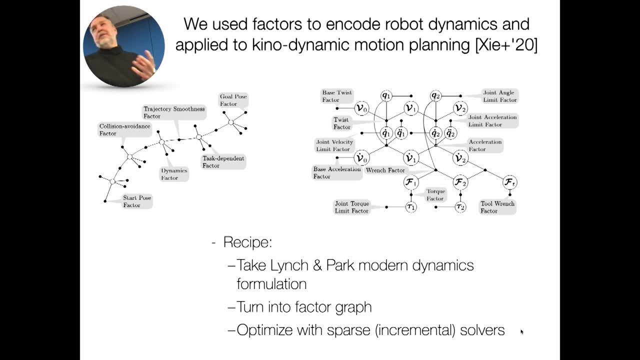 and we get sort of crazy things that way, And my student Mandy also. and so, Alberto, you're teaching. where is Alberto? There you go. So you're teaching dynamics. I've taught a mobile manipulation class three times now, and every time I got to the the coolest book. 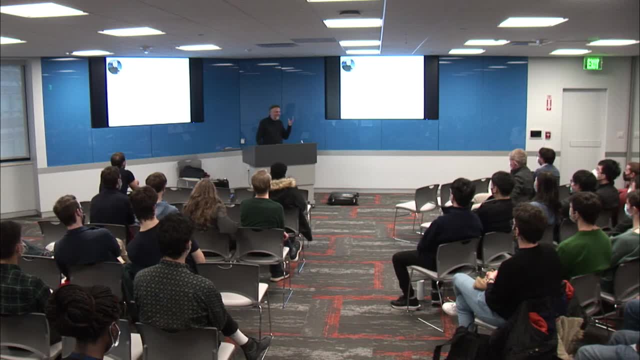 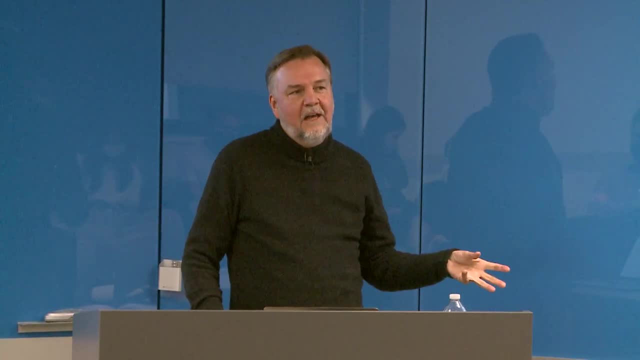 in that space of robotics I think is the Lynch and Park modern robotics book, a really cool book, very group, theoretic, very nice. But when they get to dynamics things start becoming complicated, even for grad students. There must be a better way to think about dynamics. 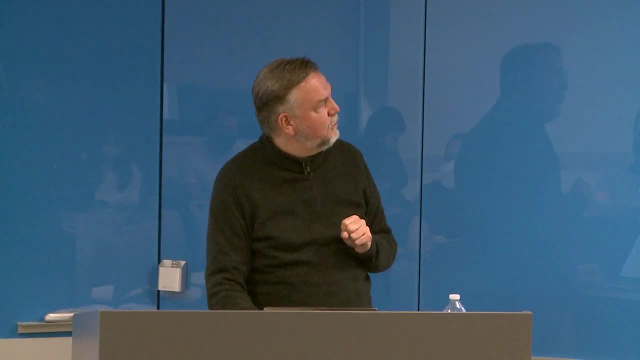 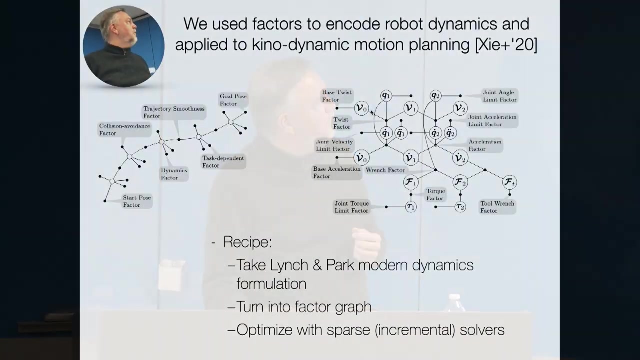 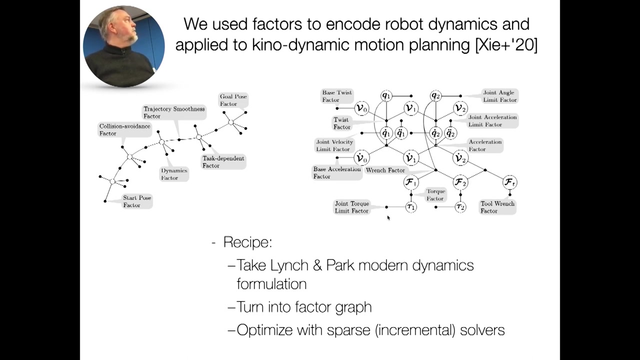 And so, with my student Mandy, we thought about: well, can we just encode all the dynamics in a factor graph? So for a two-degree freedom R, a two-link arm, we'll just introduce pauses and twists and twist accelerations. 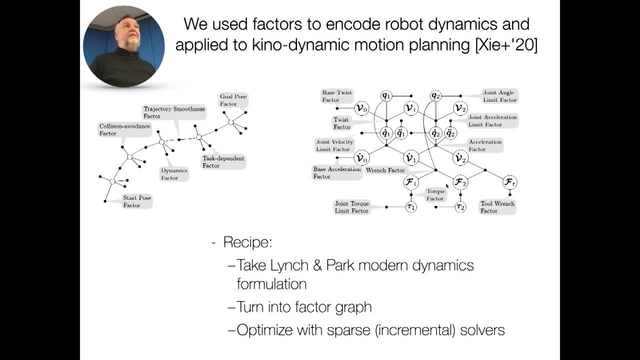 and wrenches and torques and just connect them all with constraints, And these constraints encode the entire dynamics of the robot. If you do bucket elimination on this graph, you get this very simple equation that you see in every robotics paper that does dynamics, with an m which is a function of q. 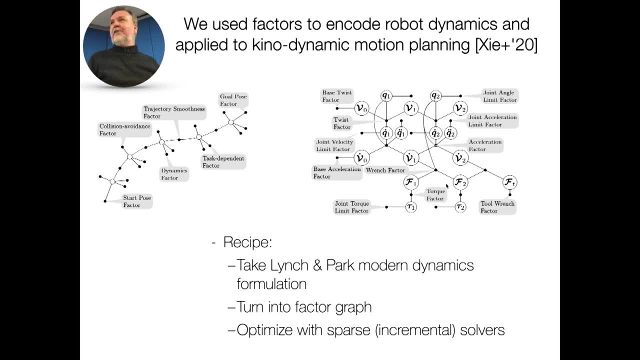 the configuration. But that's a complicated function, that m- Nobody tells you that. that mq is really complex And it's very dense. But this is a sparse graph which encodes in a sparse way that generalized inertia matrix. So yes, you can do bucket elimination. 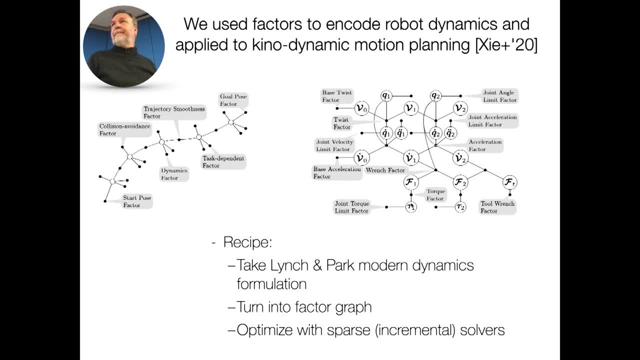 But whether it's wise to do so, that's an open question. So that's the recipe: Take Lynch and Park's stuff, turn it into a factor graph, optimize with gtsan. So this is an example of what Mandy did. 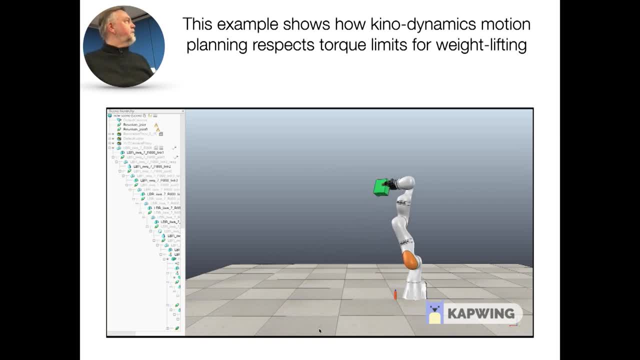 So you can see that. So she does kinodynamic planning with this. Here is a KUKA arm that tries to lift a weight, But the obvious way to lift it is not good because it breaks the torque limits, So you have to bring it closer to the body and then push it up. 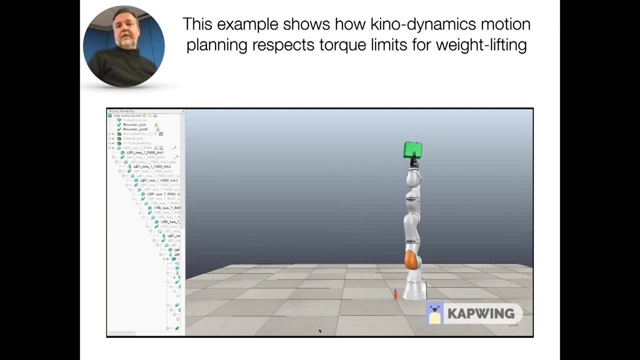 so you don't exceed your torque limits. And this is done by just laying out a factor graph with all these dynamics constraints and ask: solve this for me. So this is now motion planning with dynamics. I'm going to skip this. I'm going to skip this. 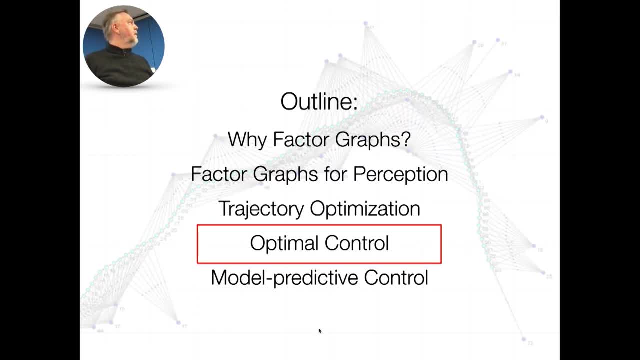 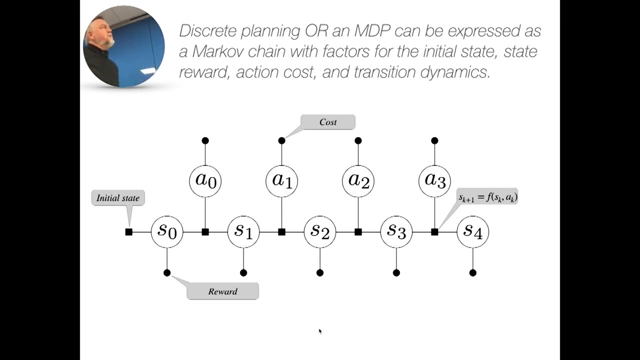 I'm going to skip this, But we also did some jumping robots with soft muscles. But I'm running out of time because I really want to talk about optimal control And, in particular, you can actually phrase any discrete planning problem or a market decision. 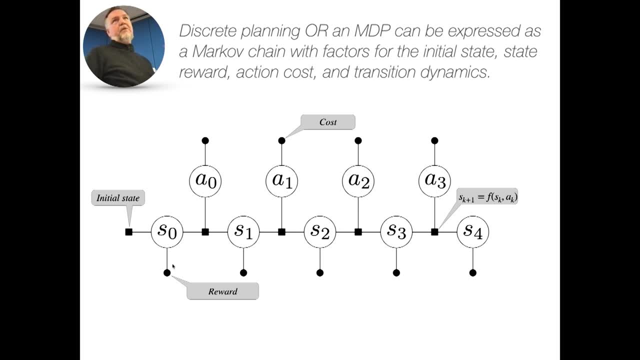 process with a factor graph. I mean, people already know that you can do it with a dynamic-based net. But I told you we can convert trivially any dynamic-based net to a factor graph. So here is the factor graph with discrete variables. 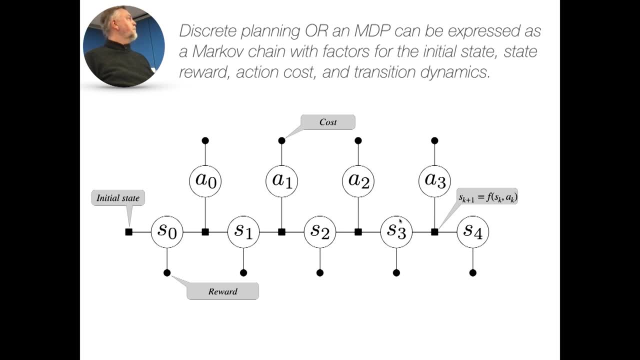 so discrete actions and discrete states, And the factors here are just well, this factor says s0 should be the initial state. There is a factor on s4, which is that better be the goal state. Then there is these unary factors that maybe reward the state. 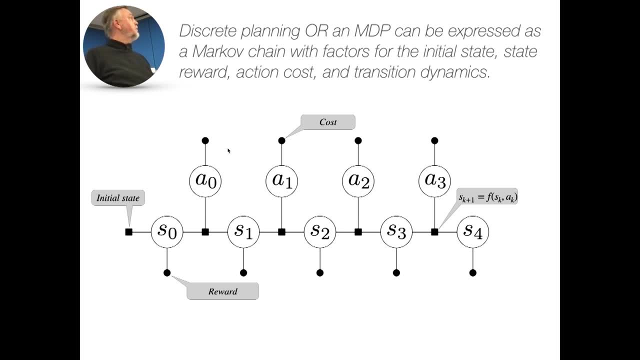 OK, So this is MVP. There is also costs for each action, And then the most important ones are these ternary factors here that say, if you do action three is this, then s3 and s4 better be in a particular relationship. 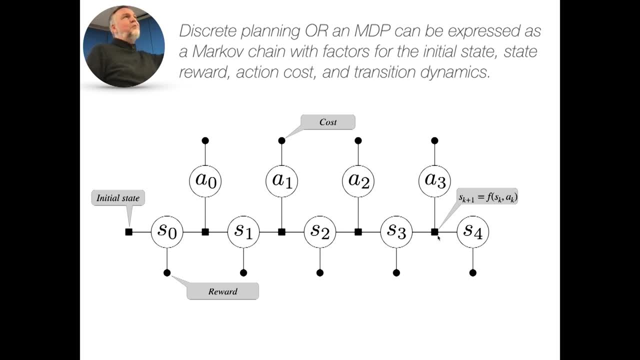 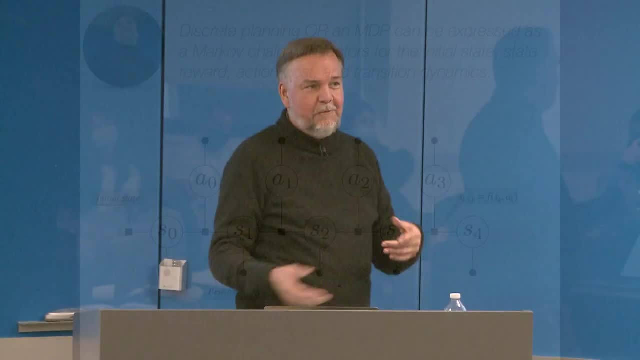 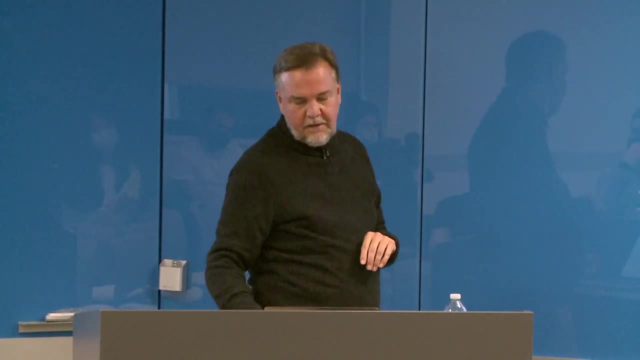 And that's a constraint. So this is a CSP view on discrete planning. And then you can just go to Reena Dekker's book and get one of her solvers and ask the solver to solve it, And now you've solved, basically, discrete planning. 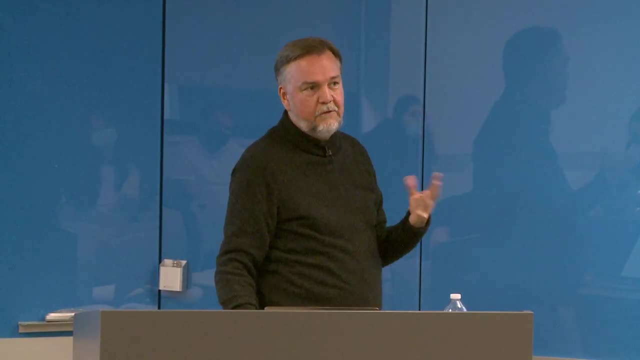 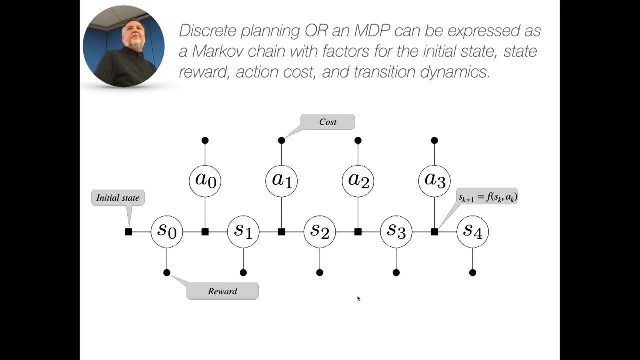 but stated as a factor graph, as a constraint satisfaction problem, and you solve it. The hidden problem is, of course, that it's exponential complexity, right. So people know that planning is piece-based, complete, so this doesn't solve that at all. 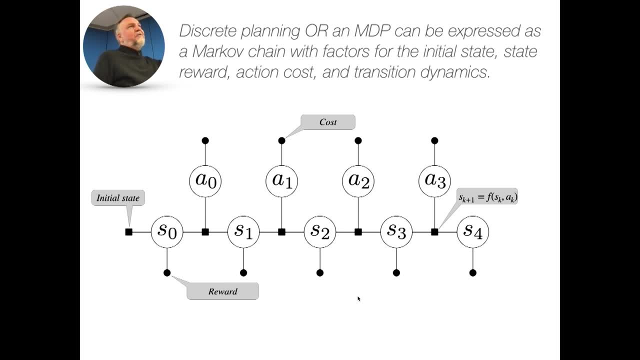 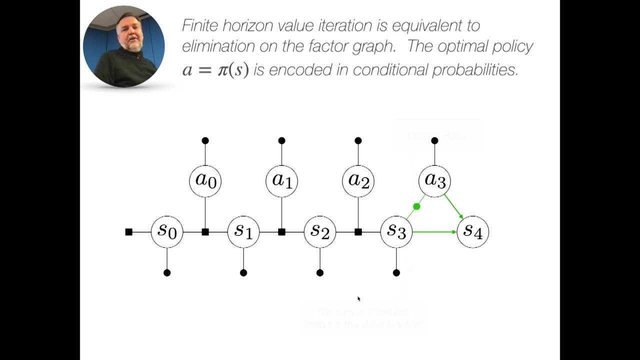 But it's kind of cool that the same factor graph that we used for it's very similar to the motion planning factor graph, right? OK, In fact. optimal control, yeah. so actually I'm going to skip this, but you can do bucket elimination. 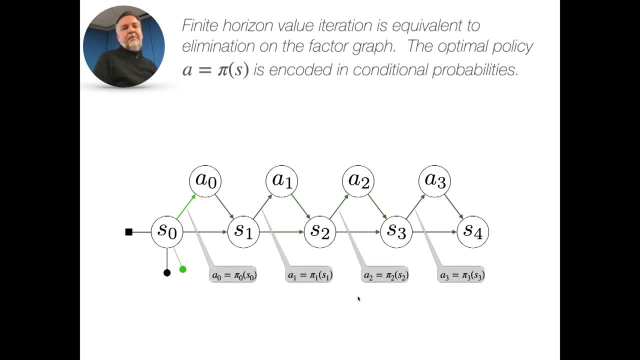 from the future to the past, And then what you get is actually functions that encode the optimal policy. This would be in an MDP. But you can also go the other direction and eliminate from the front. eliminate the front first and then go towards it. 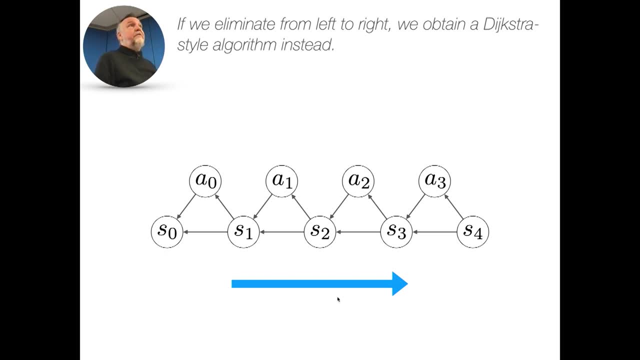 So back and that actually implements like a Dijkstra search in discrete planning. Or you can go middle out, which is a Silicon Valley joke. Who knows the Silicon Valley, Who understands this joke? OK, But if you don't understand it, you really. 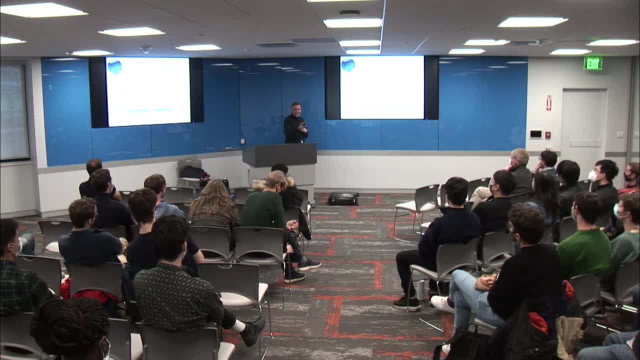 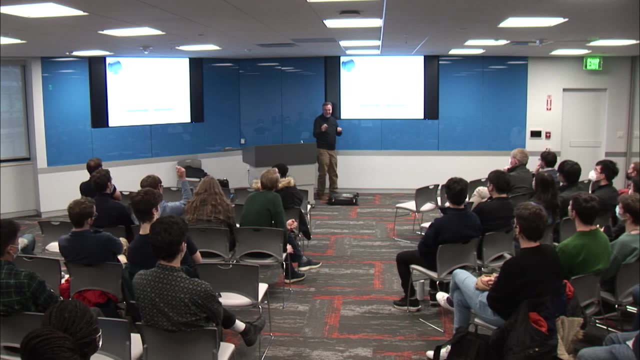 should watch Silicon Valley. This is like one of the best shows on television. It's a bit older now, but and I've lived part of that life, Not all of it. obviously, Yeah, Is it the same way? No, no, no. 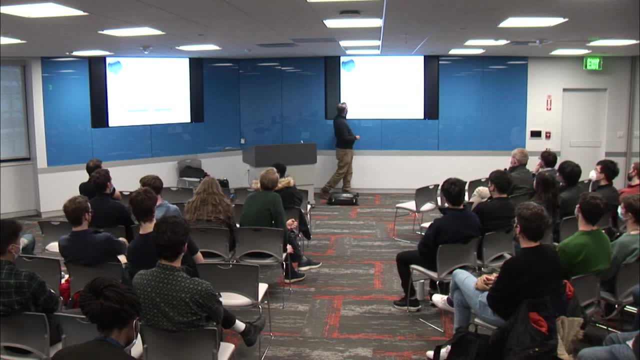 This is really very well known. So you do Dijkstra in one way. So this is forward search and backward search and you hope to meet in the middle, which is an old idea in classical search. So I'm just showing very vaguely that in factor graphs. 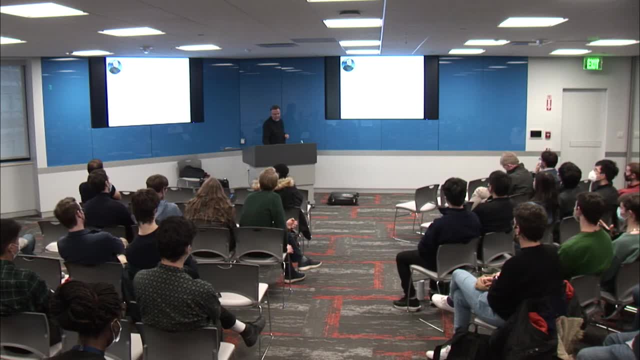 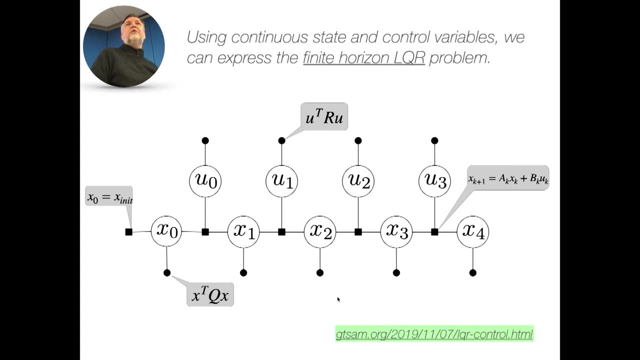 and bucket elimination. you can have all these same ideas, And then also you can do LQR. So just again, a show of hands. who knows what LQR is in this audience? OK, Wow, OK, So I'm at MIT. 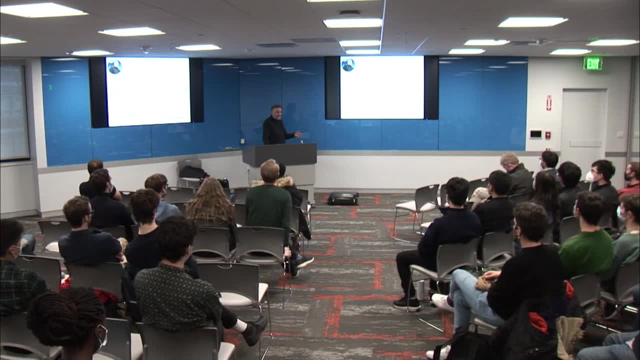 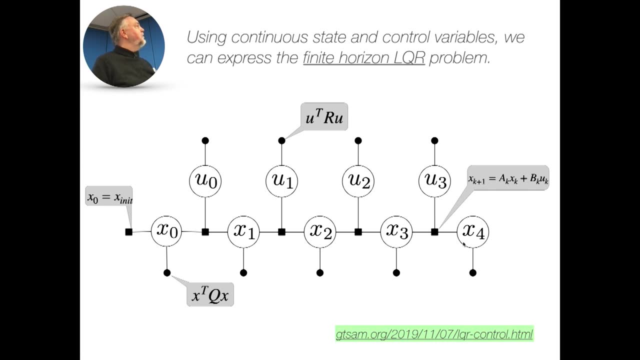 So maybe this is like in one of your first classes or something you'll get. So LQR can also be written as a factor graph. So here we have a trajectory over time and we have a control sequence And we don't want to give too much control. 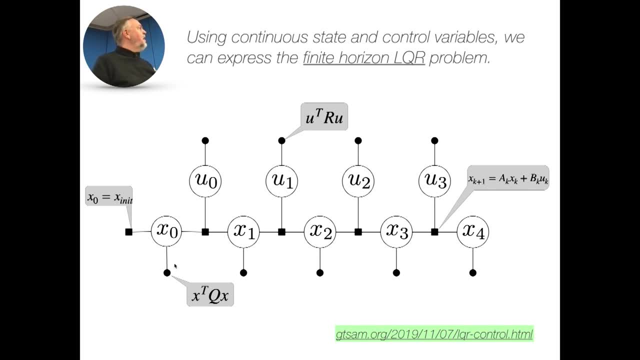 so we put a quadratic on the control, which is a cost, And maybe you have some desirability on some state. Maybe in pure LQR, we will punish everything that's not 0. So we want to get to a state that is 0, right. 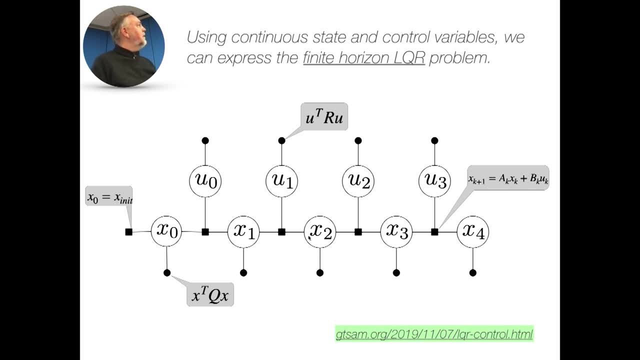 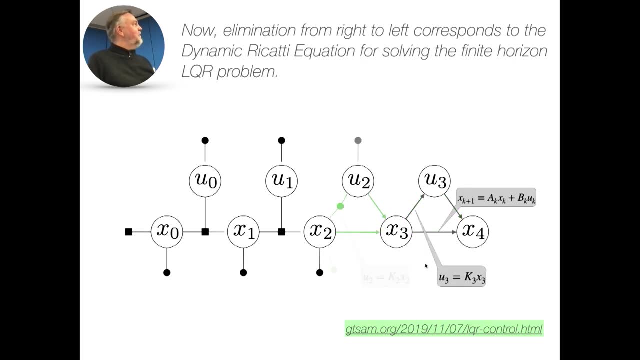 And so you have an initial state. And then it turns out, when you do bucket elimination on this, this eliminative graph, what you get is a policy. You get a finite horizon LQR policy with time-varying matrices here that give you a time-varying LQR. 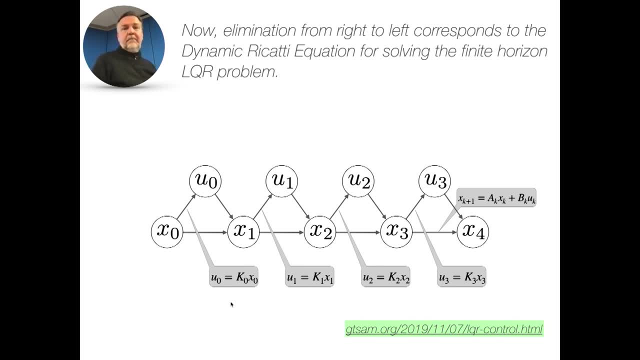 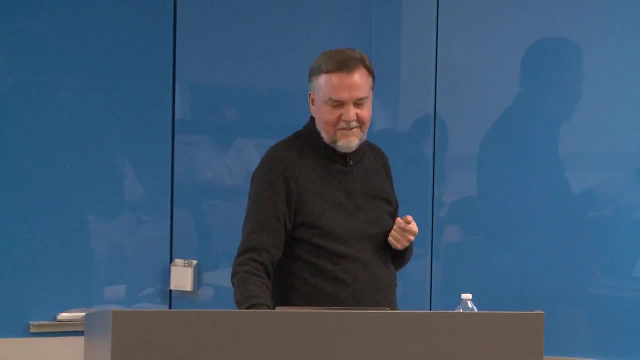 finite horizon control. OK, So you can do this with any other algorithm. You can do this with any other algorithm. So almost exactly the same algorithm as discrete search gives you LQR right. It's just in fact in GTSAM. not many people know that. 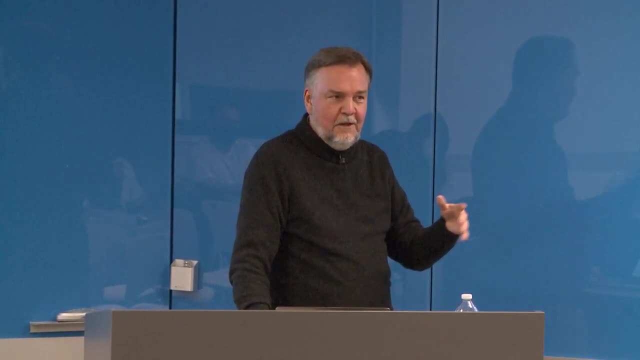 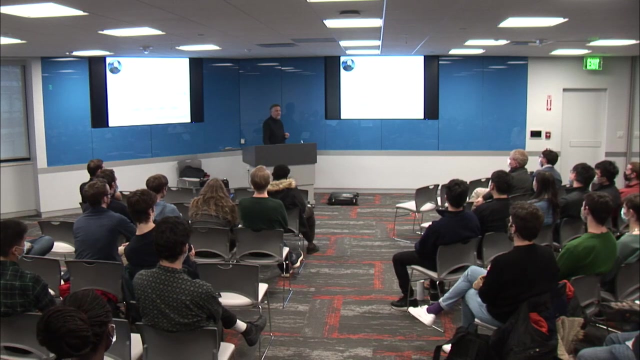 But you can do SLAM and tracking and all these things, But there is another branch and I think Kevin knows this. Where is Kevin? There is Kevin. Kevin is the only other person that works in that branch besides me. right, There is a whole branch in GTSAM that solves Sudokus. 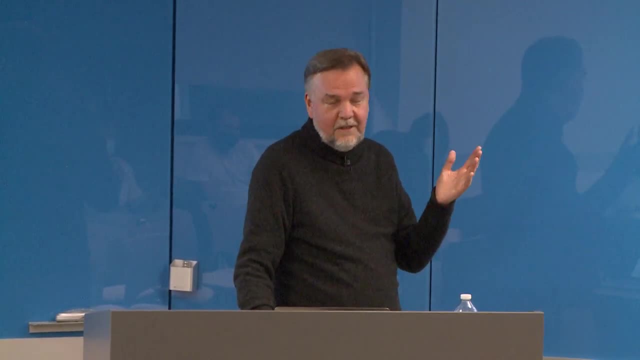 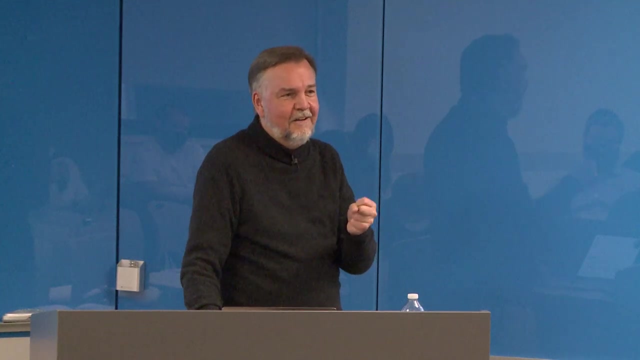 It's just bucket elimination and just constraint satisfaction and Boolean satisfiability, And what I want to do with Kevin is build a branch in the middle that does hybrids. Any hybrid problem that you solve, at least will try to do something, And then we can give that to Leslie and Tomas. 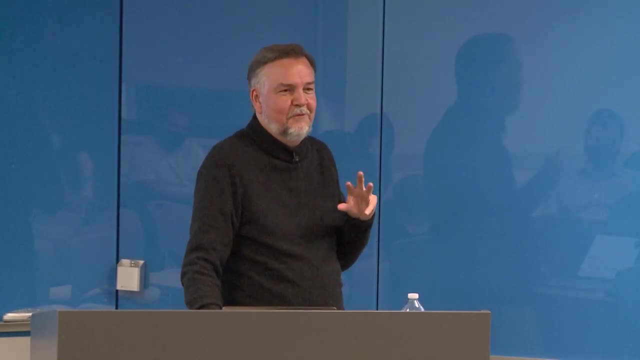 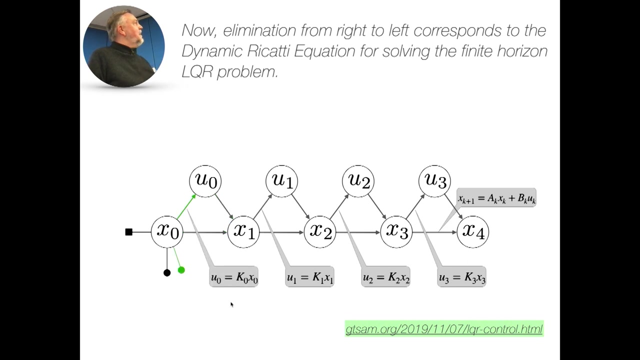 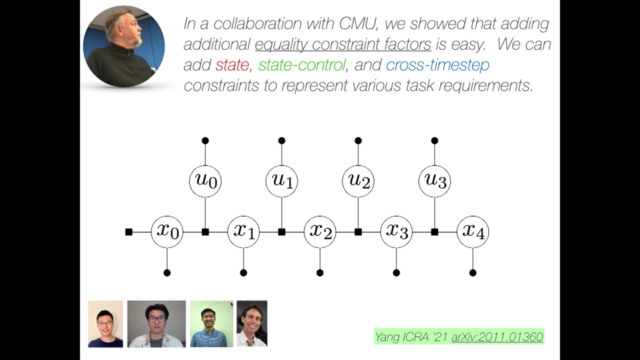 as a general hybrid solver, which will be very expensive, But yeah, but beautiful in principle. No pressure, Kevin, So you can. of course, this is LQR And it's not super interesting. It's interesting that you can see it as a factor graph. 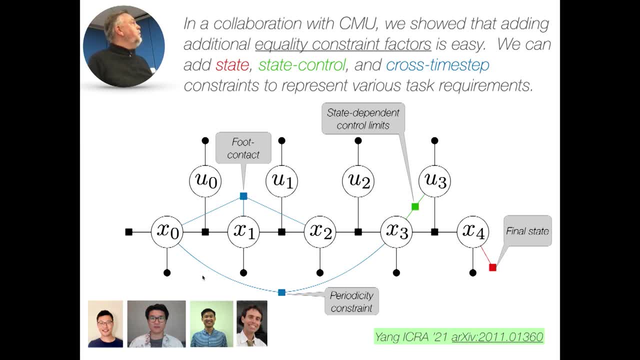 solution. But then we can do things like: oh well, these constraints, these costs are all unary. Could we just have constraints that tie things together over time, Russ? Which means now they're no longer local constraints, So you can add constraints, sort of arbitrarily, over time. 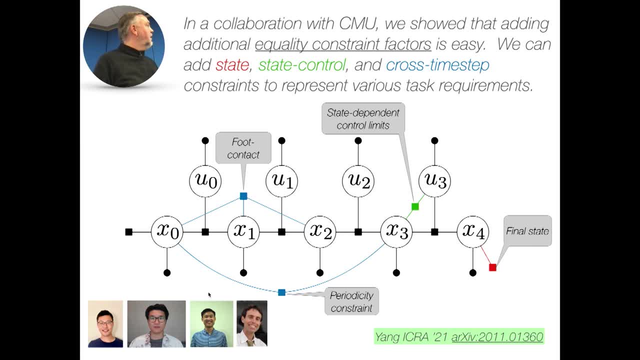 like periodicity or state-dependent control limits or something like that. So this is work we did with Howie Choset and one of his students And this is in ICRA. This is sort of equality of constraints, LQR, with arbitrary equality of constraints between timestamps. 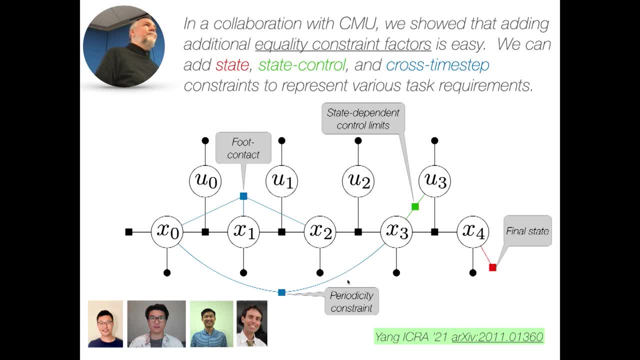 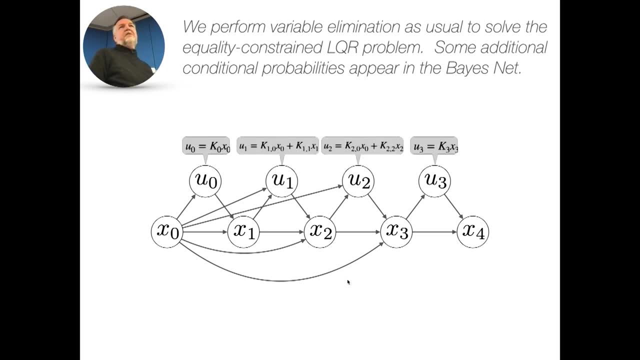 And it's really just build a factor graph, solve it. It's done. How about inequality constraints? You can also do inequality constraints, Although in GD-SAM we're not there yet. We're building in another repo. it's called GT Dynamics. 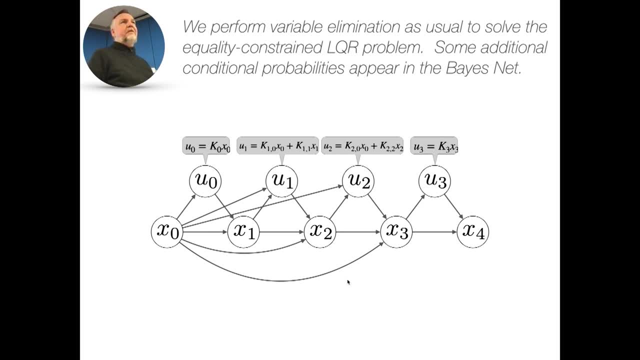 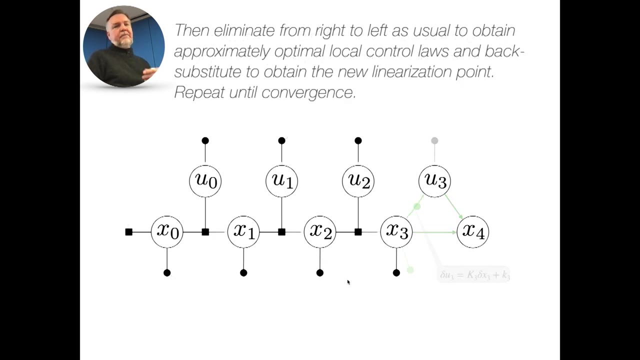 We're building an augmented Lagrangian sort of real constraints. Typically we do inequality constraints with soft versions of it, But now we're getting more serious about it And then finally you can do this. You can do this iteratively. 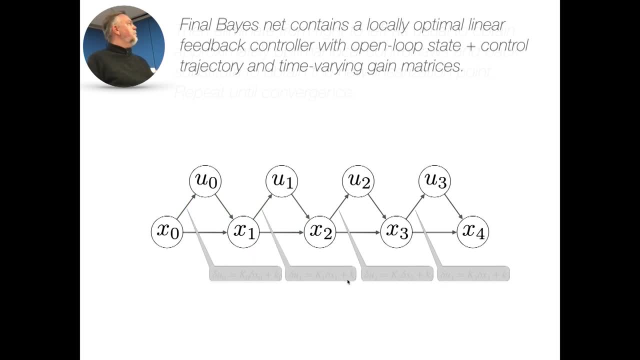 So this is an algorithm by Todorov, ILQR, which is iterative LQR. So now we can optimize for a trajectory non-linearly, then build a time-varying LQR controller around it and then use that on a robot. 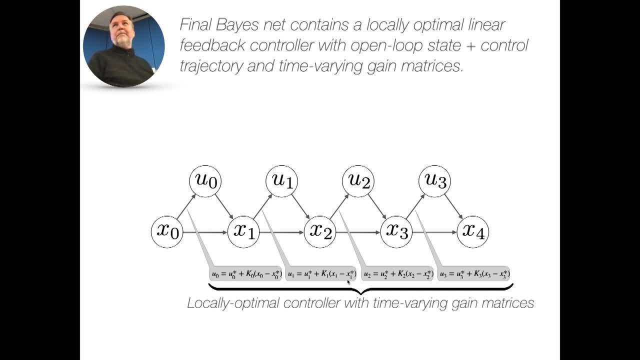 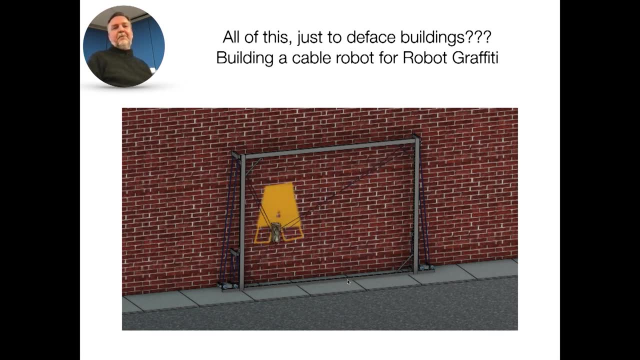 And in fact that's the second art project that I want to share with you, which is so with my student, Jerry, we want to tackle graffiti with robots, So just to deface buildings. it turns out graffiti is a really cool art and very prominent in Atlanta. 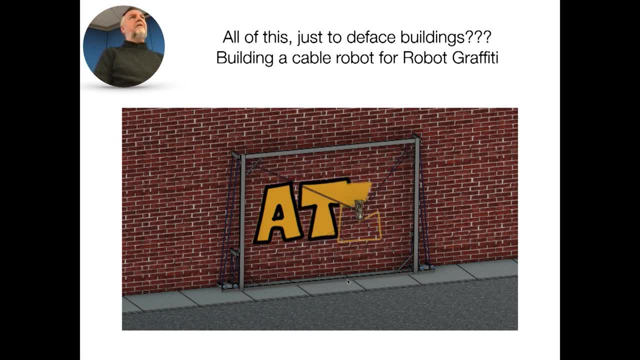 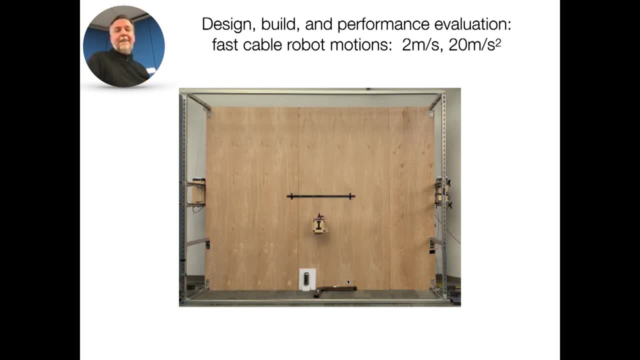 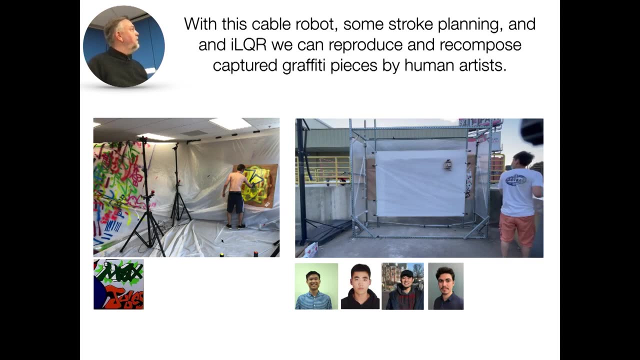 And velocities to do graffiti. well, OK, And then we did mocap so we can actually do create new works. So we did mocap here. This is actually my nephew who visited me and he's a graffiti artist And mostly he defaces trains and buildings. 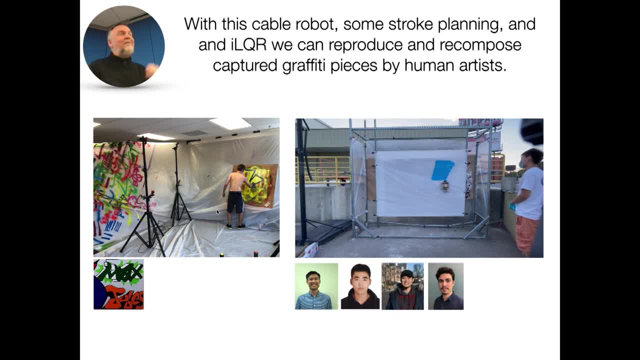 but now I had him do mocap. He was very impressed and he did Python scripts et cetera And he just graduated high school. really It was really cool to work with him And now we can take the letters that my nephew did. 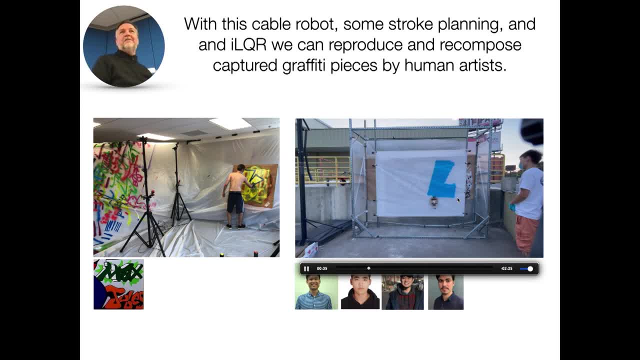 then put them together in different combinations and have the cable robots execute on the graffiti. Now how do we do that? Well, we have our desired trajectories. We solve a nonlinear optimization problem using GTSAM to get a trajectory. Then it turns out after you have the solution. 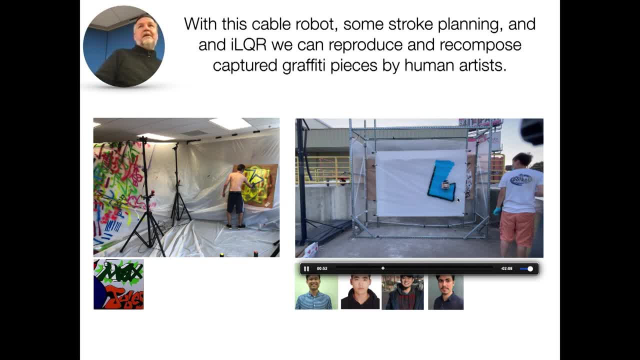 you already have the LQR time variance. You have the time-varying controller right there in the base net, OK, And then you send that time-varying LQR controller to the cable robot And then now you have a controlled graffiti system. 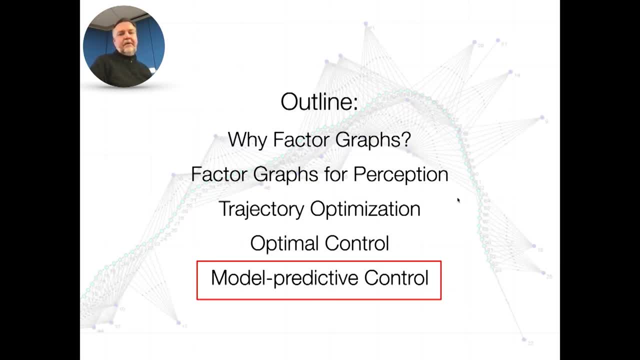 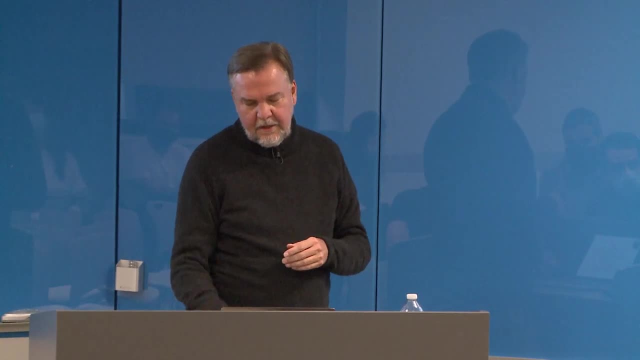 Cool, And then finally, I guess I'll stop. So there is a whole line of work where we try to do estimation and control at the same time, which is steep. But I'll just skip that part because I'm at the end of my time. 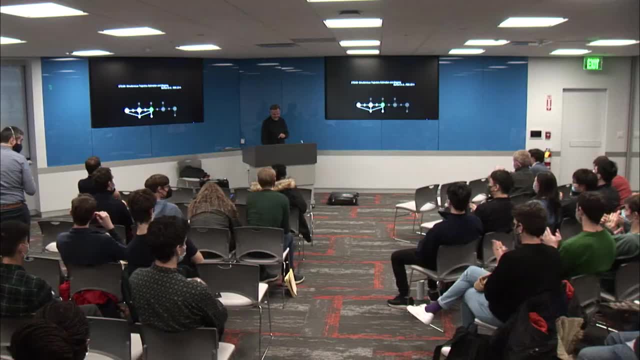 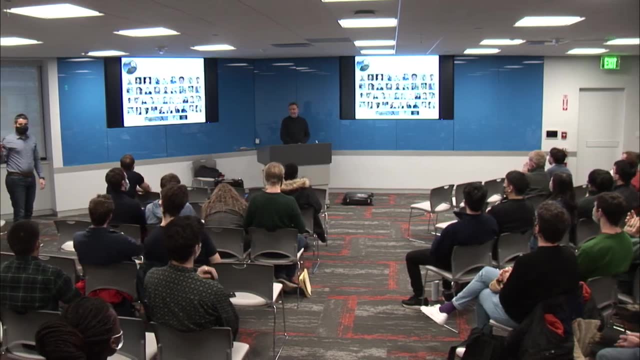 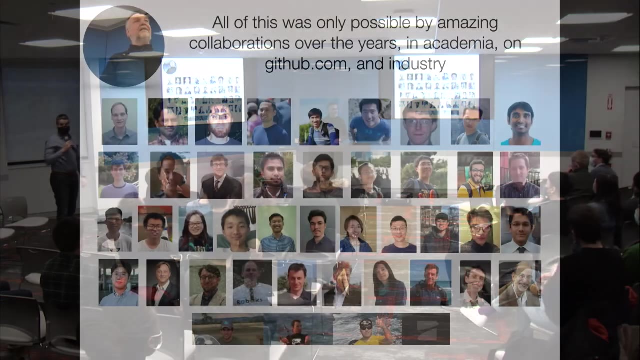 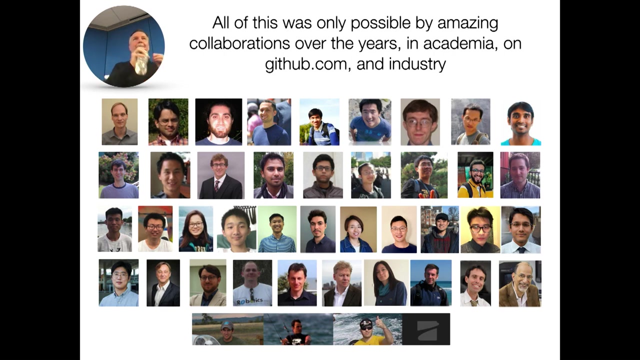 So, all right, That's it, And this is lots of people that worked on this, So here they all are. I mentioned some of them by name. Who wants to go with the first question? All right, The person in the Christmas sweater. 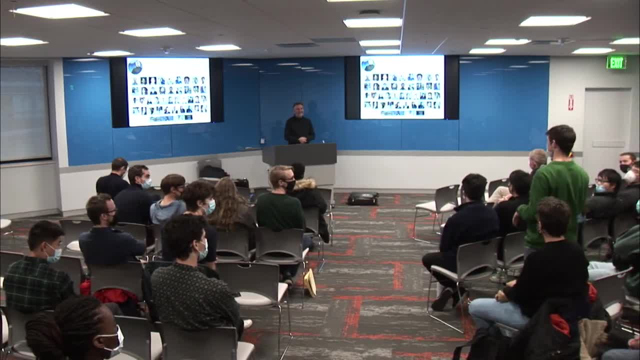 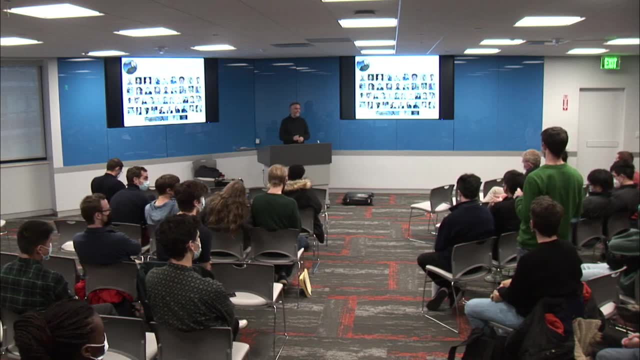 Thank you so much for coming to talk with us. I guess I'll stand So at the end of the day, all of these problems are non-convex, at least. maybe not all, but a lot of them Which, like in SLAM, we find a lot of the times. 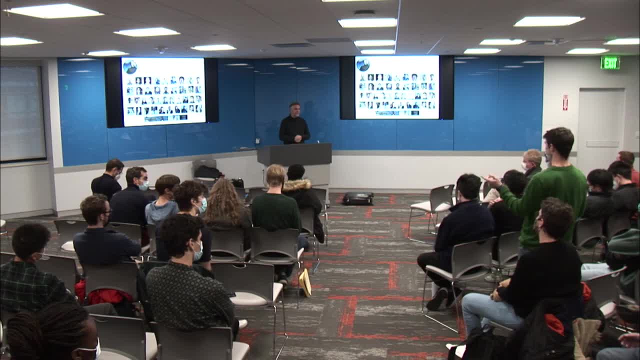 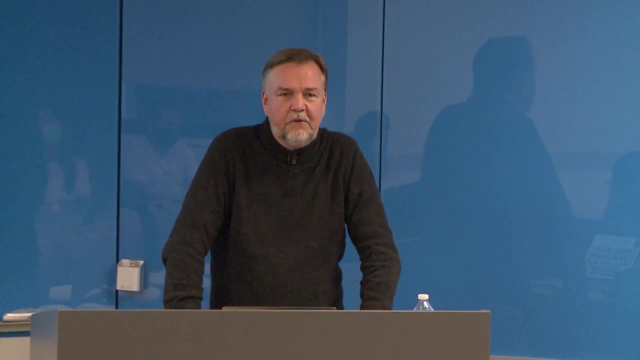 the initialization strategy really matters for all of these new action-type problems that you're solving. Do you find that you have to be somewhat artful with the initialization strategies Or in general it just works out? It really depends on the problem. So even some action problems are easy. 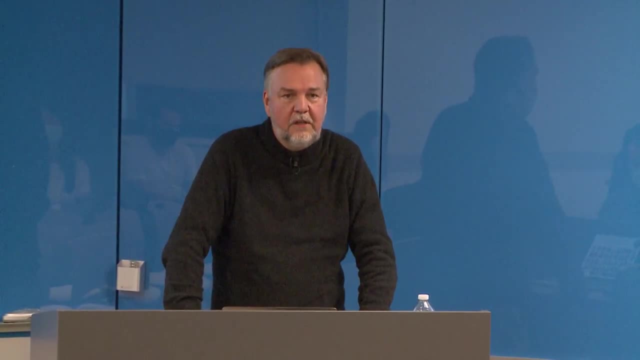 I mean LQR, for example, is convex right, It's just solving one linear system. But yeah, no, I think that's the big problem. And especially well, a lot of you are interested in mixing discrete and continuous things. 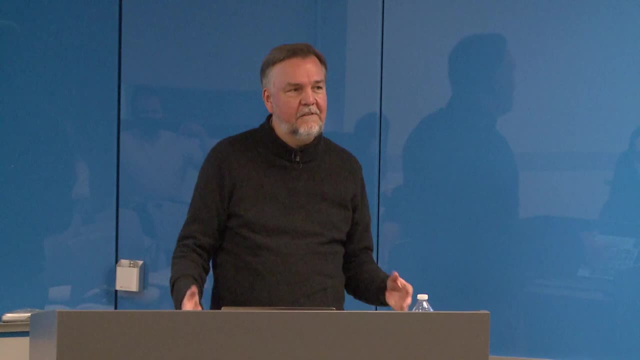 And then that's the whole TAMP problem, right, And I'm super interested in TAMP and what you guys have done here for TAMP in at least two different groups, where you're mixing task-level things and then continuous motion planning things. 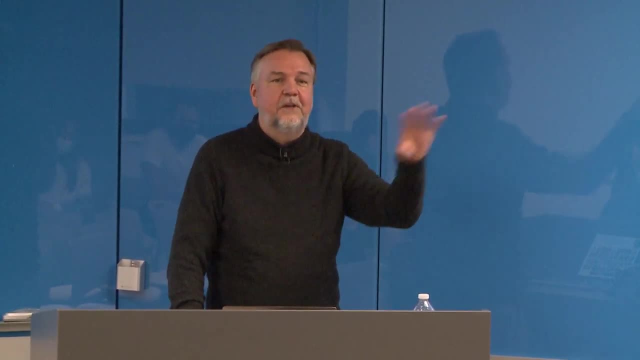 And those are very non-convex, very non-linear, exponentially complex. So initialization, in a way, is the whole game there. It's like you search your way with heuristics and try to find a spot, And it's a spot where you will not. 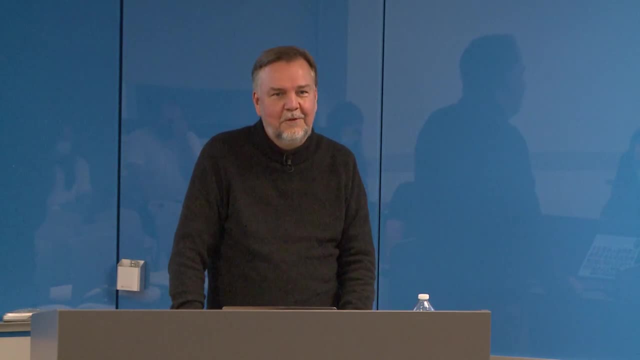 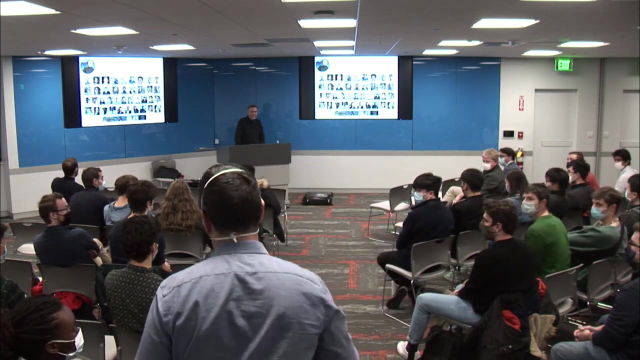 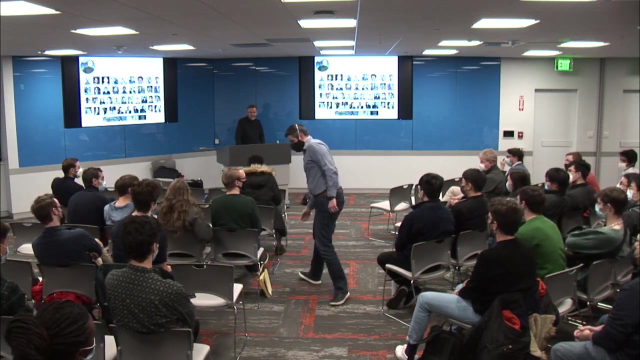 be deep in the mud in some local minimum. So, yeah, I guess I think initialization is the whole game And you have to be artful. absolutely Want to go next. There's a question here? Yeah, this is a really very interesting talk. 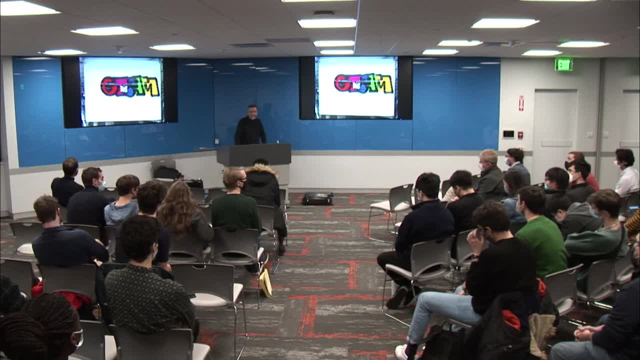 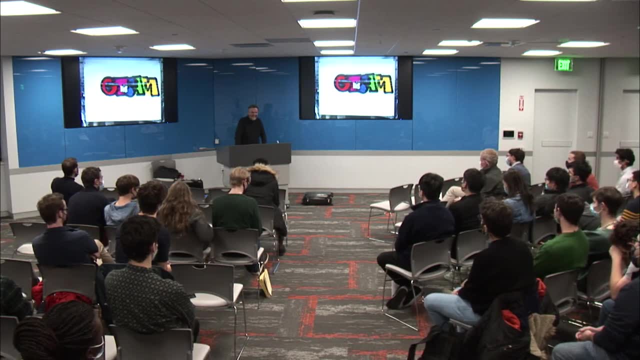 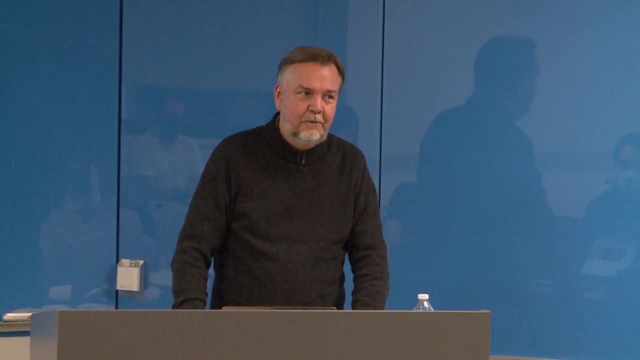 Thank you so much. I have one general question: What would you say is the weakness of GT-SAM? What would you change about it if you go back? Well, the weakness is it can do Sudokus Well with appropriate constraint satisfaction. 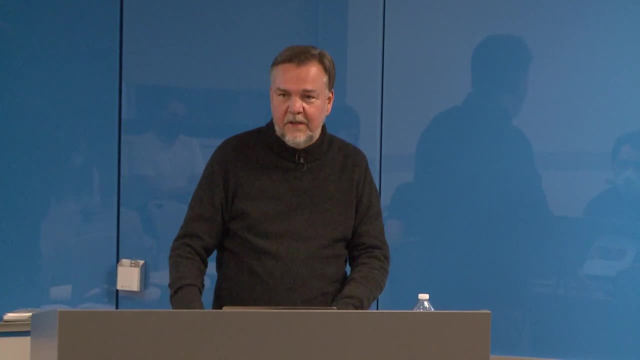 propagation. it can do Sudokus. You give it a 9 by 9 Sudoku and it never terminates. so with bucket elimination. And it can do optimization really well if you give it a good initialization For nonlinear problems. But it cannot do the mixture of both. 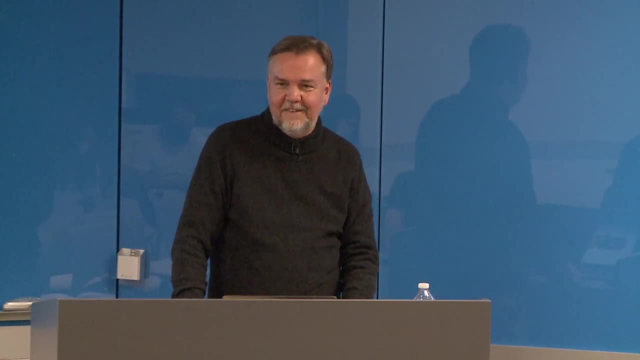 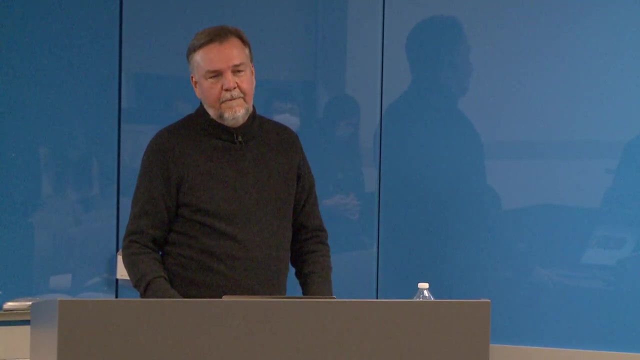 So I think that's the final frontier, if you want, is if you can just do an arbitrary factor graph and you have an algorithm that can solve it. And that is really the TAM problem, if you think about it, But also many other interesting problems. 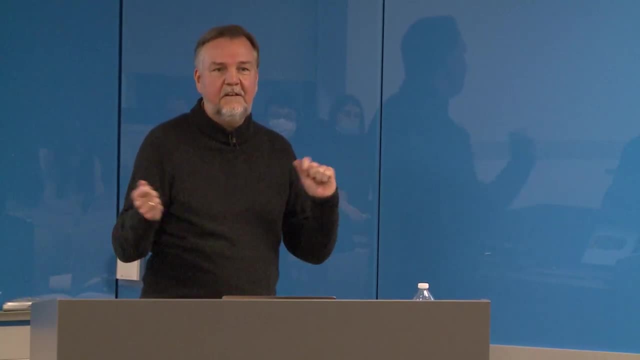 like data association and semantic slam and anything that has sort of value judgments or discrete variables in it. So it would be great, It would be great to be able to have solutions that push in that direction, And many of them are being developed here. 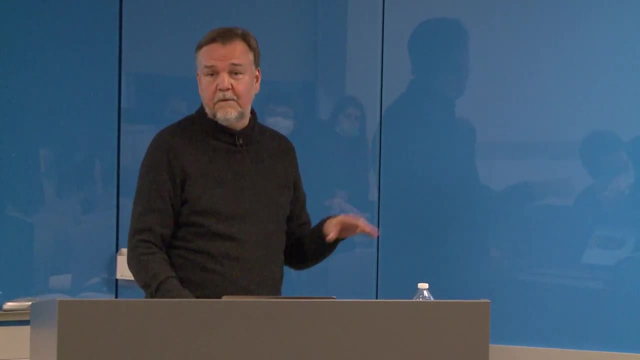 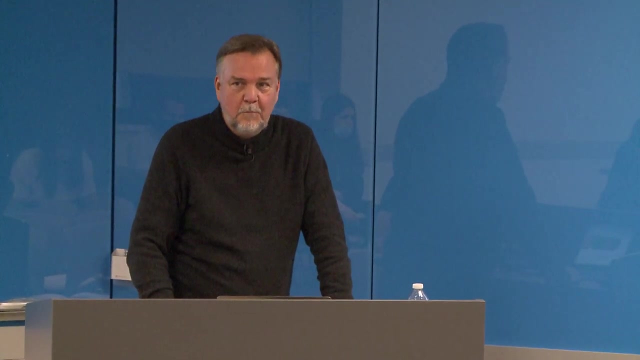 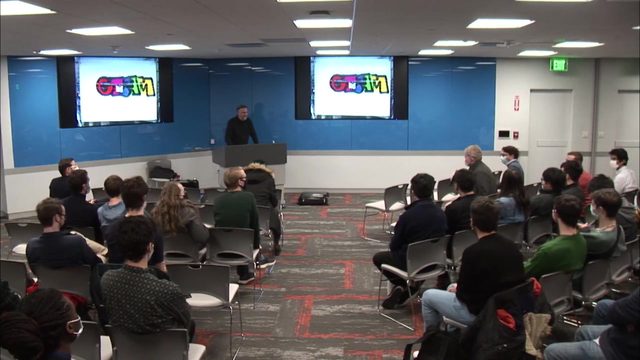 and in Michael Case's group at CMU. He has some really cool ideas there. So Kevin has a really cool. So I think that's the weakness and that's the opportunity. Thank you, Fantastic, Frank, Really awesome. How about the class of problems that involve humans? 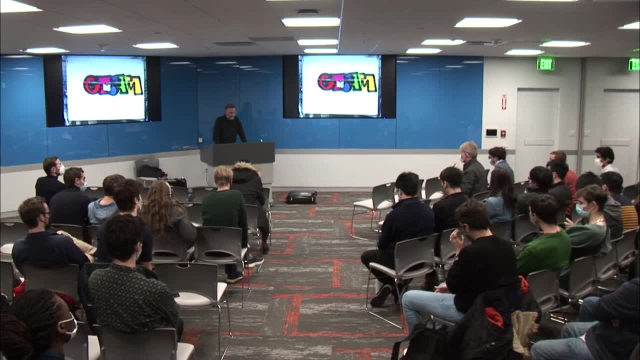 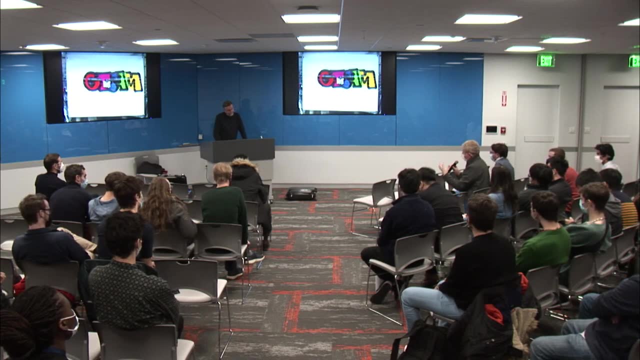 So sort of, I would say, human-centered robotics or robots interacting with humans and, for example, helping elderly people in their houses or helping drivers to drive more safely. Can you imagine how the factor graph methodology might embrace understanding and predicting human behavior? 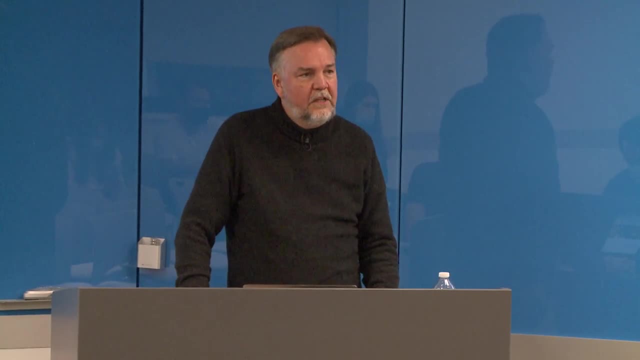 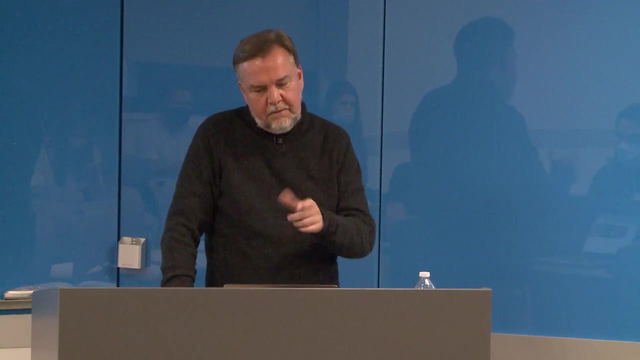 I'm not an expert in that, So I don't know, I don't know, I don't know. I don't have any experience with that, except that we were tracking people with the Skydio drone. There is two things that I hinted at. 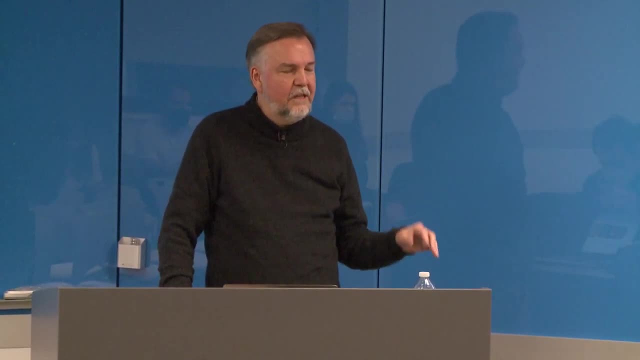 which is that you can do inference on intent. And this is a very old idea In Air Force. people have been doing sort of maneuver detection since forever, And so that's a human pilot that they're trying to do inference on. So that's one way. 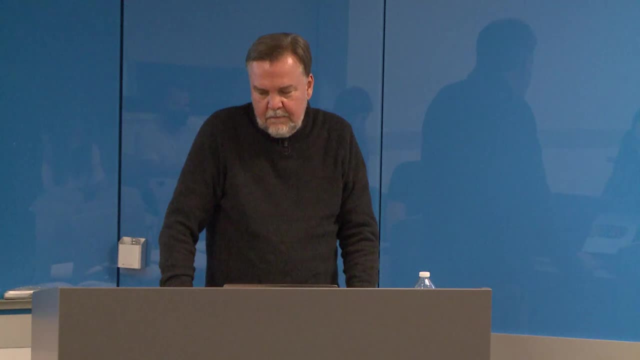 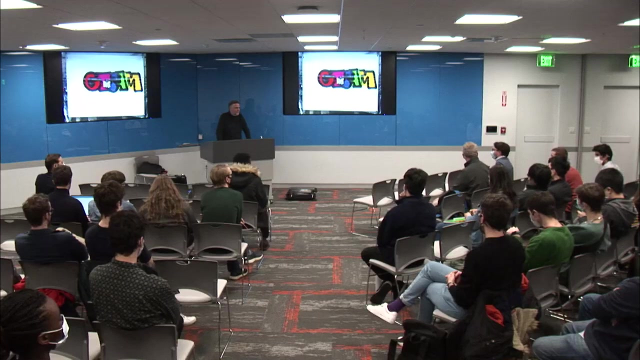 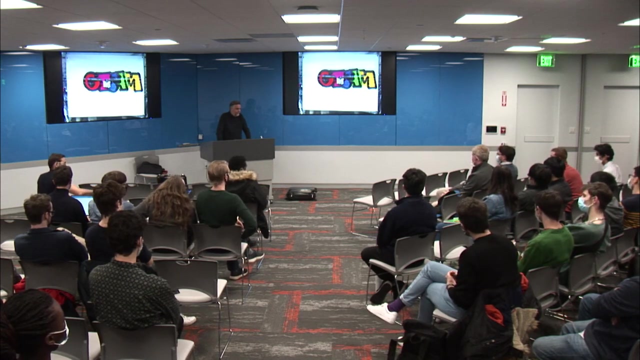 But I don't have deep ideas about that. Yeah Thanks, Frank, Great presentation. So a question about how to use GTSAM. Let's say I'm doing deep learning, I'm not doing traditional geometric estimation. Is there an easy way in which I can take advantage? 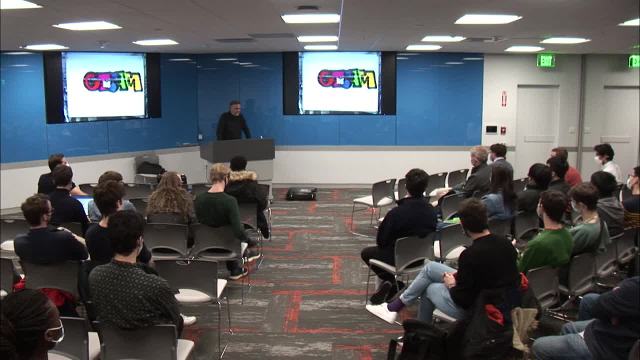 of the library for deep learning. And the second question, which is somehow related, most of it is CPU-based right now. Can we take advantage of GPU to speed up some of this? I think the answer. I can give the same answer to both questions, so that's good. 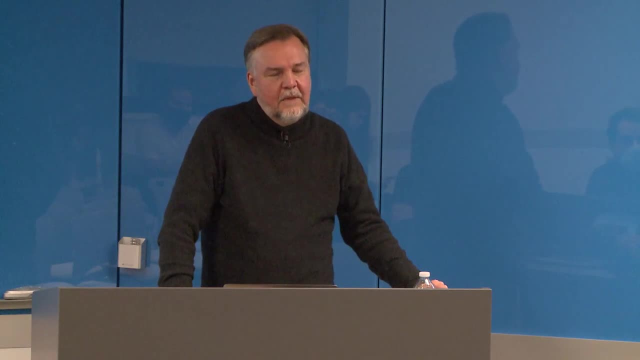 Yeah. so when I first joined Google, I worked with the Swift for TensorFlow team And I already hinted that I like languages right. I worked in ML and I love Swift, And then Chris Lattner, who had invented Swift at Apple. 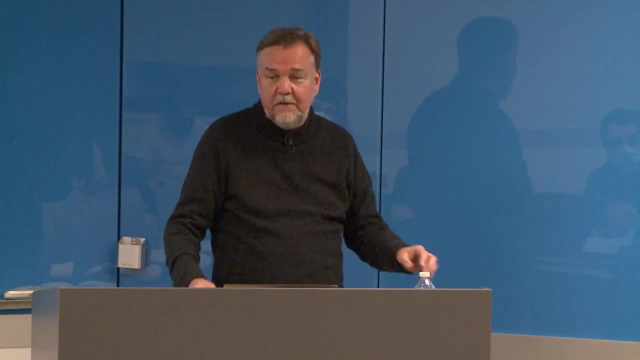 went to Google And he said, hey, I'm going to do some GTSAM And then started this whole Swift for TensorFlow initiative. So I was like this is great, We can do five graphs and deep learning in the same language. 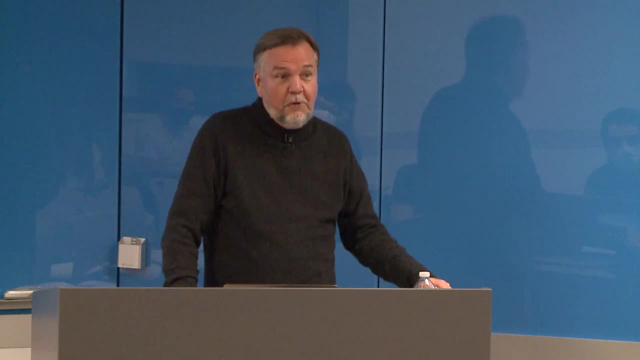 And now you get to play with Swift. Unfortunately, now Google, Chris Lattner left Google and then Google iced Swift for TensorFlow. So we did a project and we submitted a paper. So now we are trying to go back to Python. 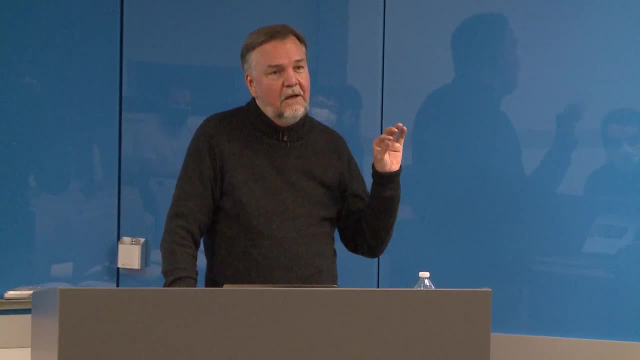 And a lot of deep learning is done in Python, And so we're trying to think about how we can expose. We already have an arbitrary factor that you can get. You have a function. You give a lambda function in Python and you create a factor. 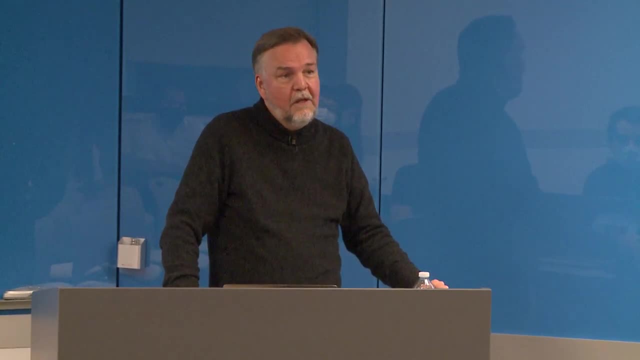 And GTSAM will do optimization for you with that factor So that lambda can be an entire PyTorch network, Right? But unfortunately, if you have a million of those factors it will call the GPU a million times separately, Whereas really what you should do. 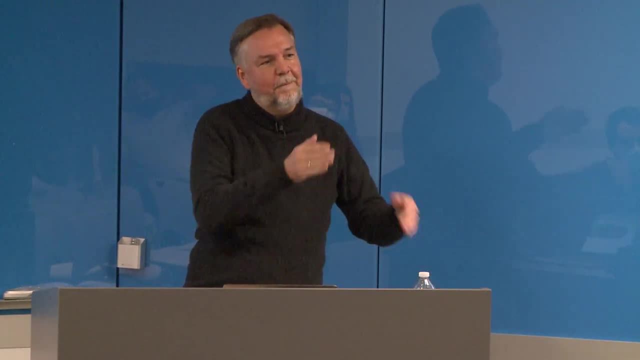 especially if you have a TPU or something you want to do, a batch with a tensor that's a million long and immediately send everything, Or batch it up in mini-batches of, say, 20.. On a GPU: 32.. 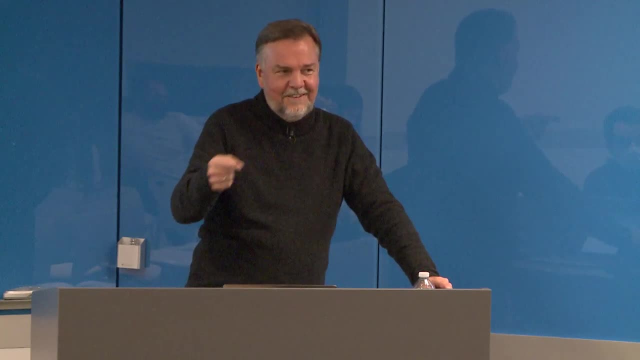 On a TPU 3,200.. OK, So of that. So we're thinking about how to enable that right now, so that you can use deep learning in a performant way. And, by the way, I should also mention and plug. 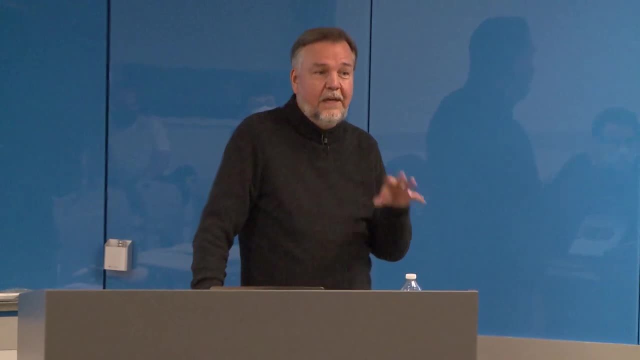 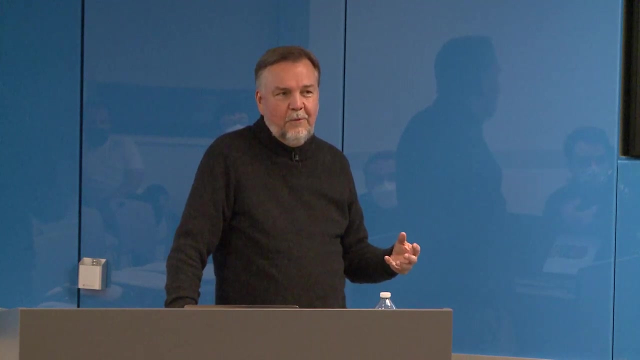 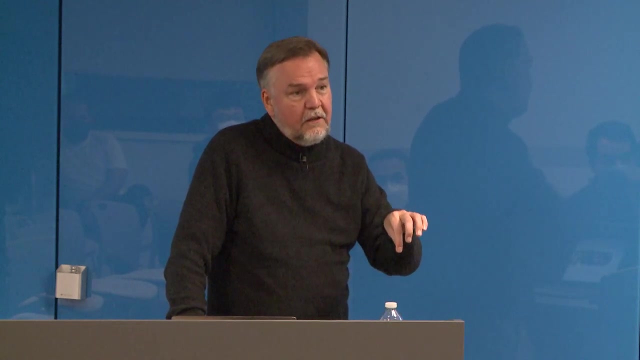 some work by a student from Michael's group. Paloma Sodi has written a really cool paper on it- It's called Leo- where she uses energy-based learning to do exactly that: Learn factors from lots of data that she then uses in a factor graph framework to optimize. 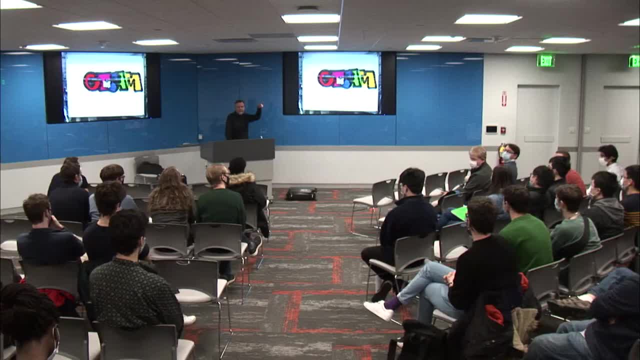 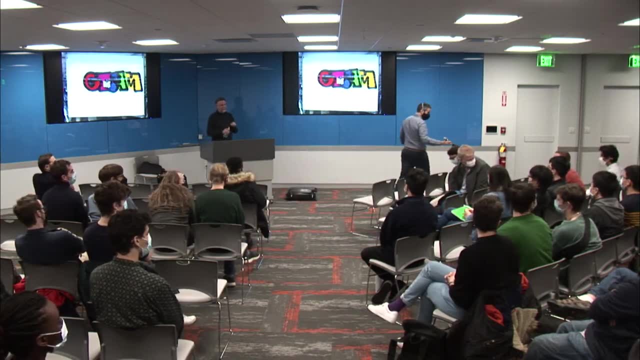 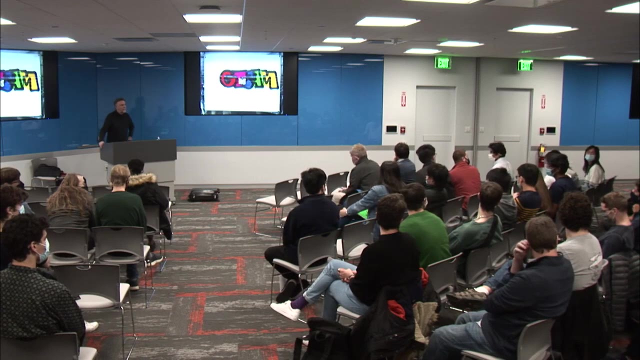 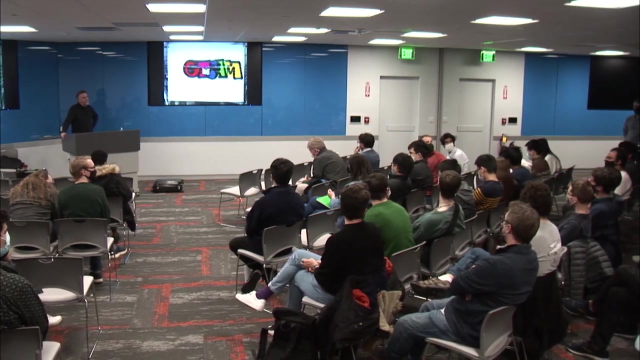 So there's a question in the back there. Thanks, Frank, I was curious. So, as we get to problems with much larger spatial and temporal scales and we want to use the factor graph to encode all the different observations we've made or the data we've collected, 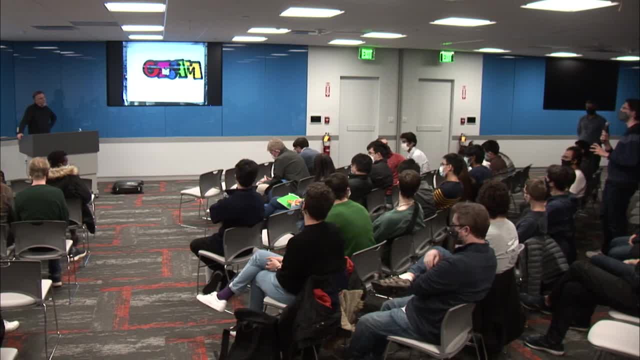 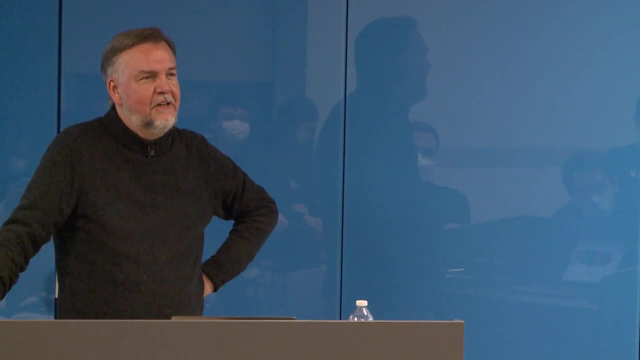 do you think there's a best tool or approach to take an arbitrary factor graph and capture the most important qualities and we get some kind of simpler representation, Or do you think that gets into a very application-specific or open question? No, I don't know of any solution there. 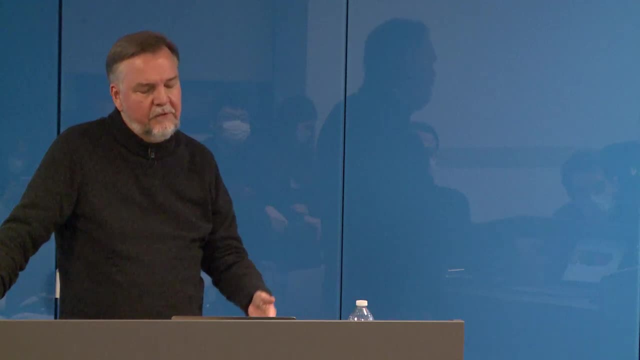 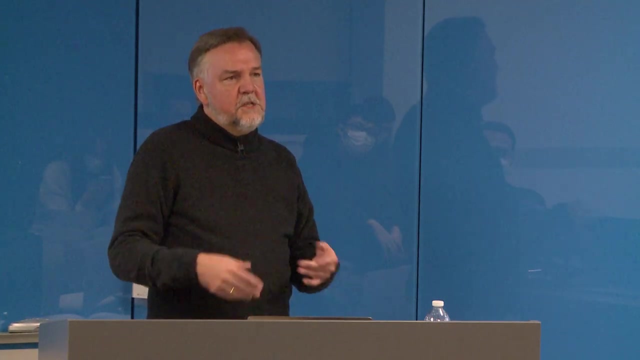 Yeah, In GDSM we have this graph. So, Nessa, dissection is a heuristic. that is very good. If you have a graph that is very large but you can split it in two and the split is not too large, then you can recursively split maybe. 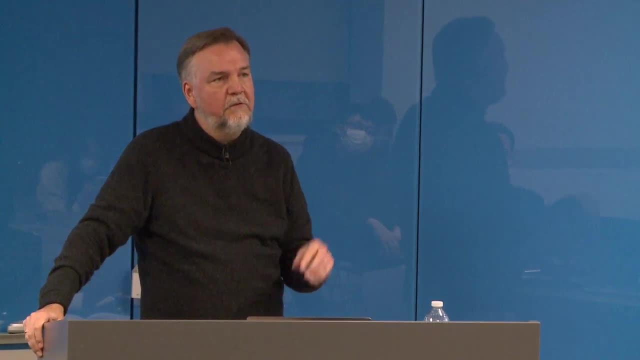 And that gives you a very good subdivision, divide and conquer of the problem. And we did it with a library called Metis, which is a graph partitioning library. So that's sort of the most general answer I can give you on how to break up problems into smaller ones. 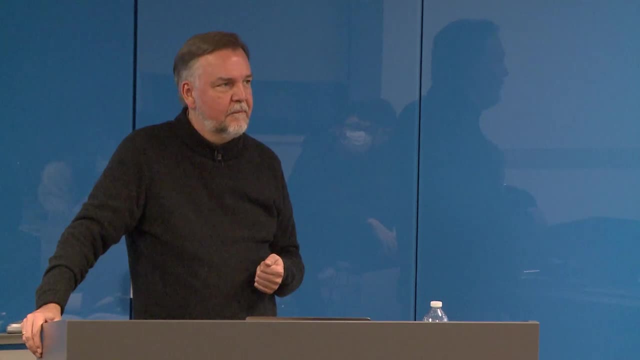 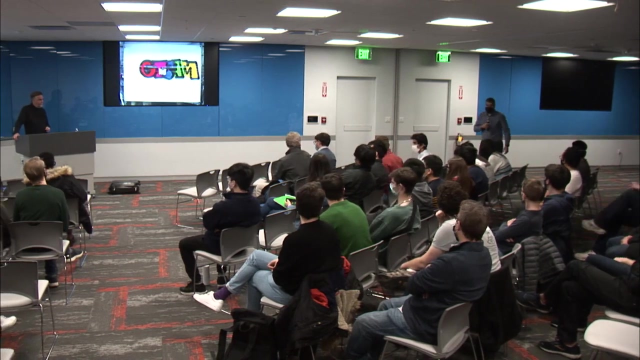 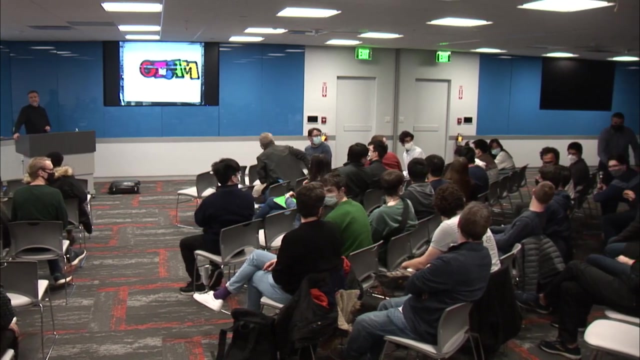 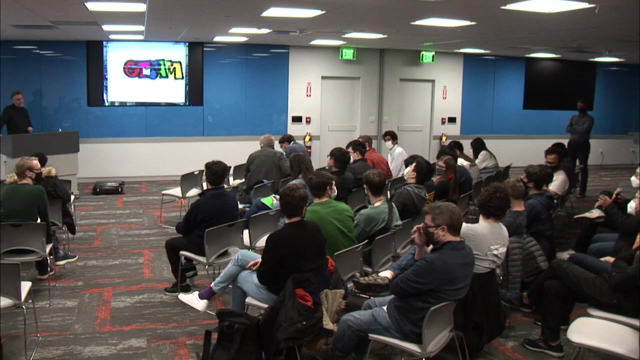 Yeah, Thank you. All right, I think that I don't know. if there are any more questions, OK, we'll take one more. Hi, thanks for the great talk. I was just wondering how actually the optimal control, or LQR, was implemented. 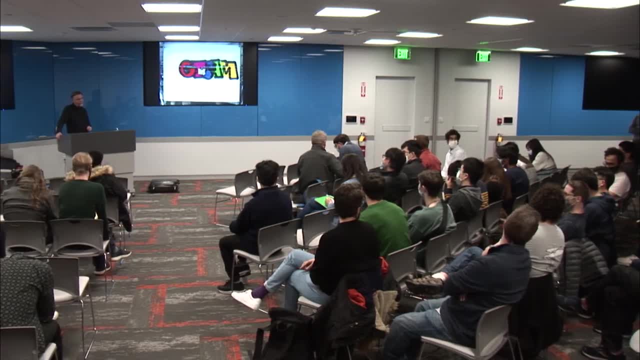 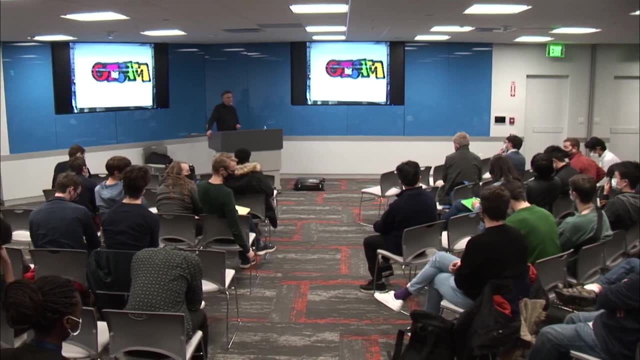 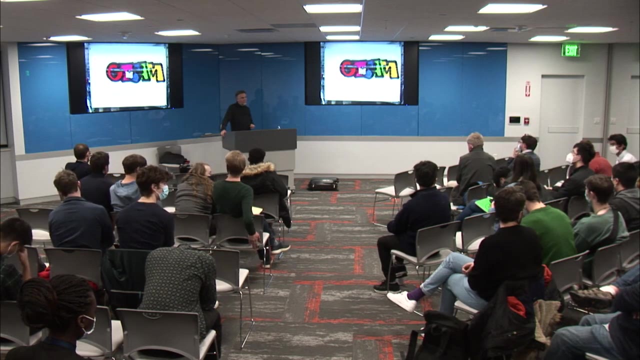 So in your slide I saw that you used some unary factors on the control actions and also the states, And I was just wondering: is it just simply putting some zero prior on each of the control actions, or is it something more complicated than that? 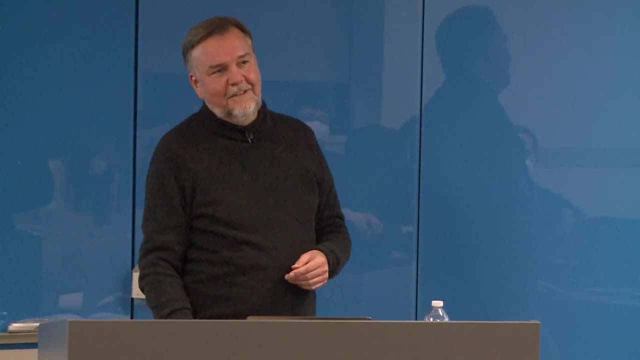 Well, yeah, it's not more complicated than that. In fact, LQR is all linear, So we don't even use the nonlinear factor graph machine. We use a GDSM- It's called the Gaussian factor graph- where everything is vectors and every factor is linear. 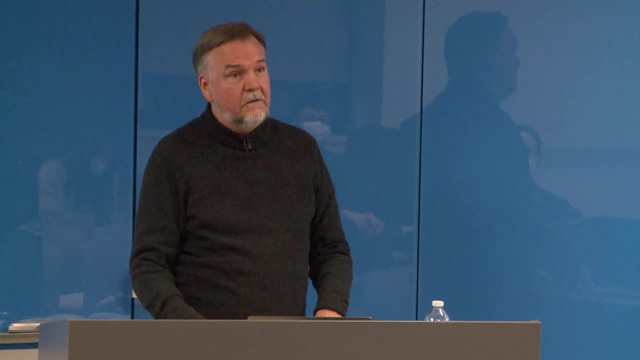 Yeah, So the GDSM is a Gaussian right or a quadratic, And the log of the Gaussian is a quadratic right. So yeah, just a prior on the zero mean prior on the controls and zero mean priors on the states. 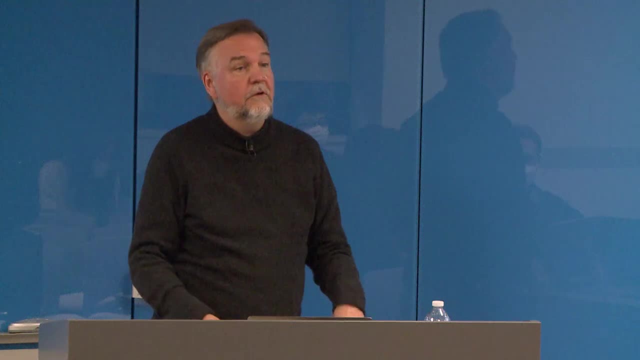 And the constraints are just soft factors, or hard factors if you use augmented Lagrangian, But then yeah, it's just linear. solve Gotcha, That's great Thanks, Yeah, In fact, in the linear case we can even do hard constraints. 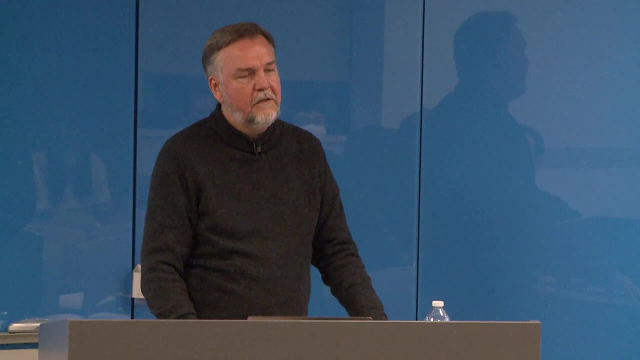 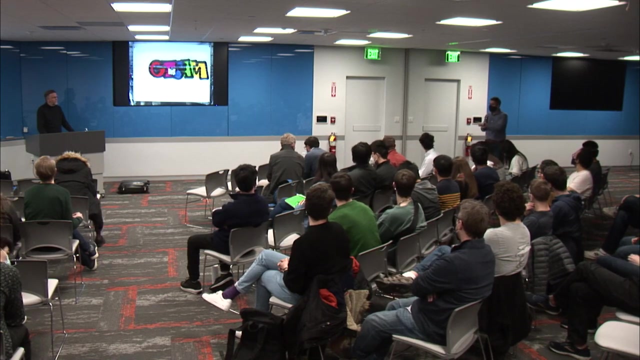 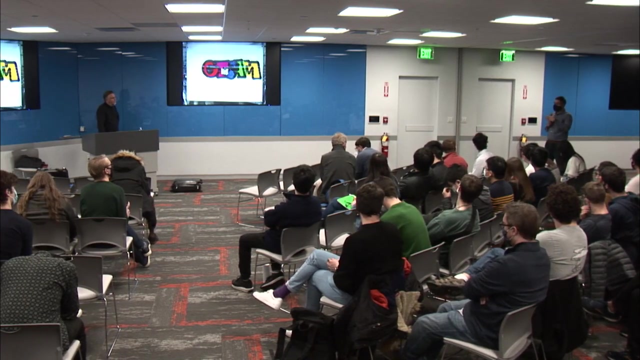 Our solver just solves them as part of the linear step, So linear constraints are easy. OK, I'll take the opportunity to ask you one more question. Have you done any case where you do both action and estimation- some form of active estimation problem? 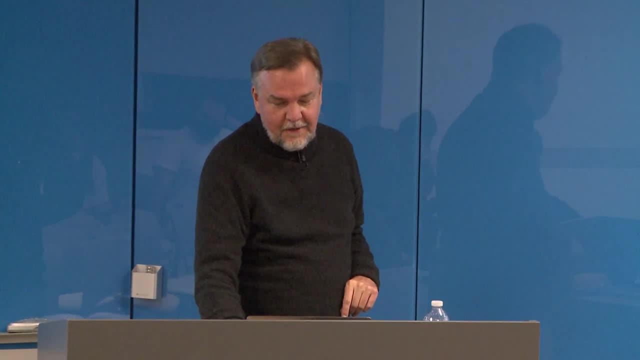 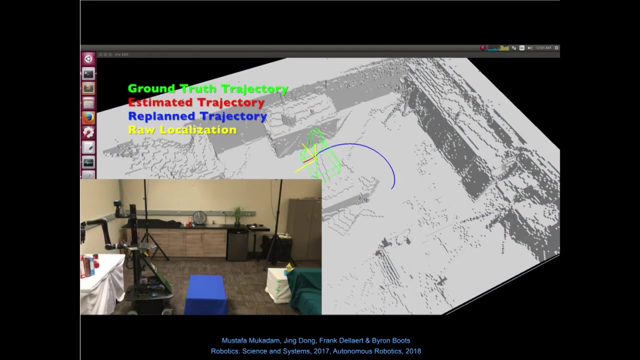 Yeah, So OK, show me, I'll show this video. This is from a paper called Steep, where we have a robot And we have a planned trajectory And then as we move, we see that noise on the carpet, et cetera. 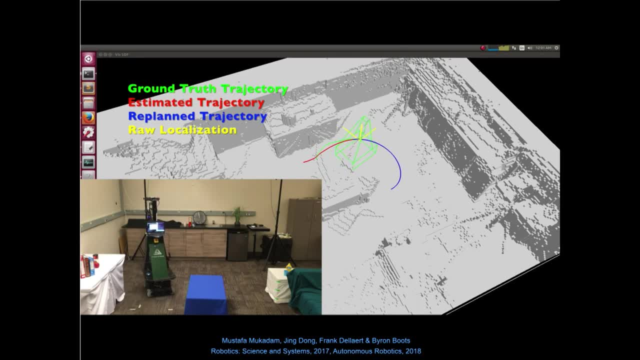 sort of deviate from our plan. So then we immediately replan And we put everything in one factor graph And then we do fast incremental replanning everything in one factor graph. Now it's a bit iffy to put both control objectives.